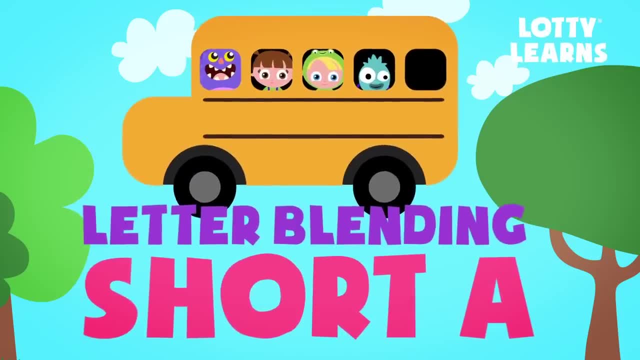 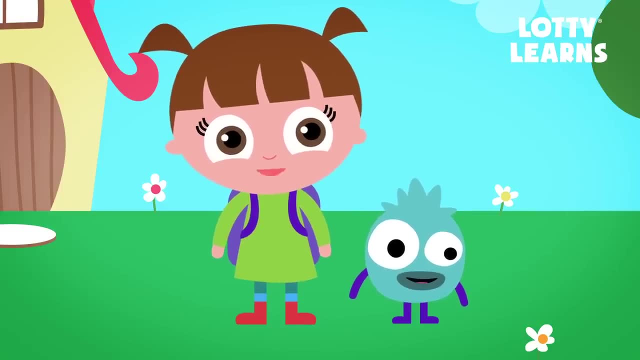 LottieLearnscom Letter- Blending with a Short A. Hi, I'm Lottie and this is Fuzz. We're on our way to school. Help us get there. by blending with the short A sound A: Just say the sound that each letter makes, then put the sounds together. 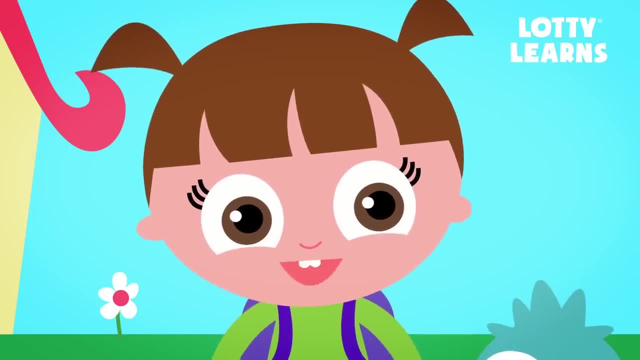 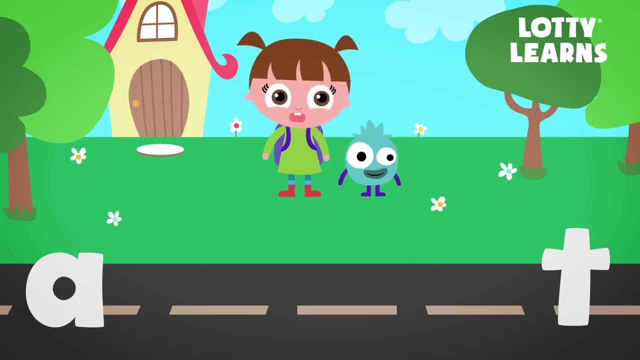 Try it with us. If you do a good job, you could win a gold star. We might even get to see Fuzz do something amazing. Here we go: The A says a and the T says t. a, t a, t at Awesome. 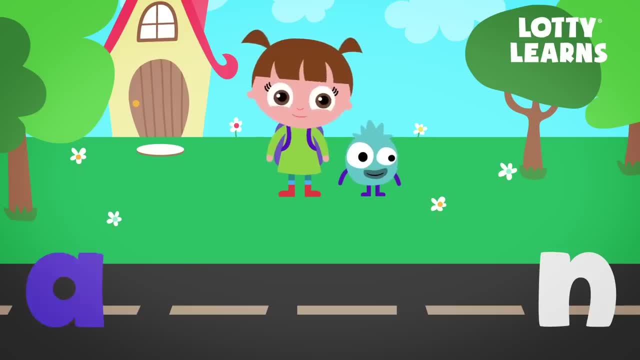 Let's do another. The A says a and the N says n, a, n, a, n, and Great job, Keep it up. The A says a and the D says d, a, d, a, d, ad You're doing so well, I think you might get a prize. 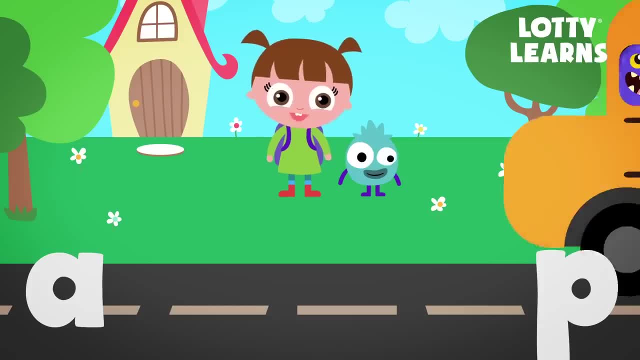 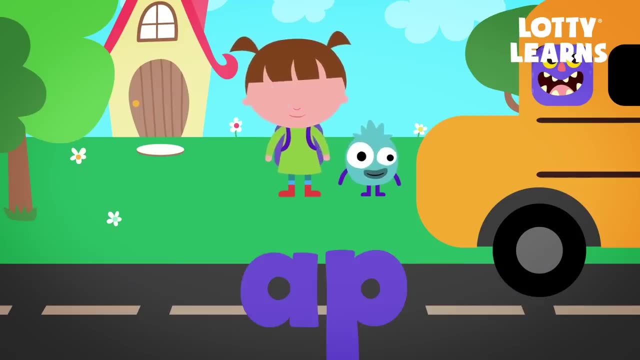 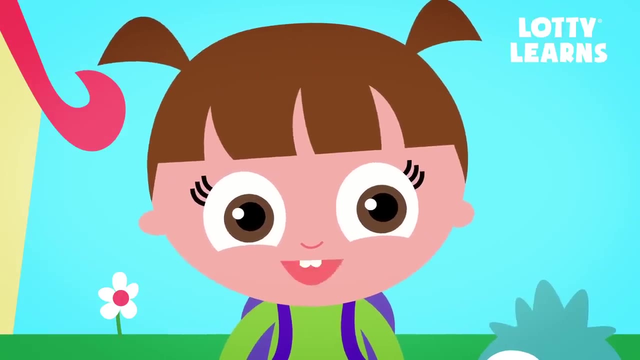 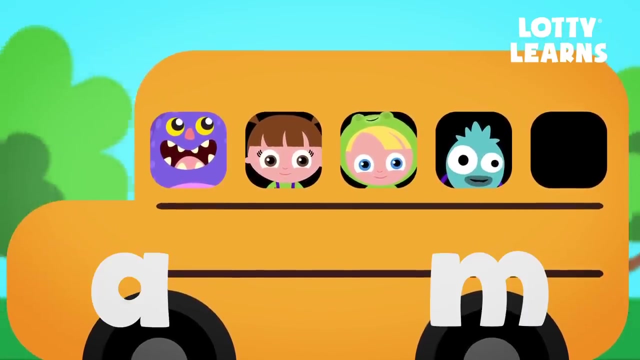 The A says a and the P says p, a, p, a, p, ap, Gold star. You just won a gold star, Keep it up. The A says a and the M says m, a, m, a, m and. 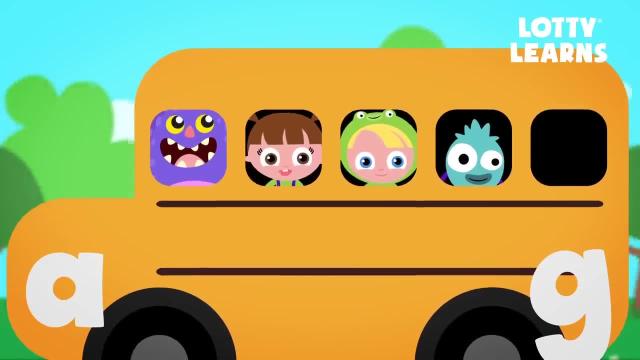 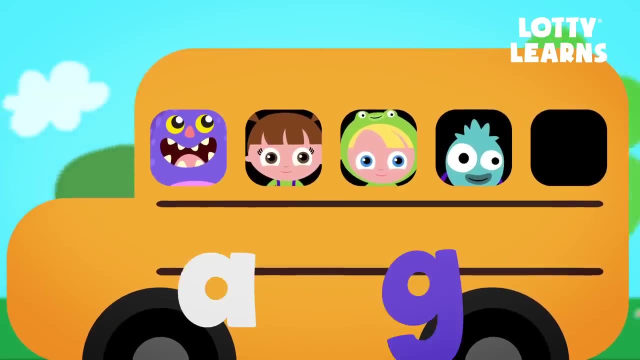 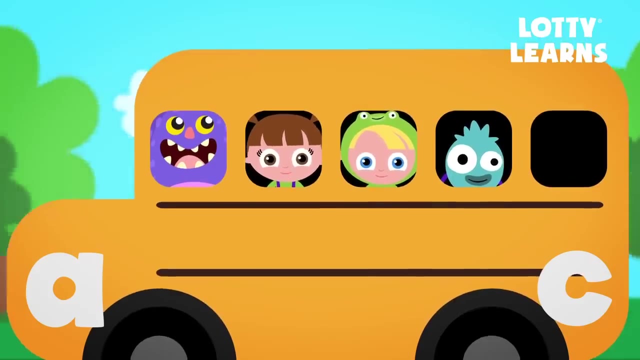 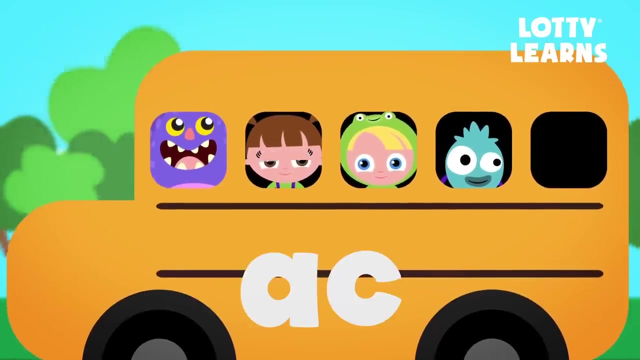 Super smart. The A says a and the G says g, a, g, a, g, ag. Almost done, Nice job. The A says a and t says c, a, c, a, c, ag. One more and we're all done. 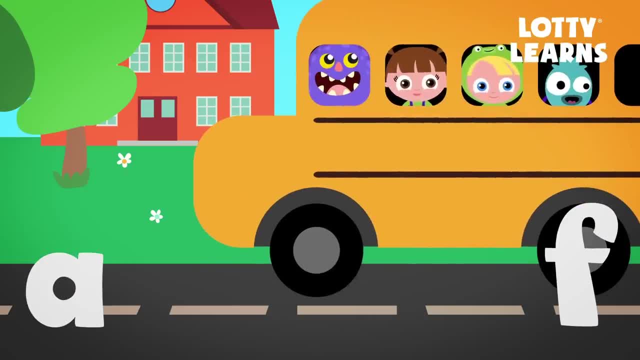 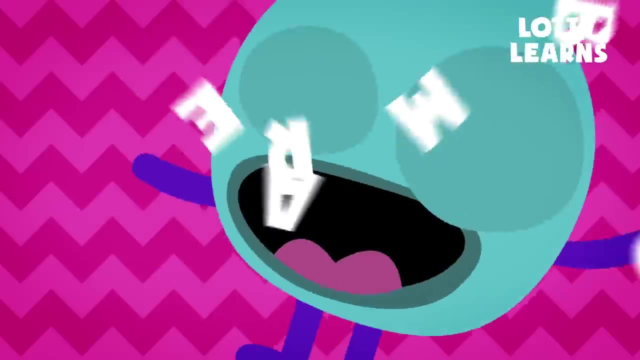 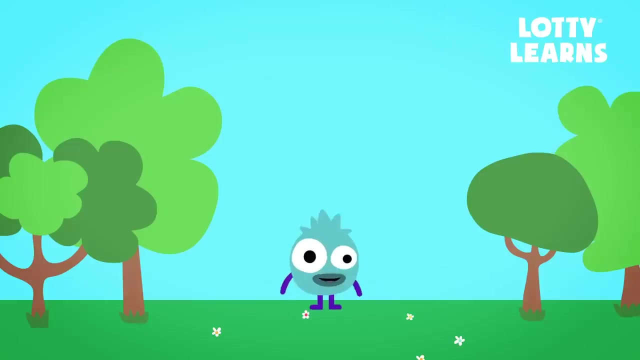 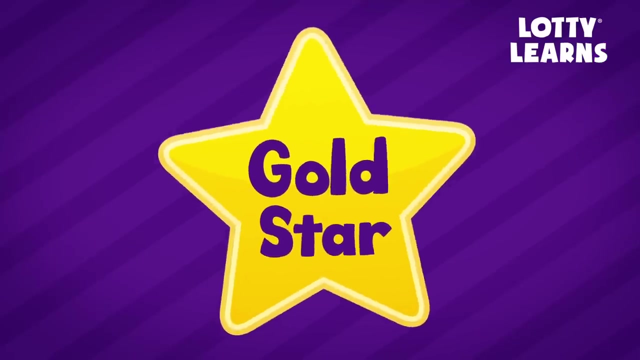 The A says a and the F says f, a, f, a, f, af. You did great, Great, But Fuzz looks hungry. I think he might grow Whoa Gold star. Thanks for helping us get to school. 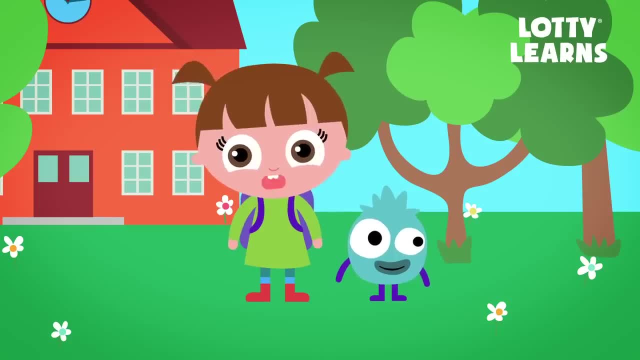 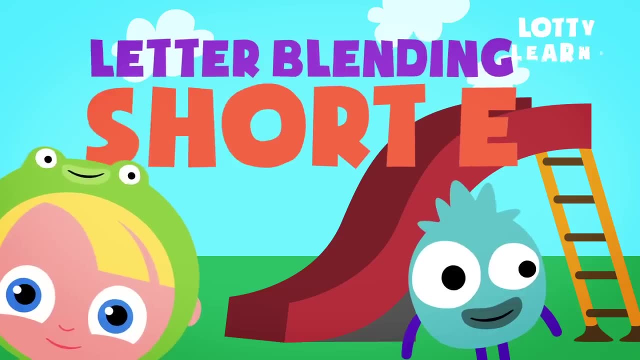 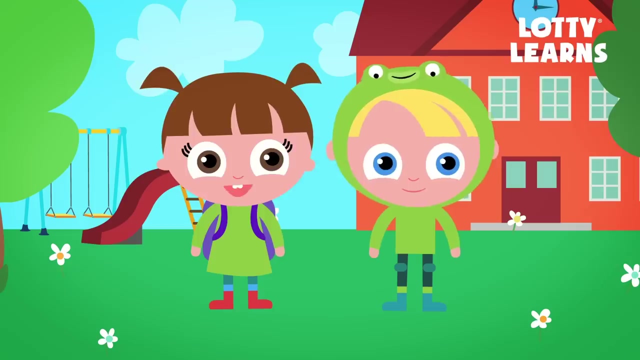 You should try the next lesson and collect even more stars. The more stars you collect, the more fun you can have See you next time. Hi there, These are my friends Chuck Hello and Chip. Hi there. Can you help them blend with the short E sound? eh? 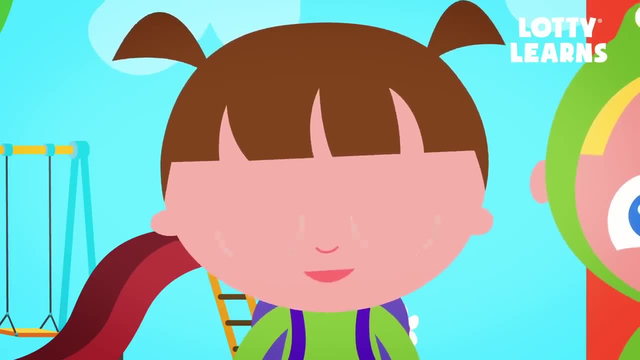 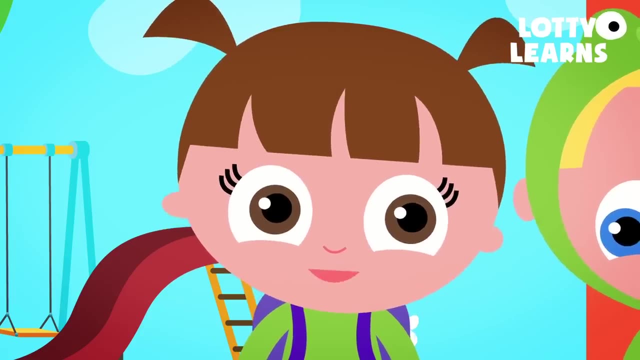 All you have to do is say the sound that each letter makes. Then put the sounds together. Try it with us. If you do a good job, you could win a gold star. We might even get to see something amazing. Here we go. 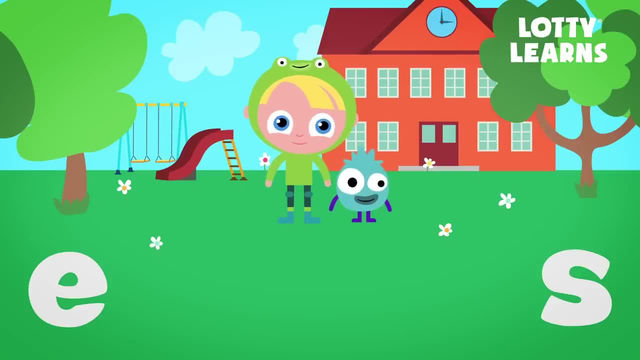 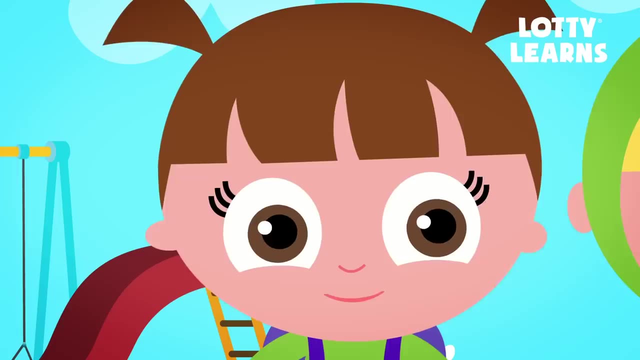 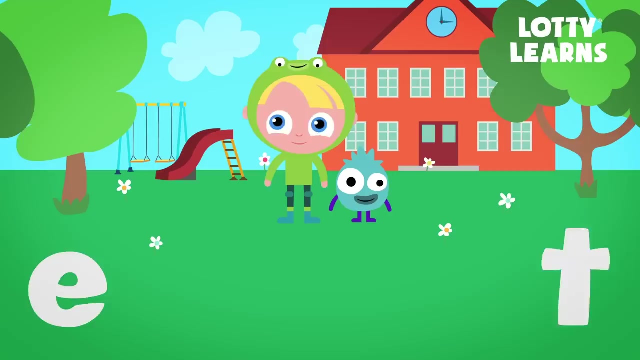 The E says eh and the S says ss, eh, ss, eh, ss, eh, ss. Great job, Keep it up. The E says eh and the T says tt, eh, tt, eh, tt, eh, tt. 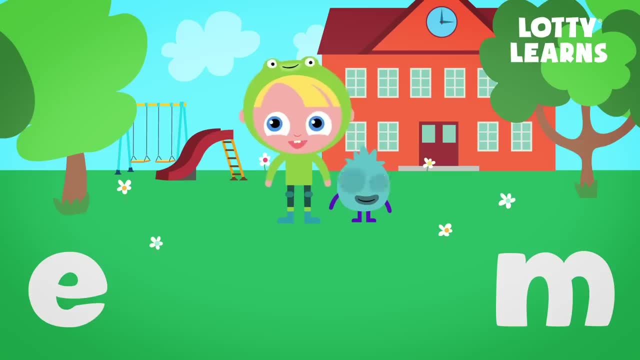 That's right, You're doing great. The E says eh And the M says m, eh, m, eh, m m. You're doing so well, I think you might get a prize. The E says eh and the P says p, eh, p, eh, p, eh p. 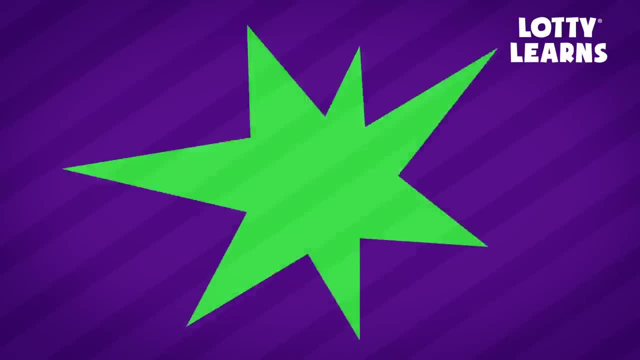 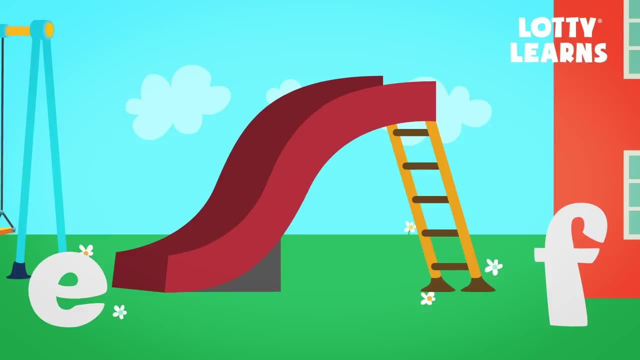 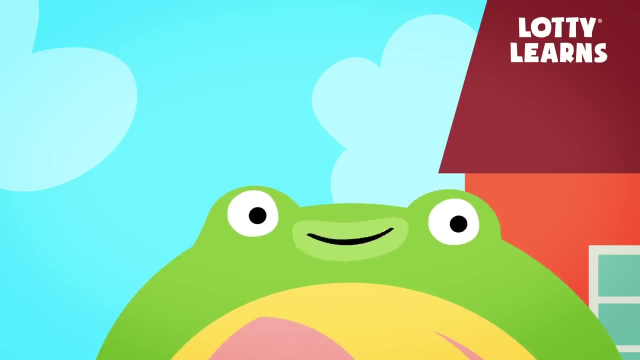 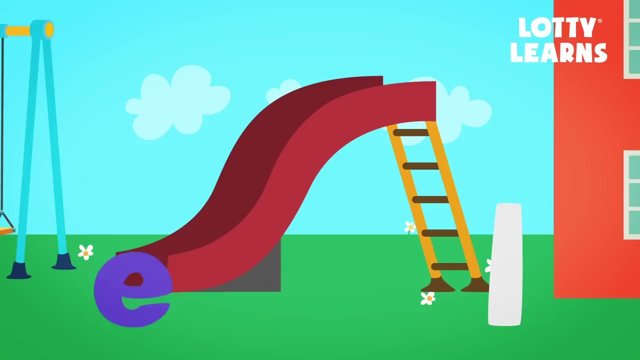 Gold star. You just won a gold star, Keep it up. The E says eh and the F says f, eh, f, eh, f, eh. Oh, yeah, You're doing great. The E says eh and the L says l eh, l, eh, l l. 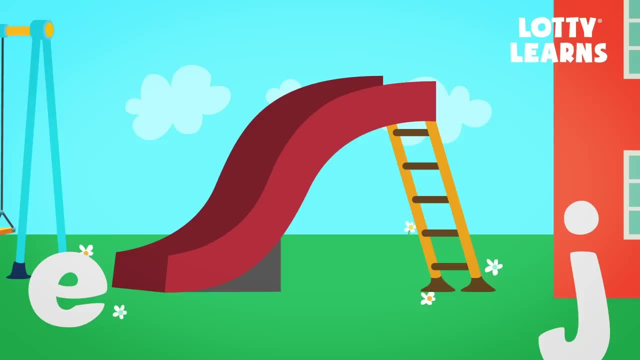 Almost done, Nice job. The E says eh and the J says j Eh, j Eh, j. Edge One more and we're all done. The E says eh and the D says d Eh, d. 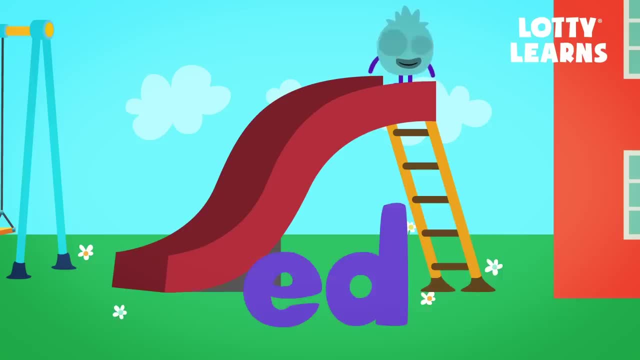 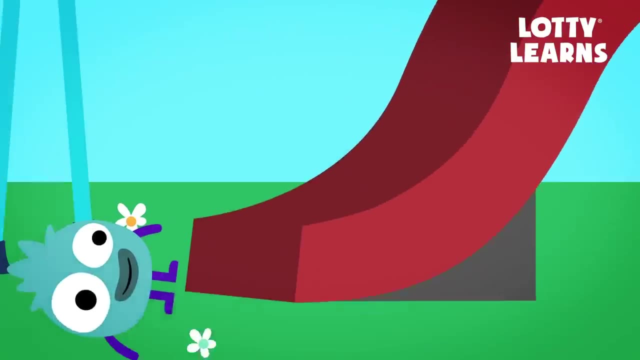 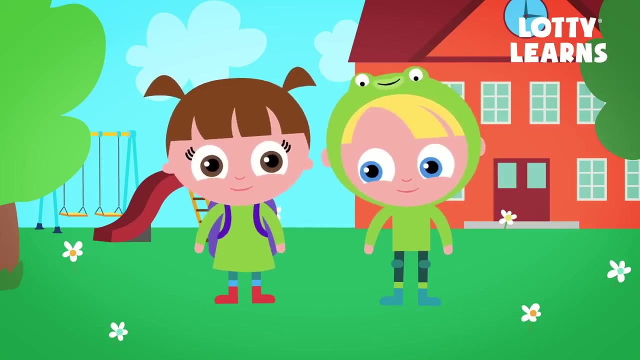 Eh d Edge. Great job. Let's see what Fuzz is up to. Fuzz is totally cool. We had such a fun time with you. Hope you visit us again soon. Remember to practice everything you learned today with your parents. 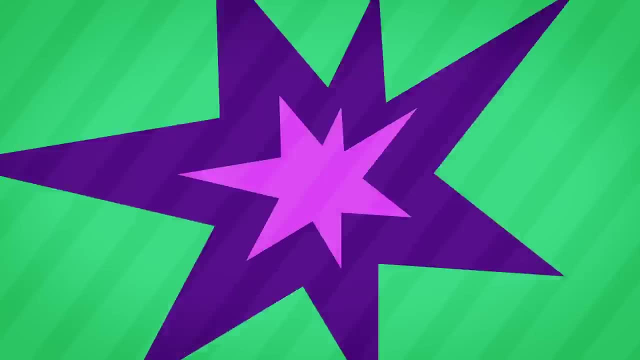 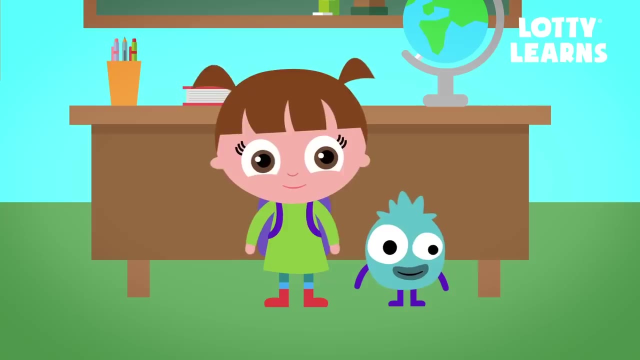 Don't forget to subscribe to our channel. Goodbye, LottieLearnscom. Letter Blending with the Short. I Hello again, friend. Isn't school fun. Let's blend with the short I sound. ih Just say the sound that each letter makes. 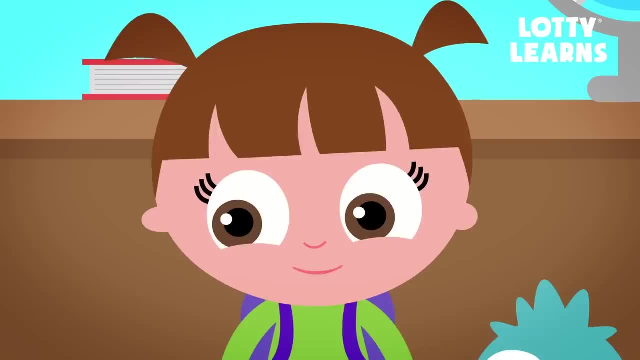 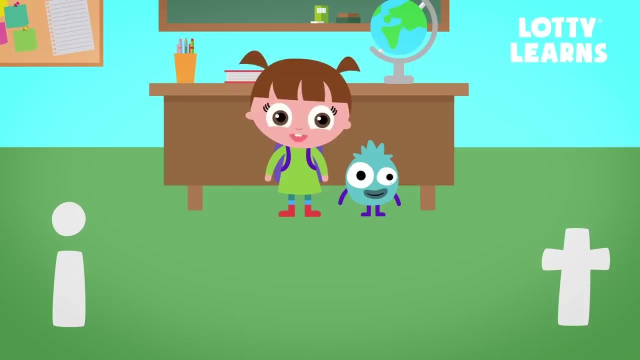 Then put the sounds together. Try it with me. If you do a good job, you could win a gold star. You might even get to see Chip or Fuzz do something silly. Here we go. The I says ih and the T says t. 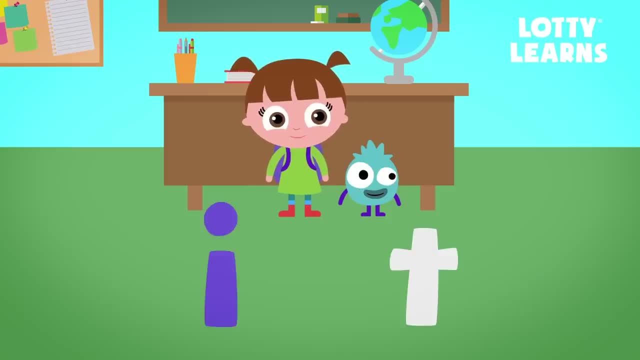 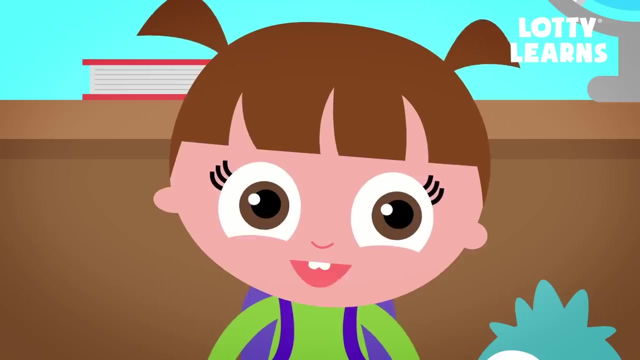 Eh t, Eh t. It Super smart. The I says ih and the S says ss, Ih ss, Ih ss, Ih ss. Isn't this fun. The I says ih And the P says p. 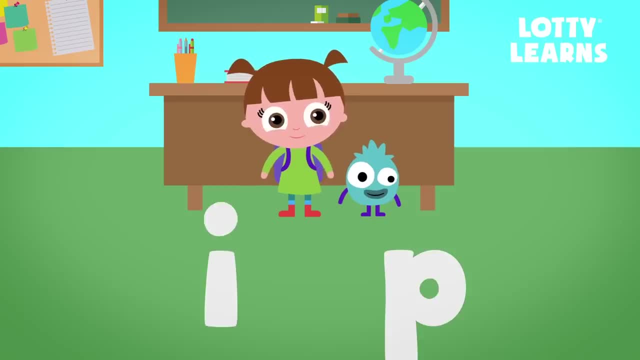 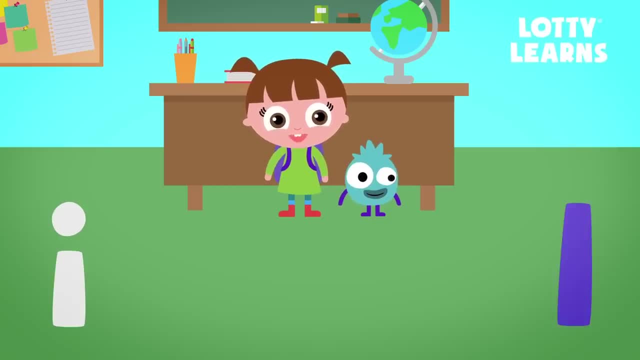 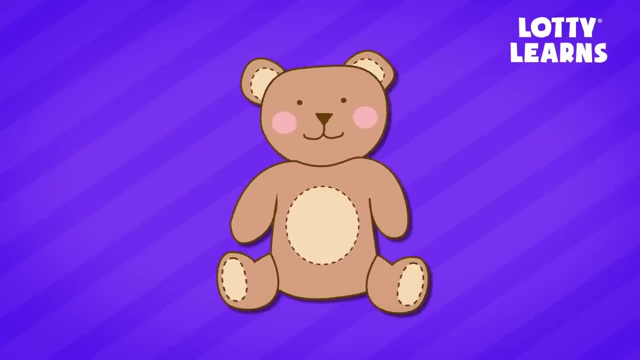 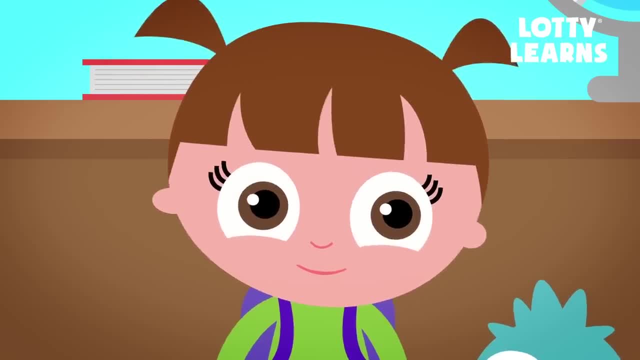 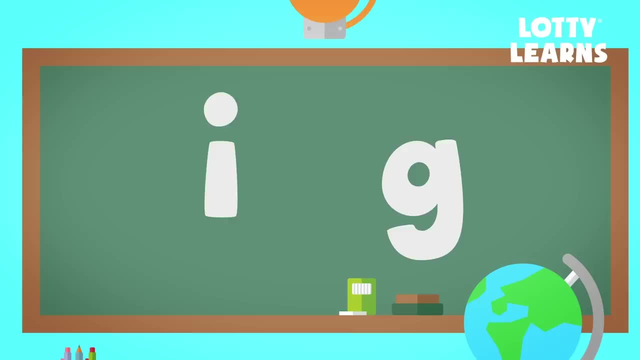 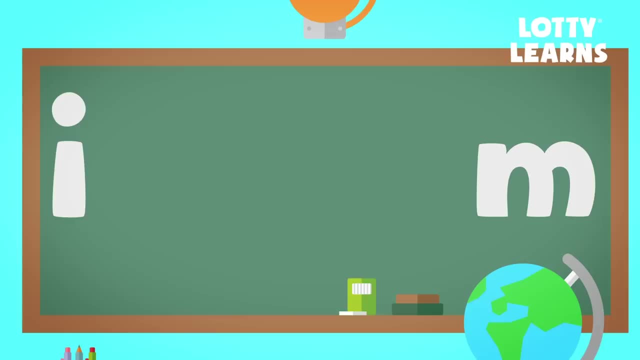 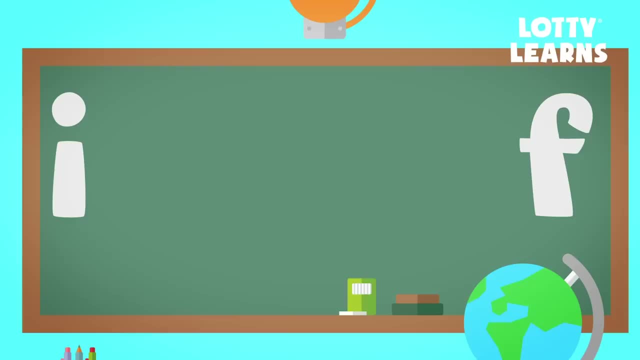 We won another. Alright, Let's do another for the kids too. Both of you finish up: If, if, if, One more and we're all done. The I says if and the N says mm, I, mm, I, mm in. 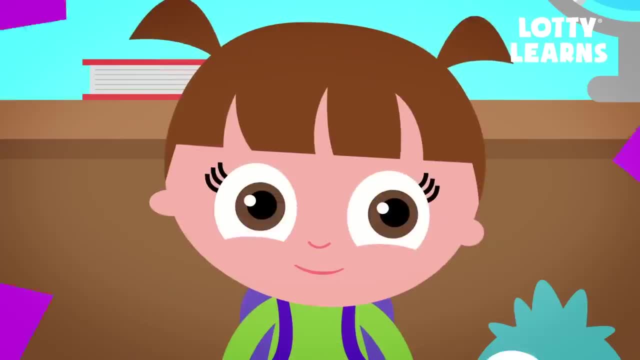 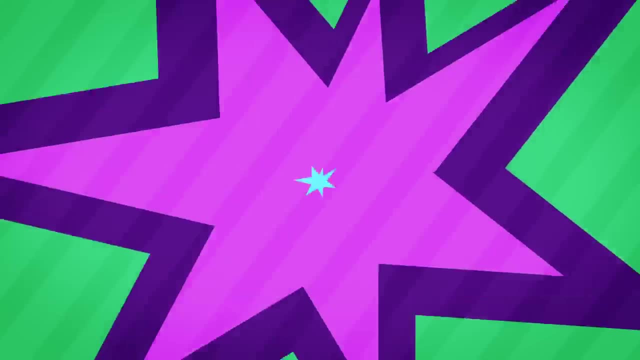 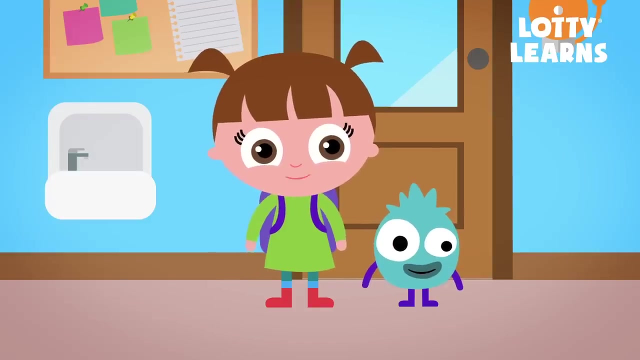 Gold star. Great job. Thanks for learning with us. We had such a fun time with you. Hope you visit us again soon. LottieLearnscom Letter blending with the short: O: Hi, I'm Lottie and this is Fuzz. 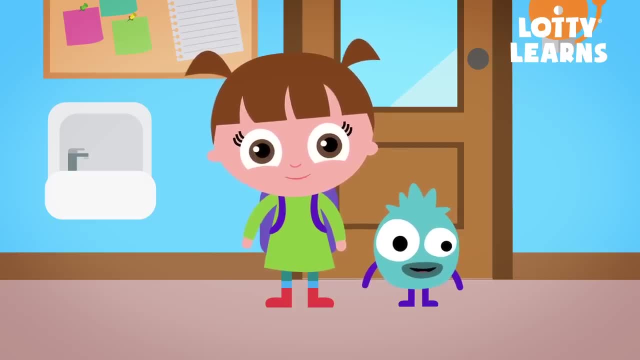 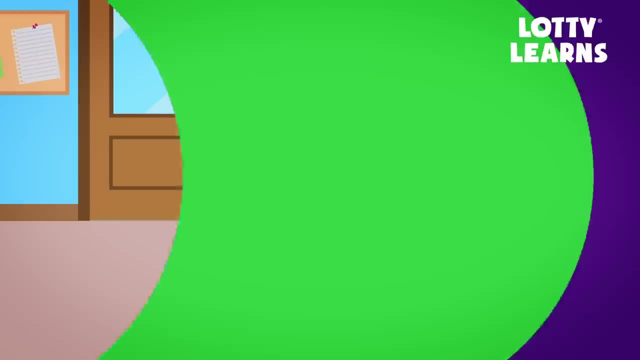 Can you help Chuck and Chip blend with the short O sound aw before the school bell rings. All you have to do is say the sound that each letter makes, then put the sounds together. Try it with us. The O says aw and the N says nuh. 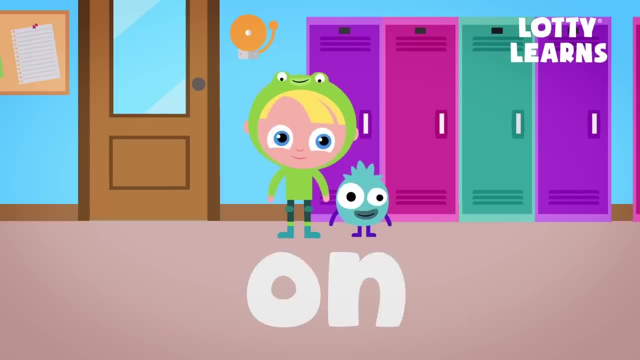 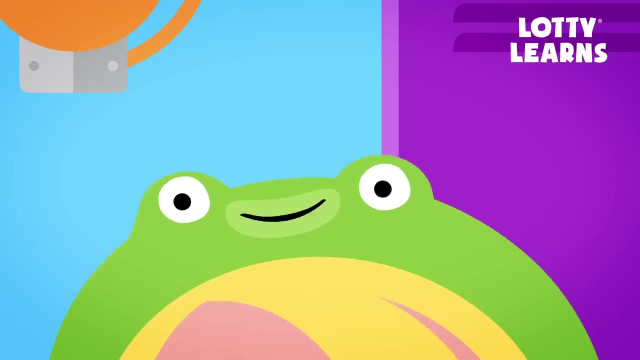 Aw nuh, Aw nuh. On Super, You're smart. The O says aw and the T says tt, Aw, tt, Aw, tt, Aw, tt. This is fun. Let's keep going. 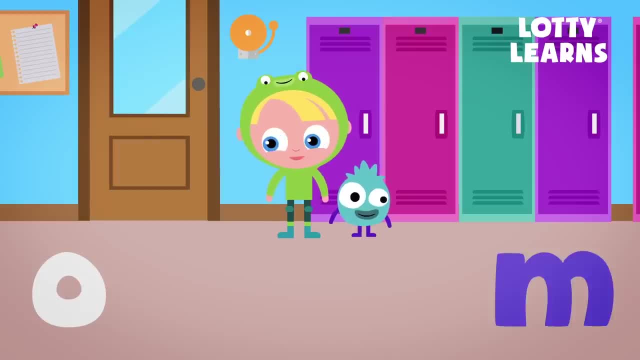 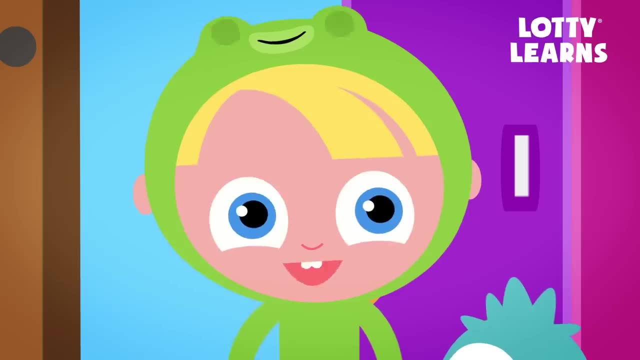 The O says aw and the M says mm Aw, mm Aw, mm. Om You're doing so well, I think you might get a prize. The O says aw and the P says nuh. 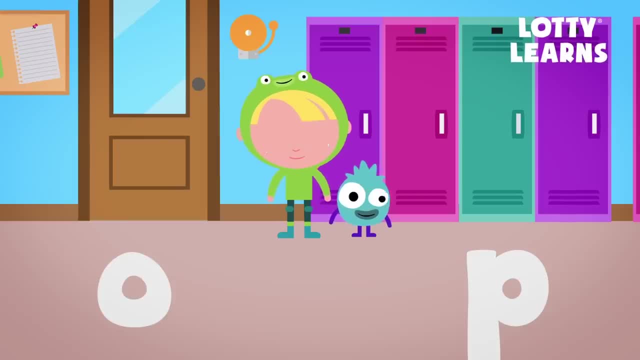 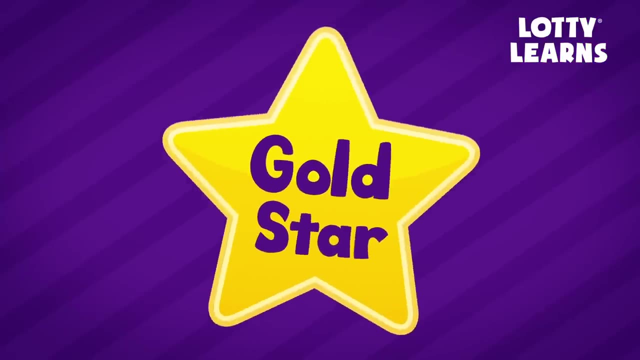 And the P says ph aw, ph aw opp Gold star. You just won a gold star, Keep it up. The O says aw and the B says b Aw, b aw, b Awb. 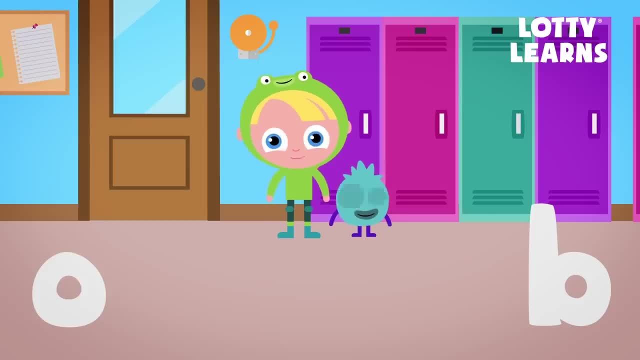 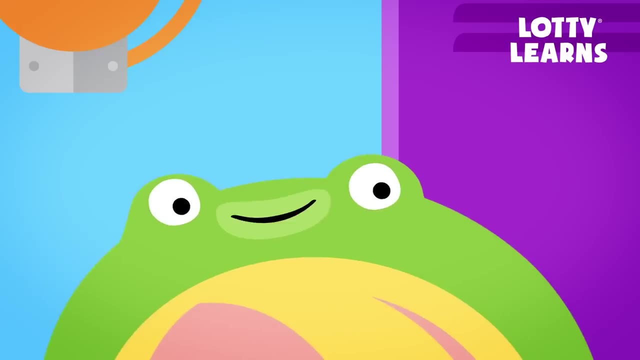 You're doing awesome. The O says aw and the D says nuh, Aw, nuh, Aw, nuh, Nuh, Aw, nuh, Nuh nuh. You did awesome, Almost done, Nice job. 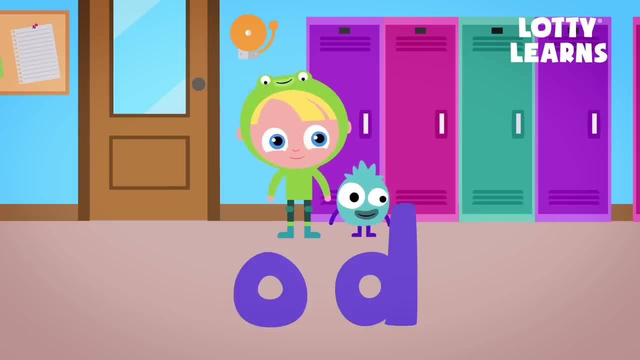 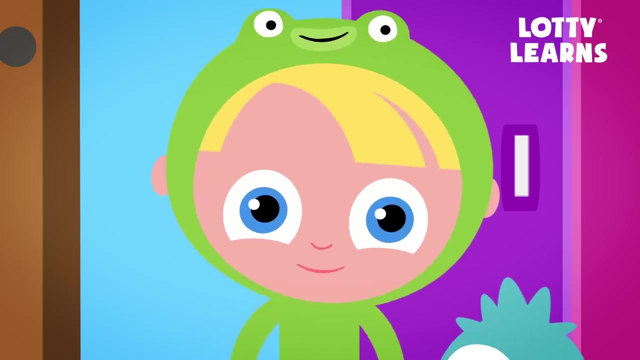 The O says aw and the Z says zz, Aw, zz, Aw, zz, Aw, zz. One more and we're all done. The O says aw and the G says g, Aw, g, Aw, g. 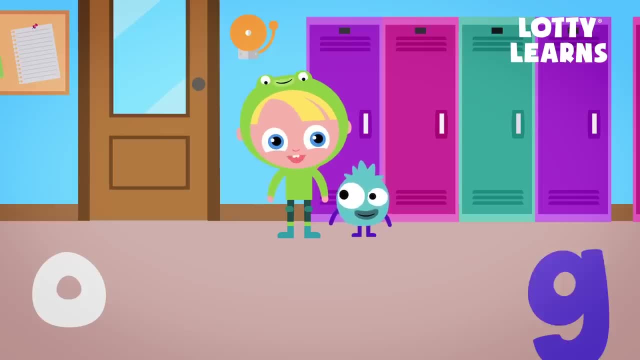 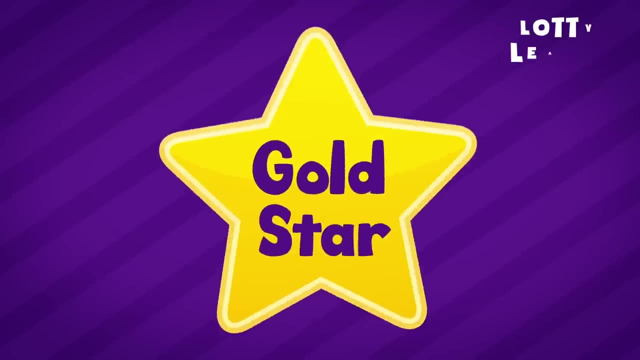 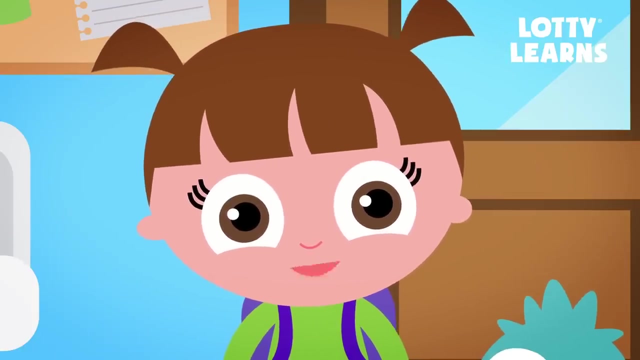 Awg, Awg, Awg, Awg, Awg- Gold star. You should try the next lesson and collect even more stars. Thanks for learning with us. We had such a fun time with you. Hope you visit us again soon. 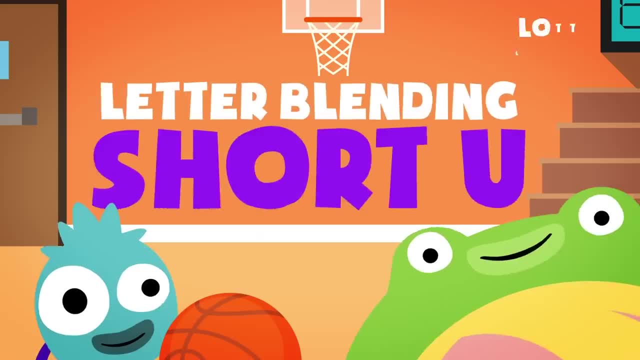 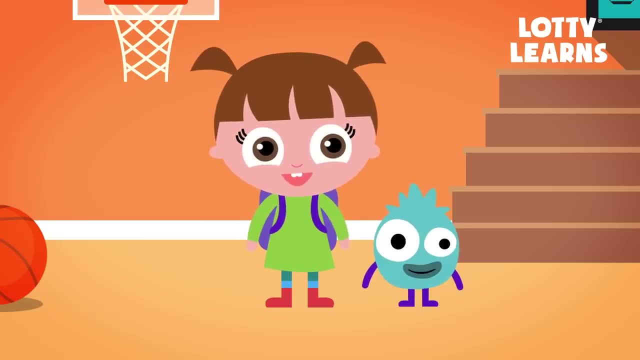 LottieLearnscom Letter Blending with the Short U: Hi, I'm Lottie and this is Fuzz. Let's blend with the short U: sound, uh, Just say the sound that each letter makes, Then put the sounds together. 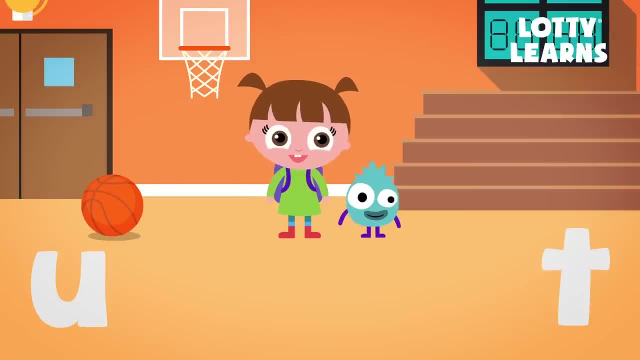 If you do a good job, you could win a gold star. Here we go. The U says uh and the T says t Uh, t Uh, t Ut Super smart. The U says uh and the P says p. 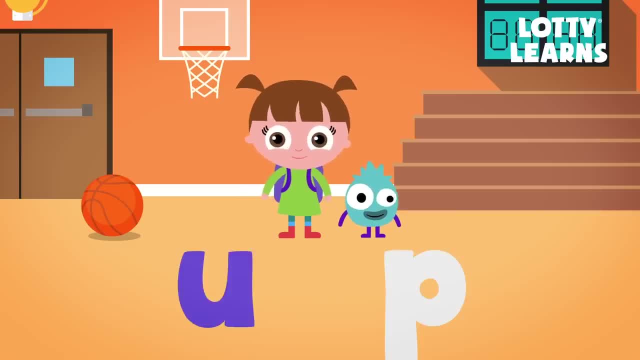 Uh, p, Uh, p Up. Great job, Keep it up. The U says uh And the M says mm, Uh, mm, Uh, mm. Um, You're doing so well. I think you might get a prize. 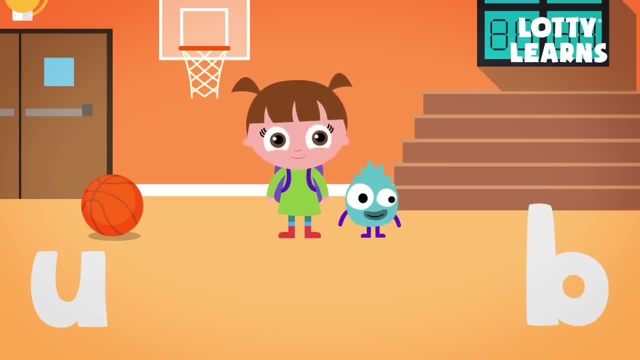 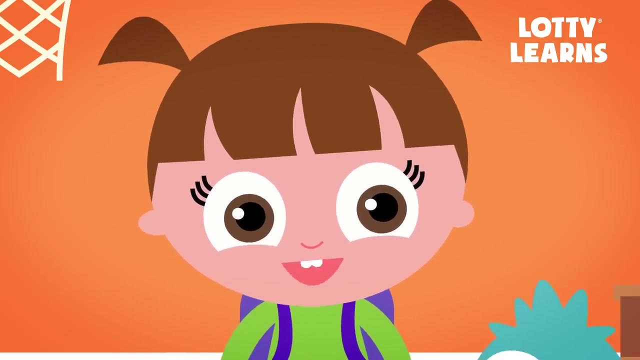 The U says uh And the B says buh, Uh, buh, Uh, buh, Uh buh. Nice job, You just won a sticker, Super smart, Let's do another. The U says uh And the G says guh. 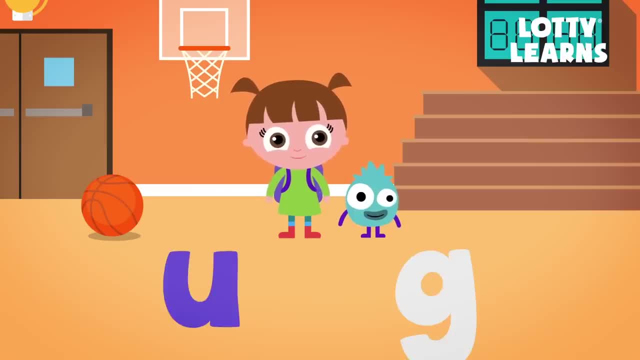 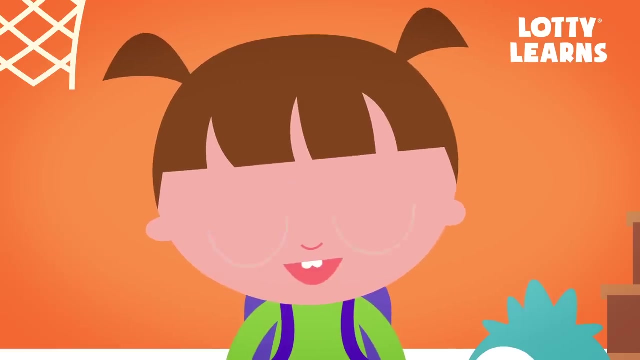 Uh guh, Uh guh, Uh guh, Great job, Keep it up. The U says uh And the S says ss, Uh, ss, Uh, ss, Us. Almost done, Nice job. The U says uh. 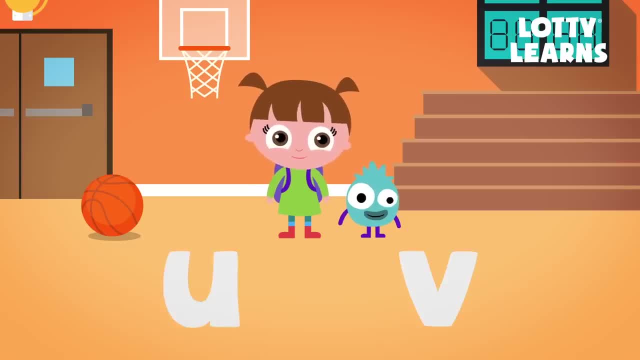 And the V says mm, Uh, mm, Uh, mm Of One more and we're all done. The U says uh And the N says mm, Uh, mm, Uh, mm. Un Gold star, You should try the next lesson. 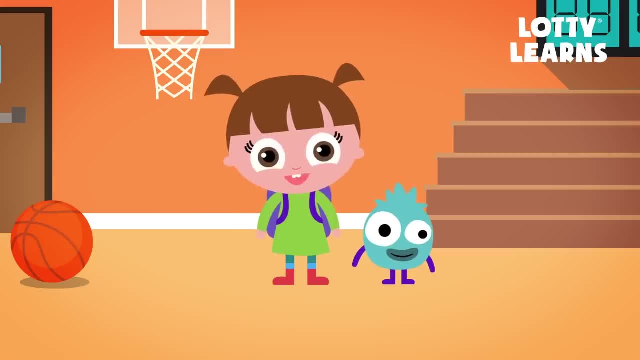 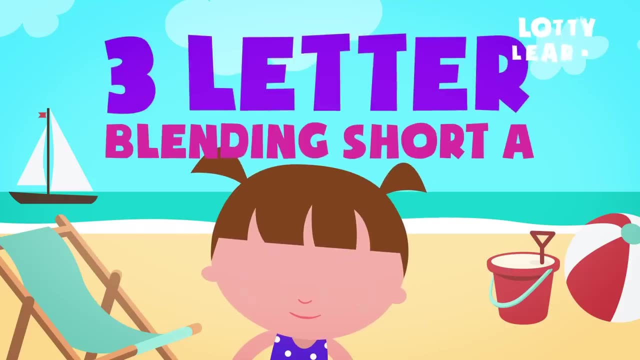 and collect even more stars. Thanks for learning with us. We had such a fun time with you. Hope you visit us again soon. LottieLearnscom. Three-letter blending with the short A. I'm Lottie and this is Fuzz. 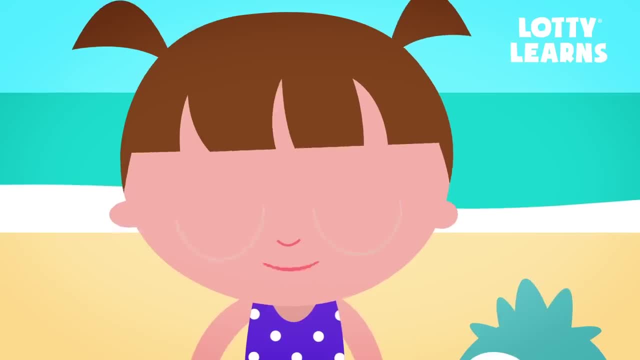 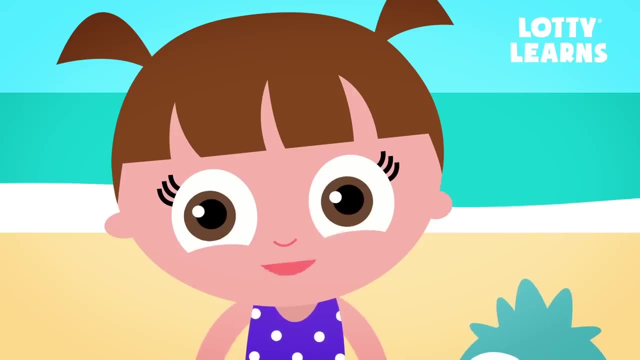 Hang out at the beach with us. We're going to blend three letters together using the short A sound eh. First we'll put two letters together, like we've done before, But this time we'll add one more letter to the beginning. 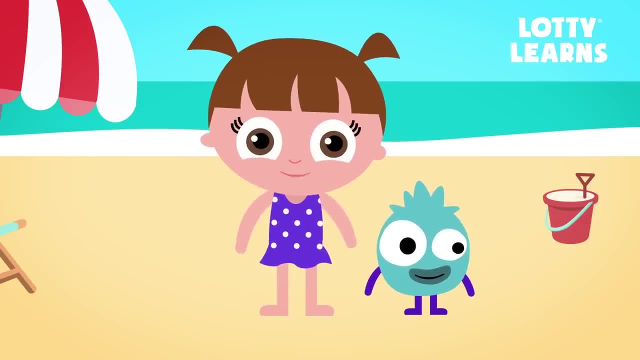 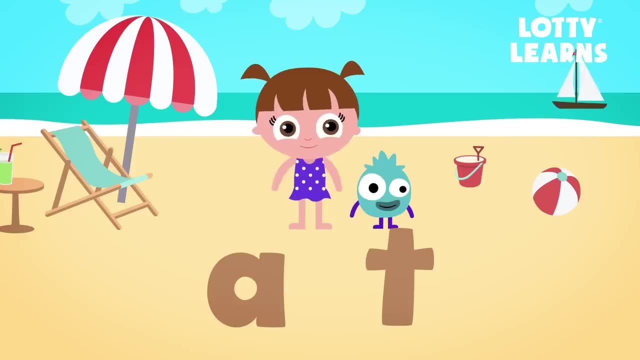 Try and do your very best so you could win a gold star and even get to see Fuzz do something silly. Here we go. This says eh At. Now that we know A and T say at: let's try and put a few other letters. 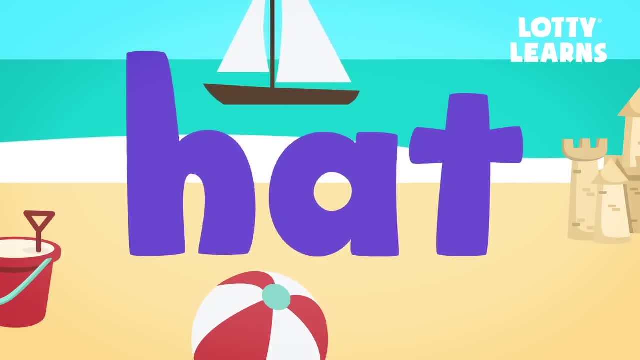 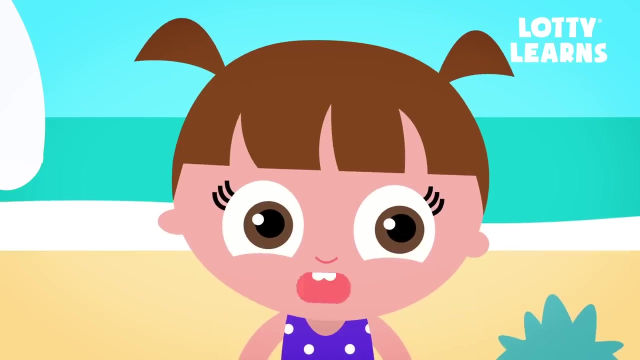 at the beginning: Huh At Hat Ss At Sat Buh At Bat Cuh At Cat Rr At Rat Mm At Mat. Awesome job, This says eh. 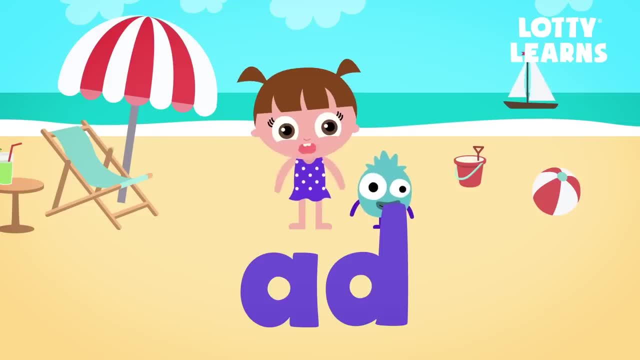 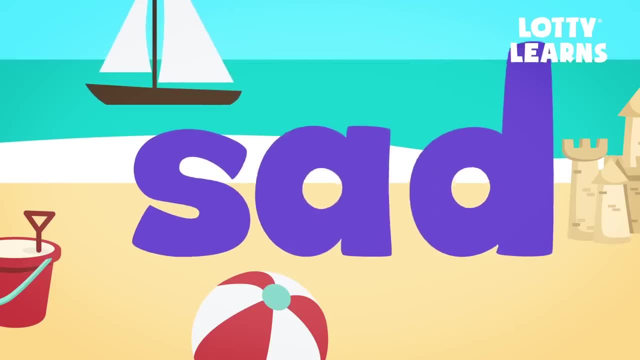 Duh Ad. Now that we know A and D say ad. let's try and put other letters at the beginning: Ss Ad Sad Tuh Ad. Tad Buh Ad Bad Duh Ad. 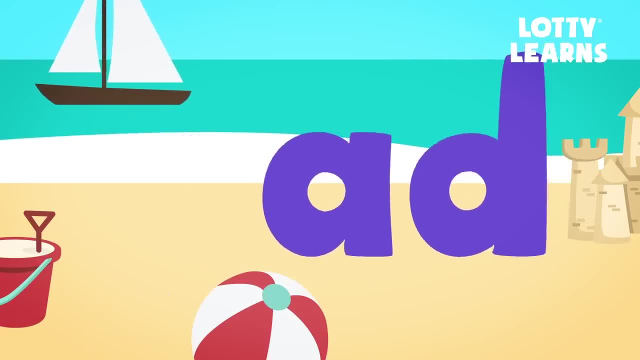 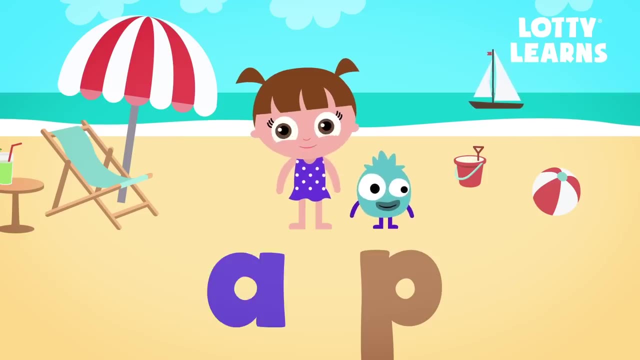 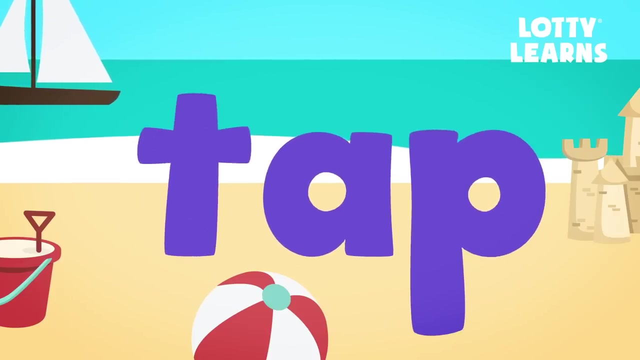 Dad Ad Pad, Mm Ad Mad Great. This says: eh, Puh, App. Now that we know A and P say app, let's try and put other letters at the beginning: Ss, App, Sap. 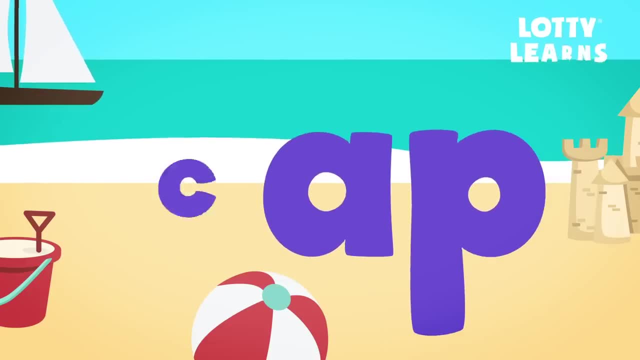 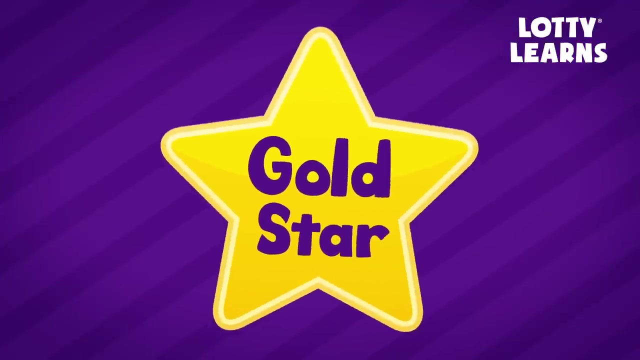 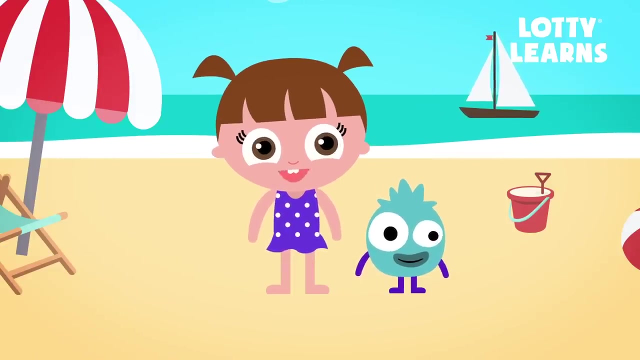 Tt App Tap, Nn App Cap, Rr App Rap, Mm App Map. Amazing Gold star. You should try the next lesson and collect even more stars The more stars you collect. 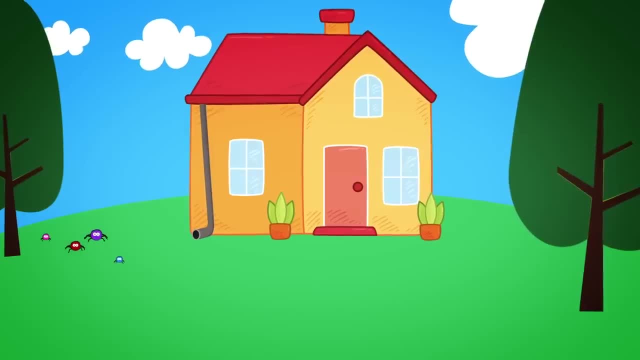 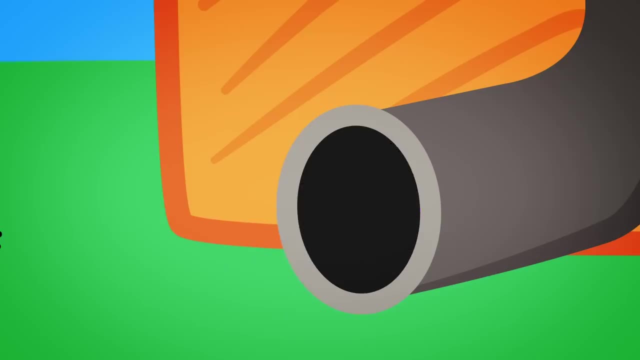 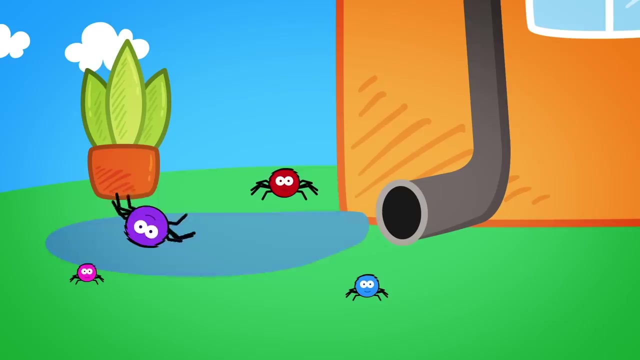 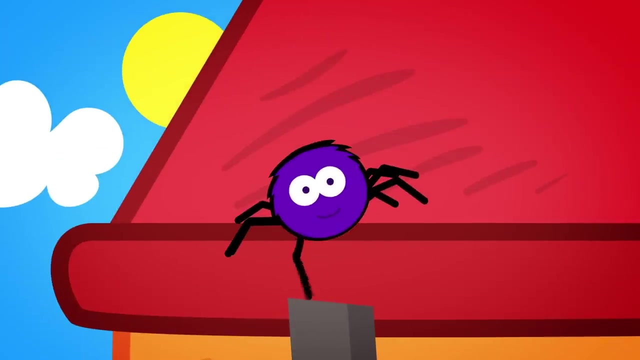 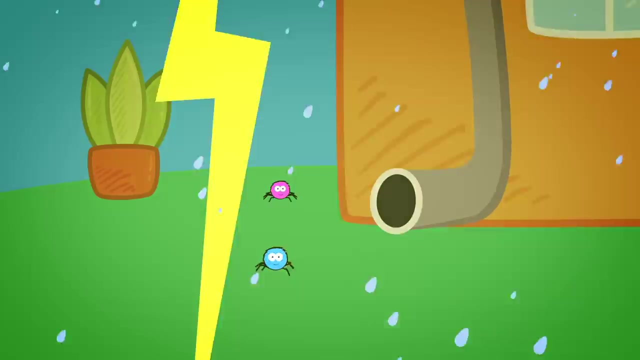 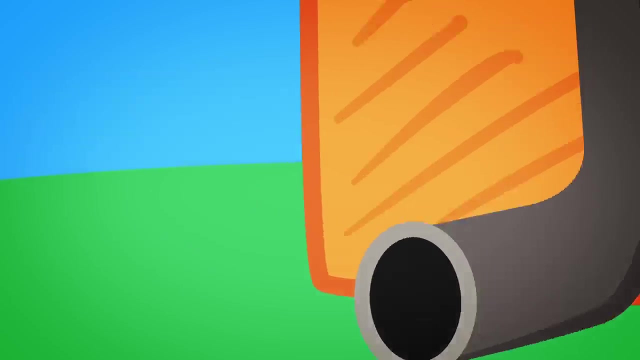 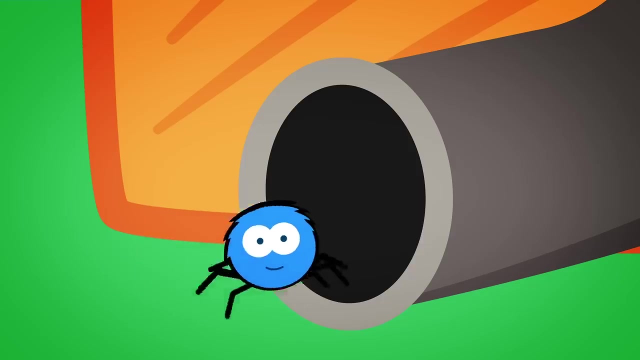 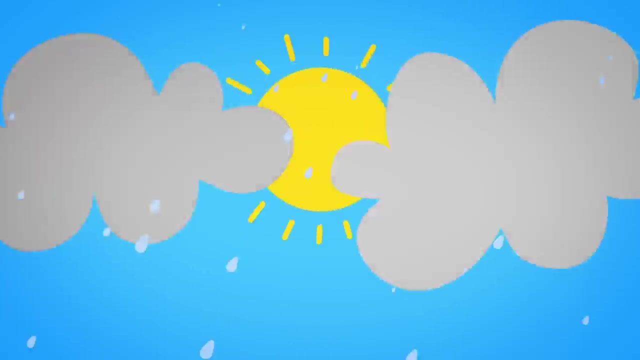 the more fun you can have. Remember to subscribe. See you next time. Bye, Baby tower spider. The look with the spider without the water spout. Down came the rain And washed the spider out. Up came the sun And dried up all the rain. 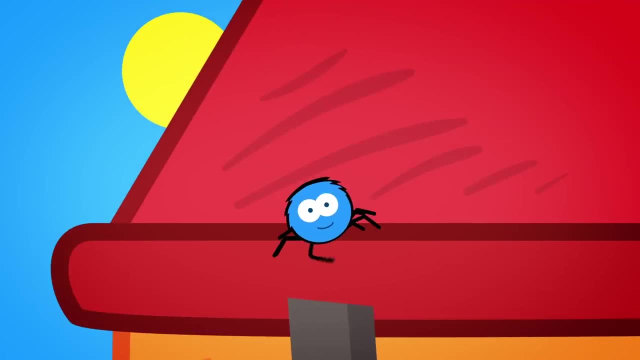 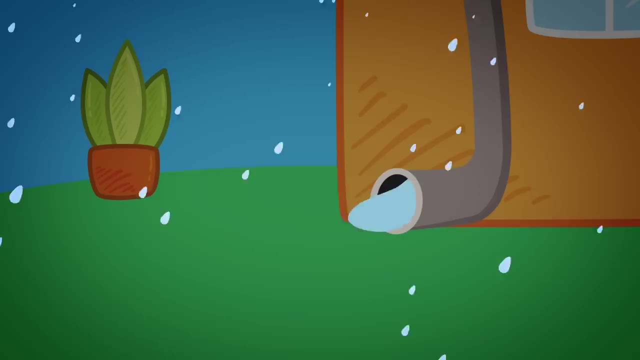 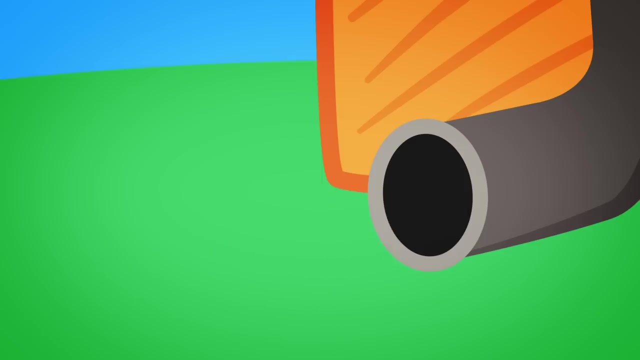 So the itty bitty spider Went up the spout again. Baby sister spider. The itty bitty spider Went up the water spout. Down came the rain, Up came the sun, and it ride up all the rain. so the itsy bitsy spider went up the spout again. 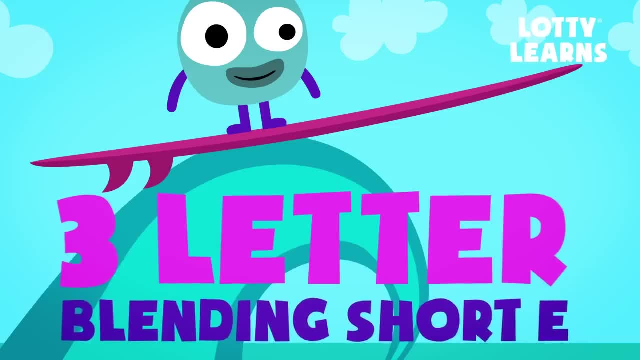 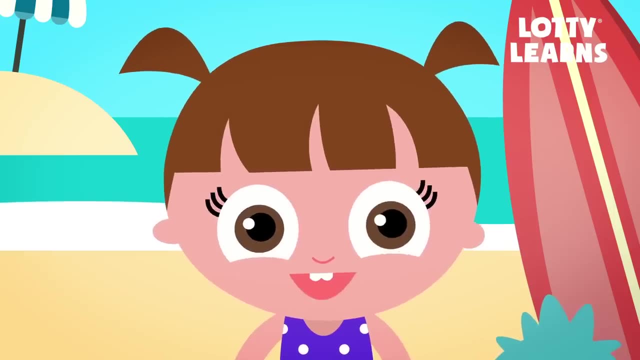 LottieLearnscom. Three-letter blending with a short E. Hi, I'm Lottie and this is Fuzz. Today we're going to blend three letters together using the short E sound. eh, First we'll put two letters together, like we've done before. 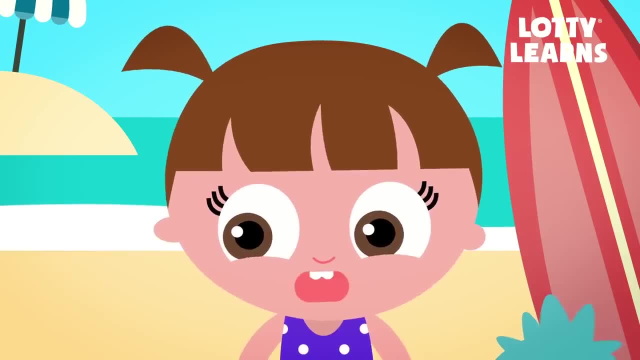 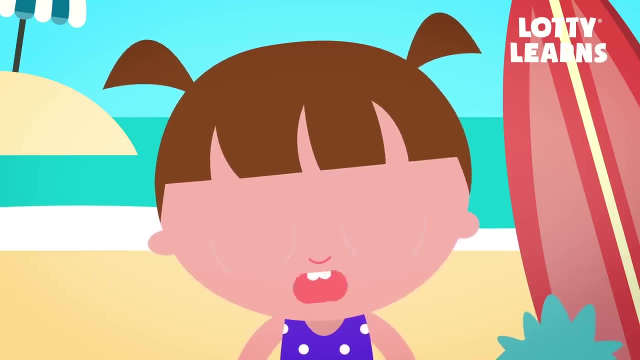 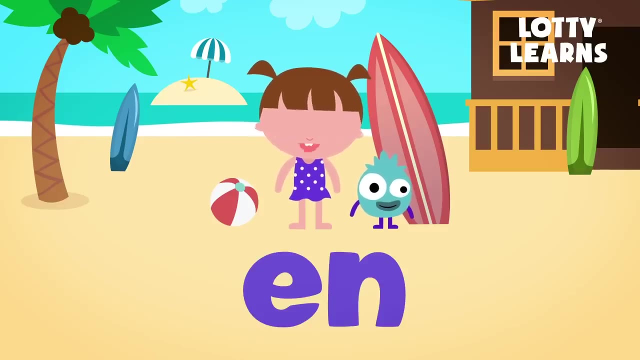 But this time we'll add one more letter to the beginning. Try and do your very best so you could win a gold star and even get to see Fuzz go surfing. Here we go. This says eh, nn- n. Now that we know E and N say n, let's try and put other letters at the beginning. 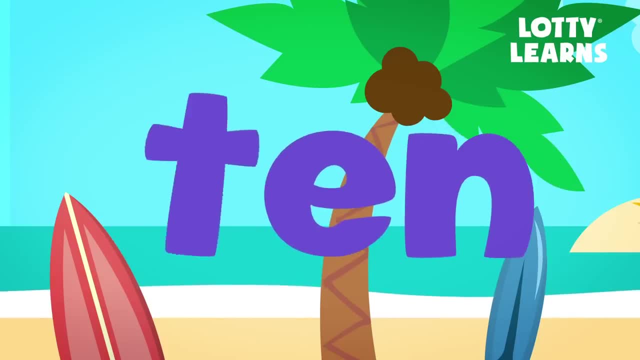 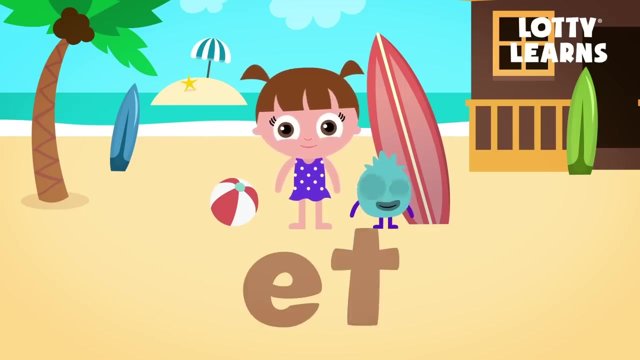 N hen T en ten F en pen D en den P en pen Z en zen. Awesome job. This says eh t, et. Now that we know E and T say et, let's try and put other letters at the beginning. 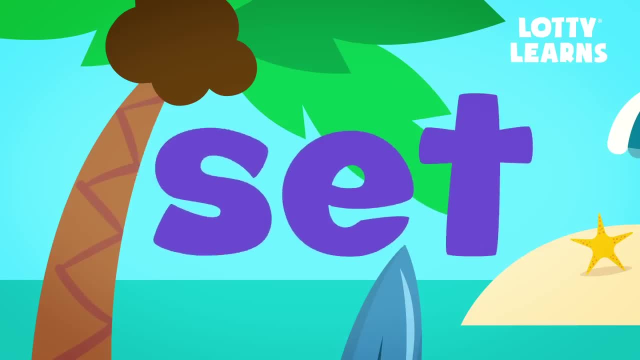 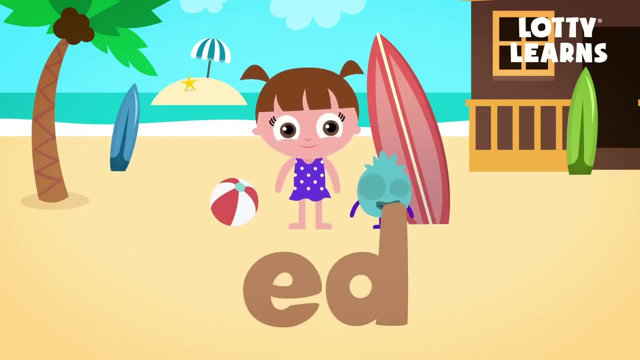 S et set P et pet N et net W et wet G et get M et met Great. This says eh, d, ed. Now that we know E and D say ed. 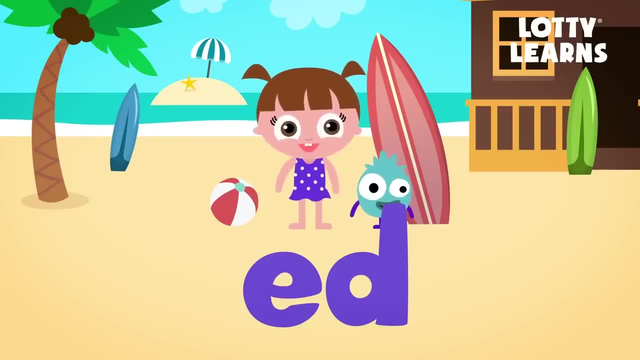 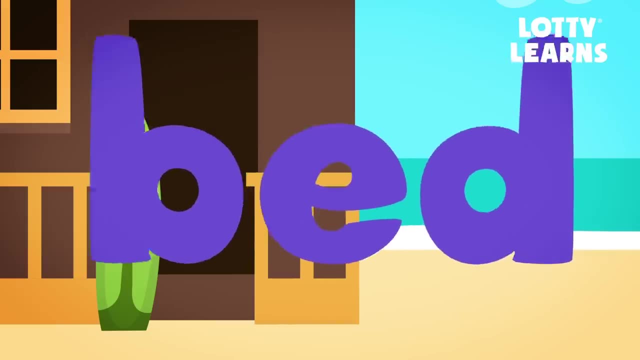 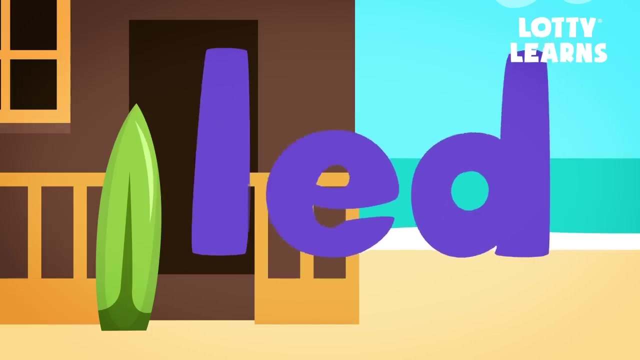 let's try and put other letters at the beginning: Ed bed, B, ed bed R, ed red M ed, med T ed, ted, L ed led. Amazing You're doing so well. Let's see what Fuzz is up to. 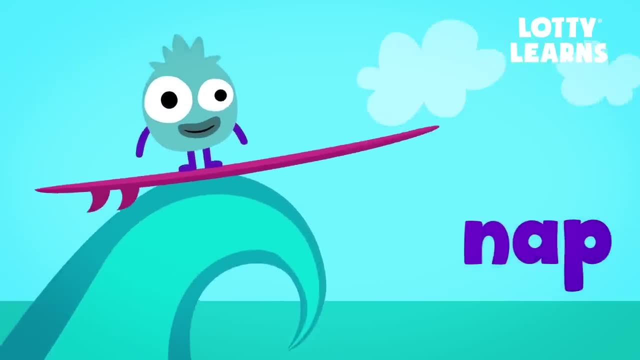 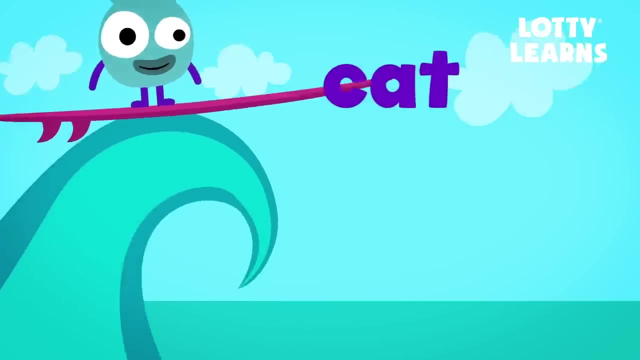 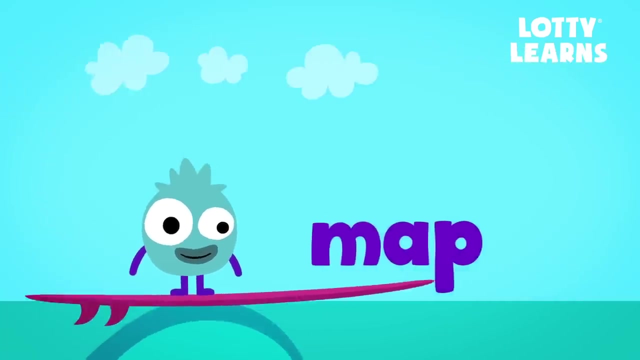 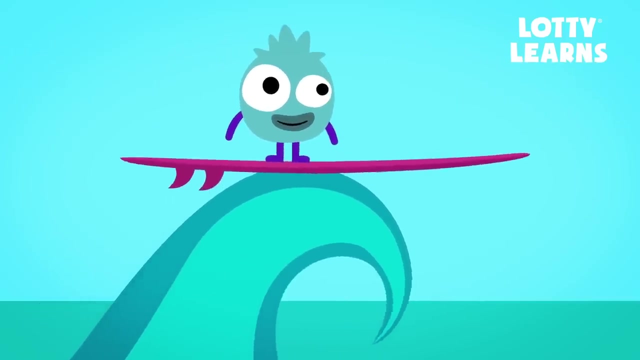 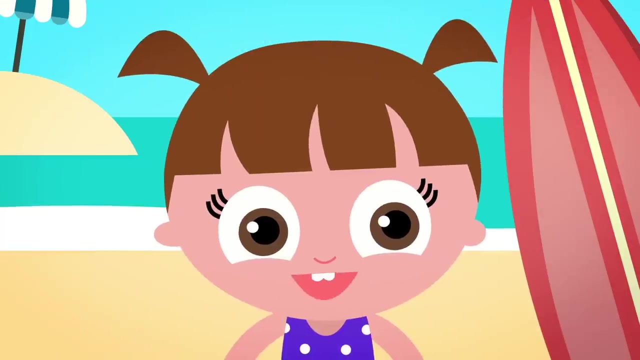 Let's see what Fuzz is up to Nap. Great job Hat Cat. Super smart Pad Map. Nice job Bad. That was awesome. Gold star Fuzz is totally cool. You should try the next lesson and collect even more stars. 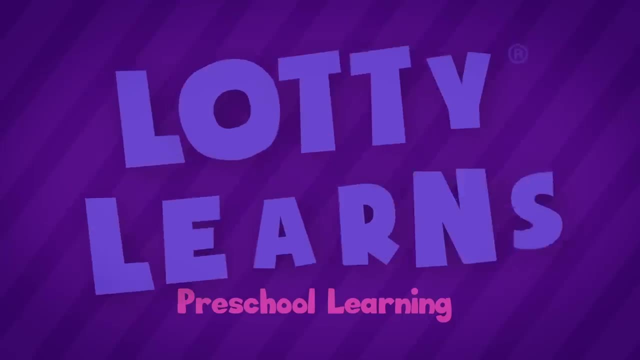 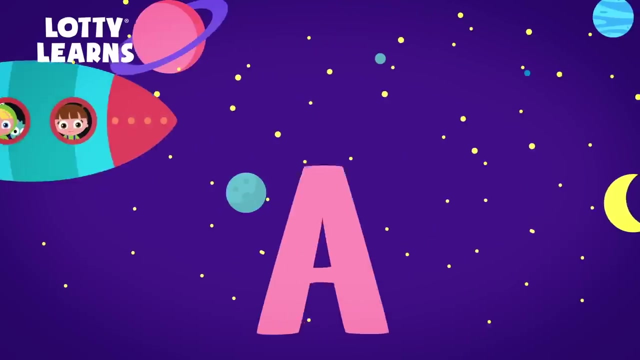 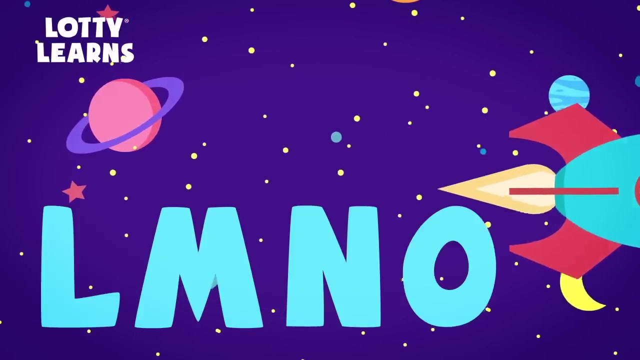 The more stars you collect, the more fun you can have. LottieLearnscom Uppercase A, B, C, D, E, F, G, H, I, J, K, L, M, N, O, P. 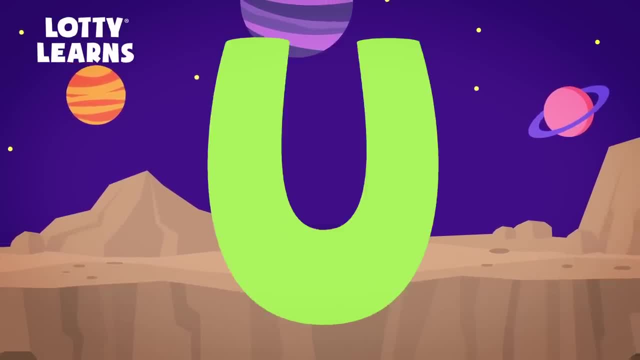 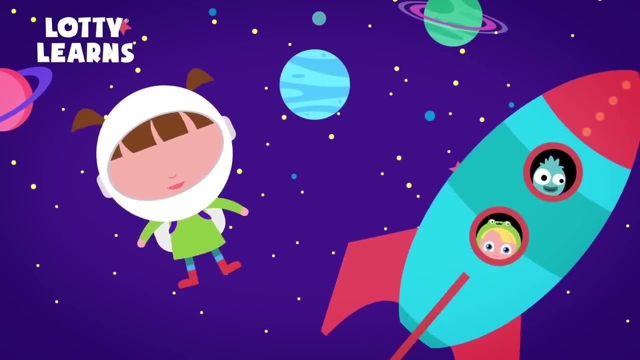 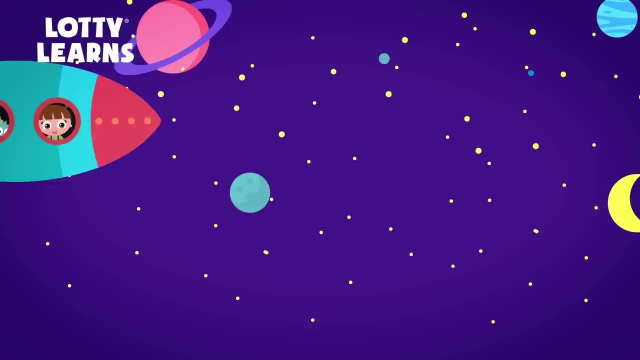 Q, R, S, T, U, V, W, X, Y and Z. Now I know my ABCs. Next time won't you sing with me Lowercase A, B, C, D, E, F, G. 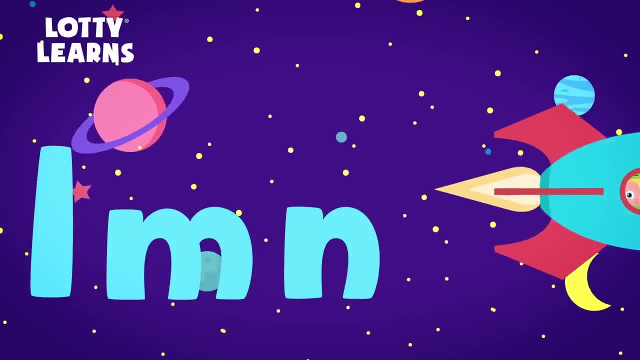 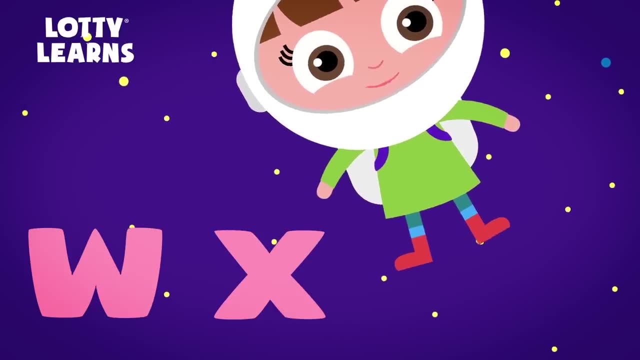 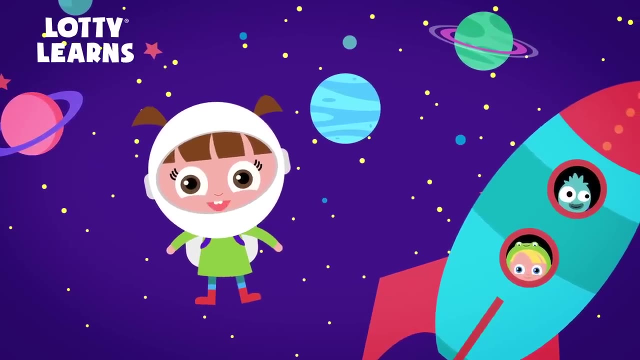 H, I, J, K, L, M, N, O, P, Q, R, S, T, U, V, W, X, Y and Z. Now I know my ABCs. Next time won't you sing with me? 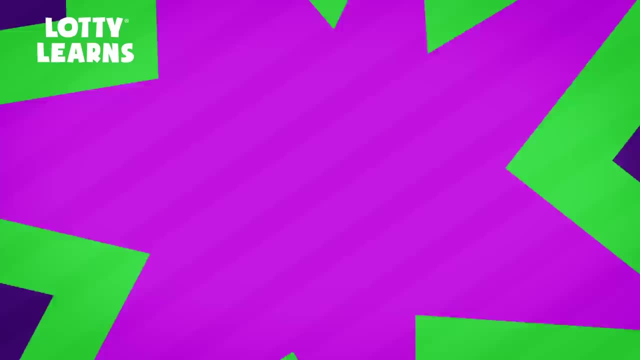 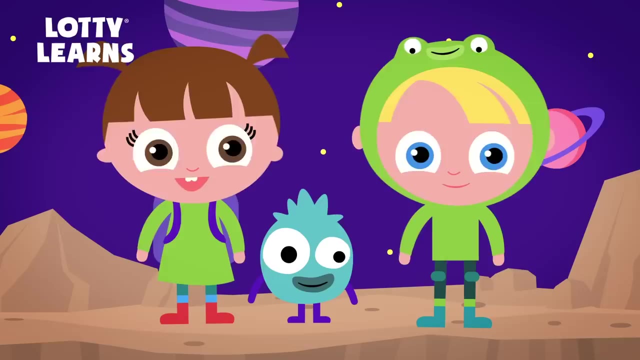 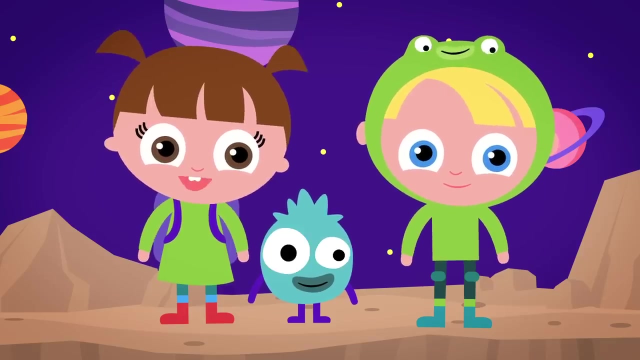 Gold star. That was all of the upper and lowercase letters. Great job. If you ever forget what the letters look like, just watch this video again. Thanks for learning with us. We had such a fun time with you. Hope you visit us again soon. 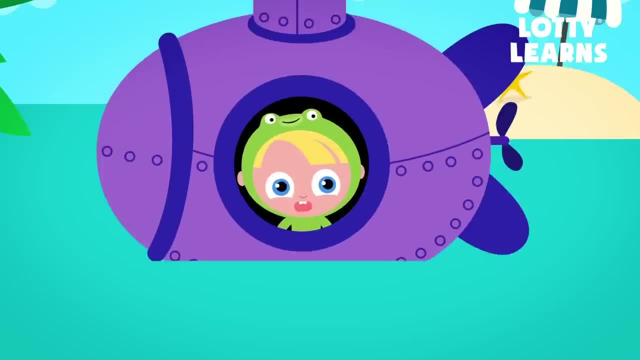 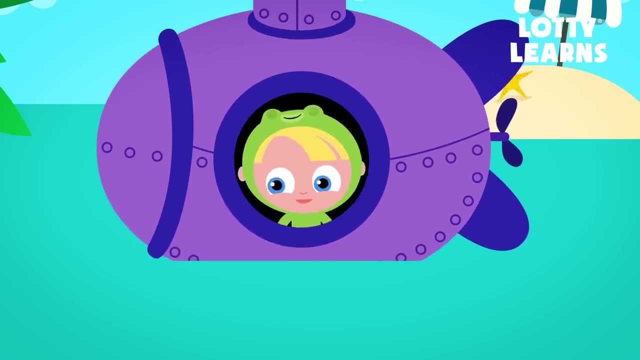 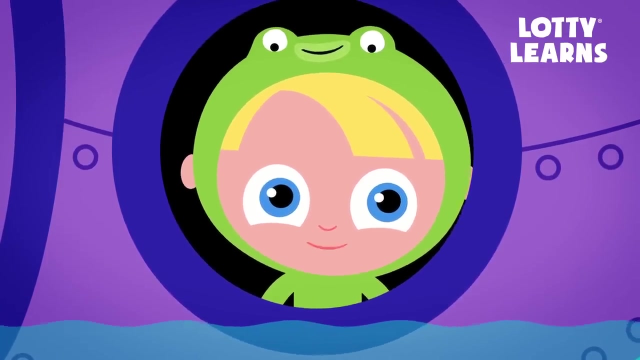 Three-letter blending with the short I. Hi there, I'm Chuck and this is my friend Chip. What's up? Today we're going to blend three letters together using the short. I sound I First. we'll put two letters together, like we've done before. 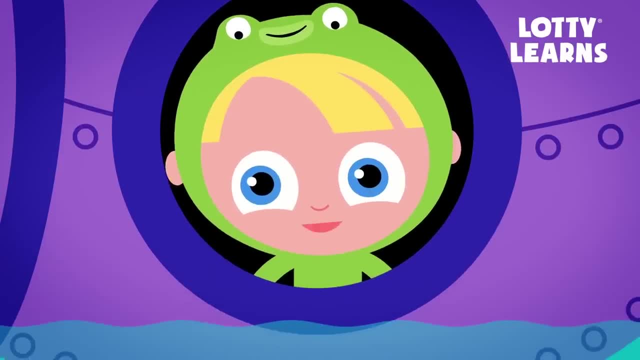 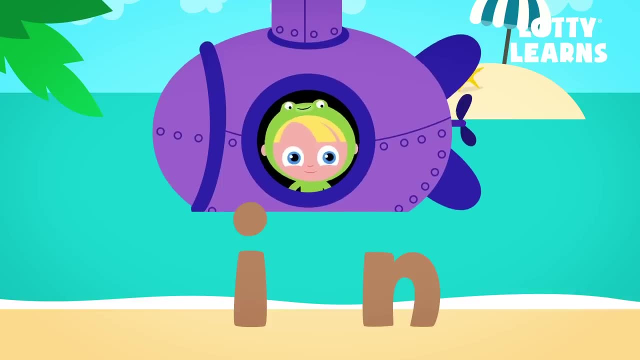 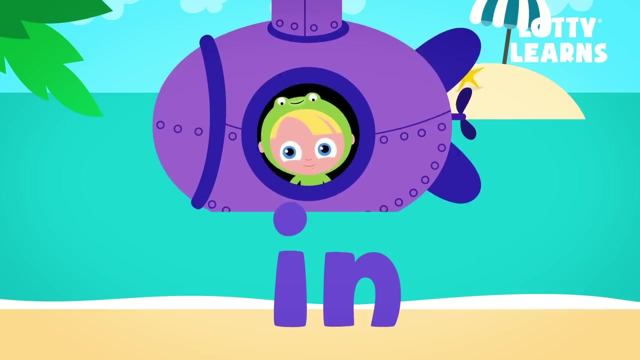 but this time we'll add one more letter to the beginning. Try and do your very best so you could win a sticker and even get to see something silly. Here we go. It says I-N In. Now that we know I and N say in. 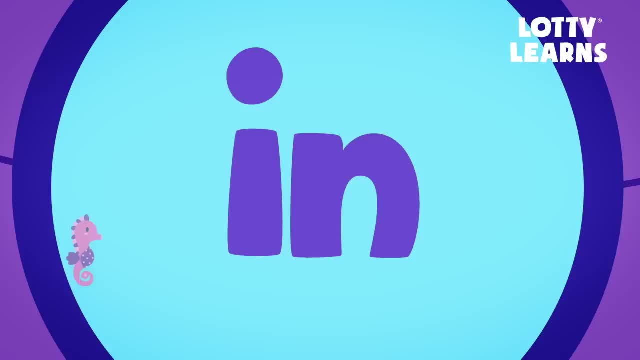 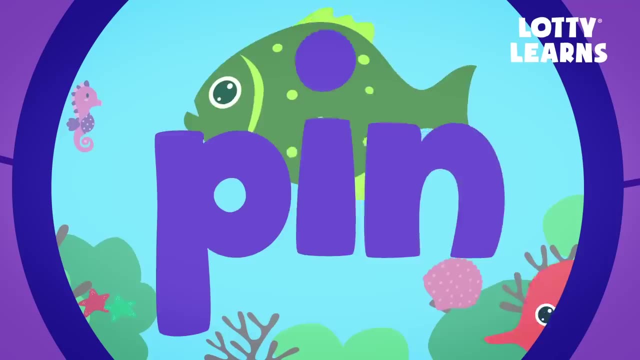 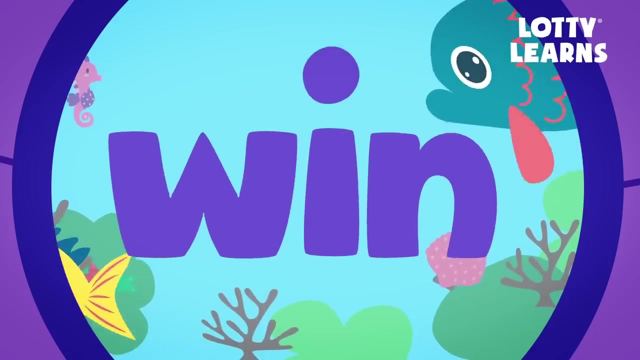 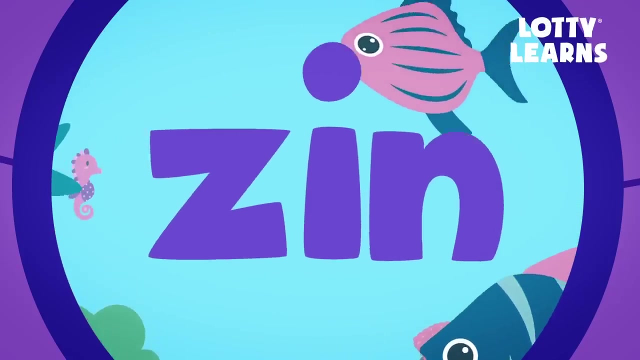 let's try and put other letters at the beginning: In T In Tin, P, In Pin B, In Bin W, In Win F, In Fin Z, Z In Zin. 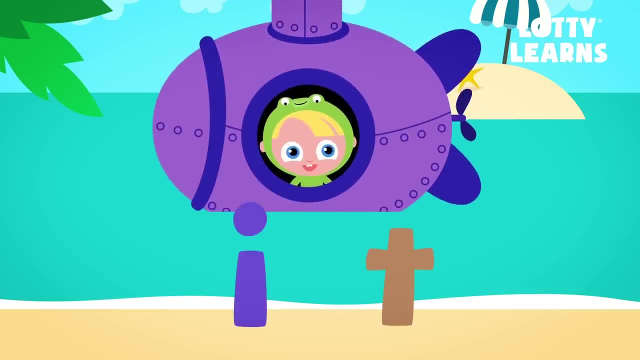 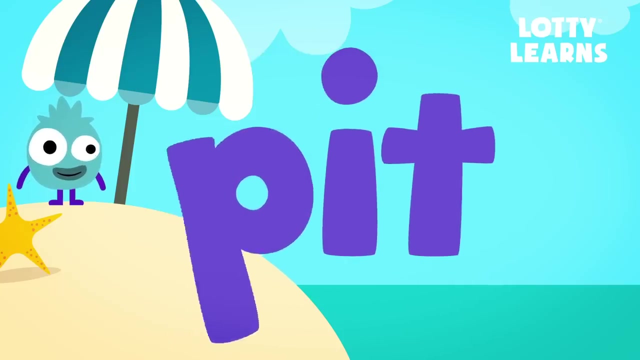 Awesome job. This says I-T It. Now that we know I and T say it, let's try and put other letters at the beginning. S It Sit P It Pit, S It Fit S. 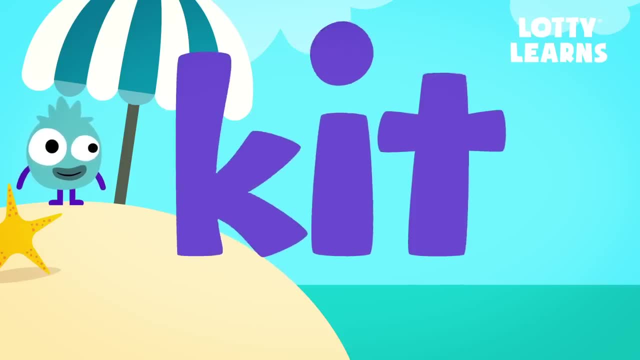 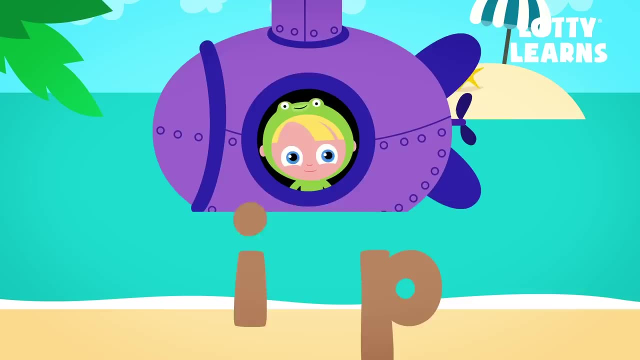 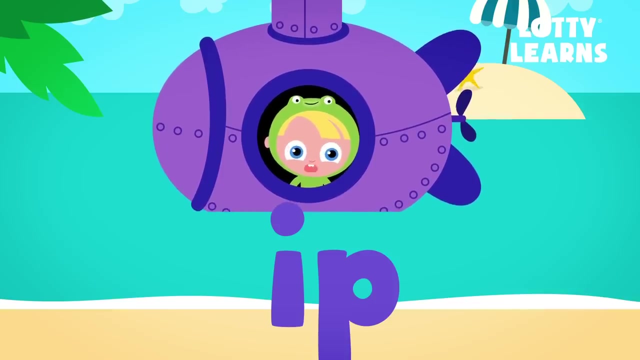 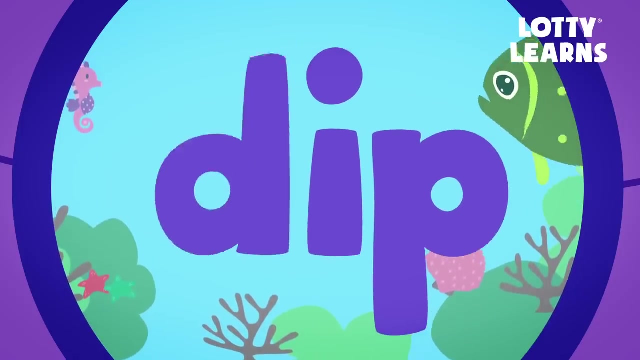 It Fit, K It Kit M It Mit Great. This says I-P, Ip. Now that we know I and P say ip, let's try and put other letters at the beginning: S, Ip, Sip. 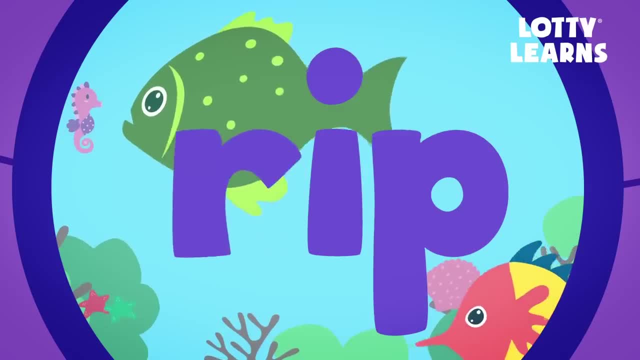 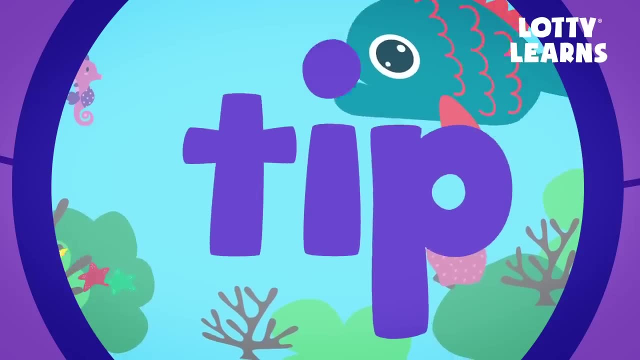 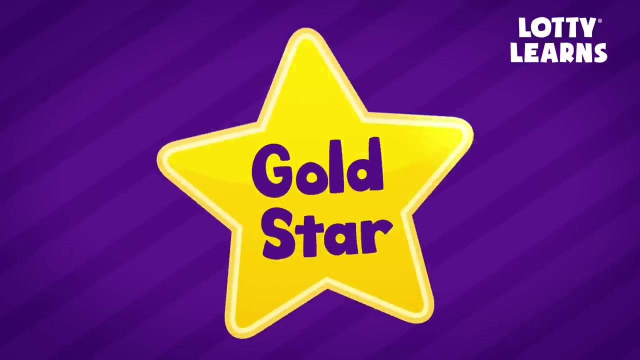 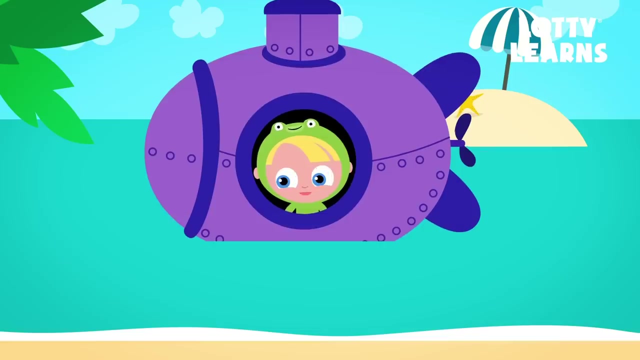 D, Ip, Dip, R, Ip, Rip H, Ip, Hip T, Ip, Tip L, Ip, Lip. Amazing Gold star. You should try the next lesson and collect even more stars. The more stars you collect, the more fun you can have. 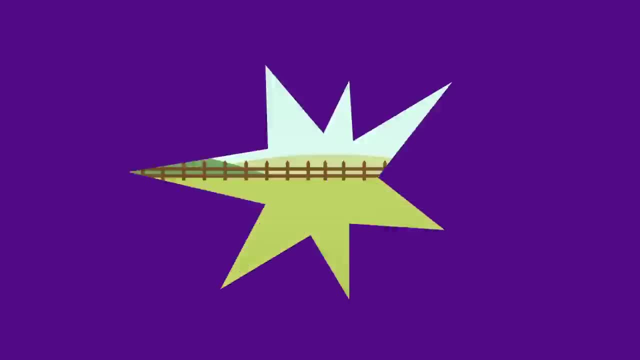 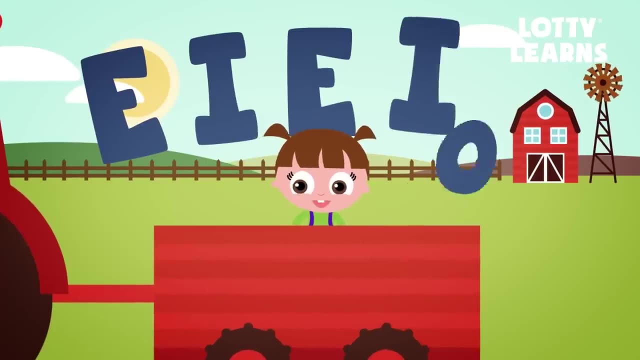 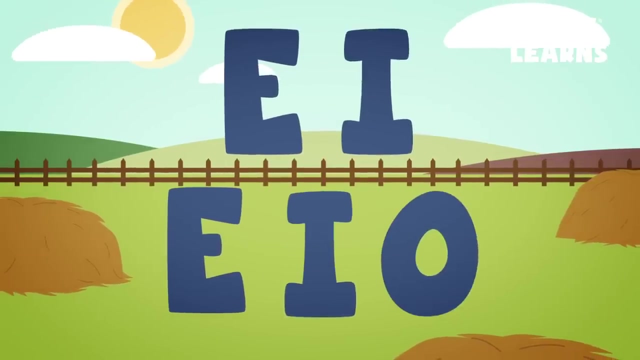 Remember to subscribe. See you next time. Old MacDonald had a farm E-I-E-I-O And on that farm he had a cow E-I-E-I-O With a moo moo here and a moo moo there. Here a moo, there a moo, everywhere a moo moo. 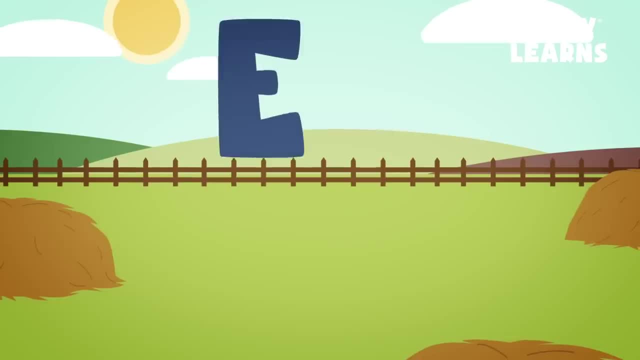 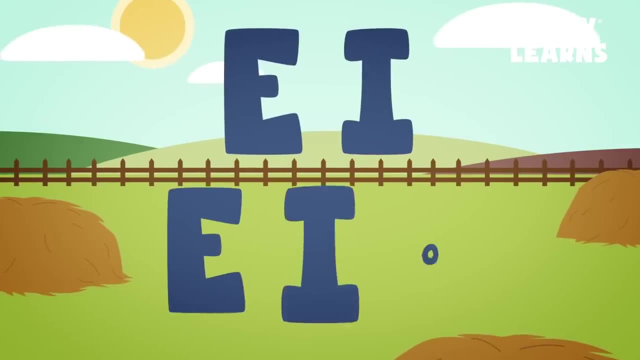 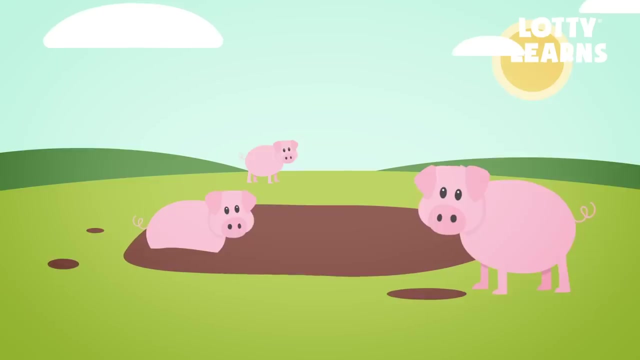 Old MacDonald had a farm E-I-E-I-O. Old MacDonald had a farm E-I-E-I-O And on that farm he had a pig E-I-E-I-O With an oink oink here and an oink oink there. Here an oink, there an oink, everywhere an oink oink. 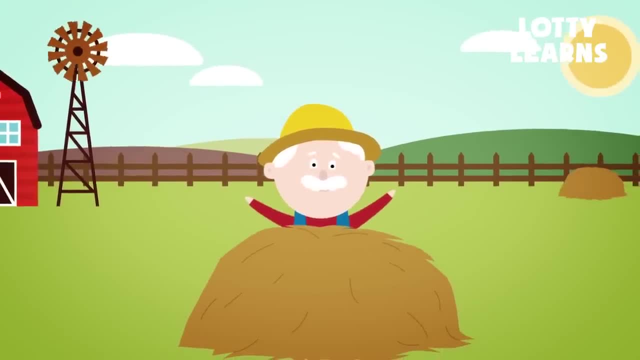 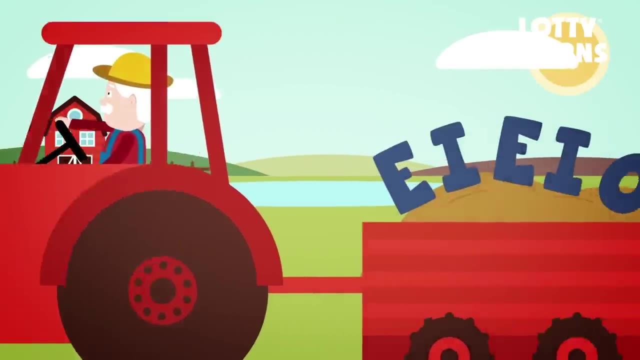 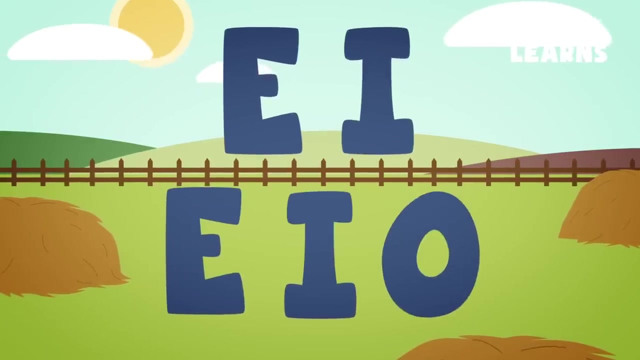 Old MacDonald had a farm E-I-E-I-O. Old MacDonald had a farm E-I-E-I-O And on that farm he had a duck E-I-E-I-O With a quack quack here and a quack quack there. Here a quack, there a quack, everywhere a quack quack. 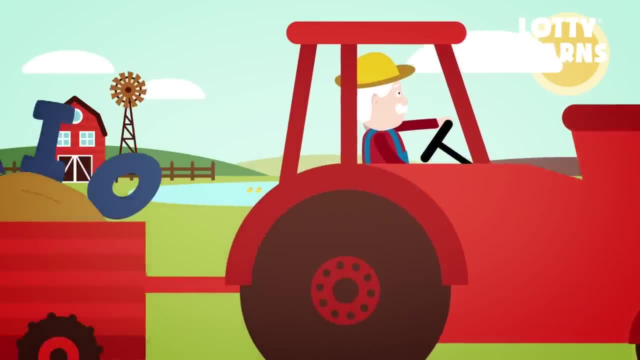 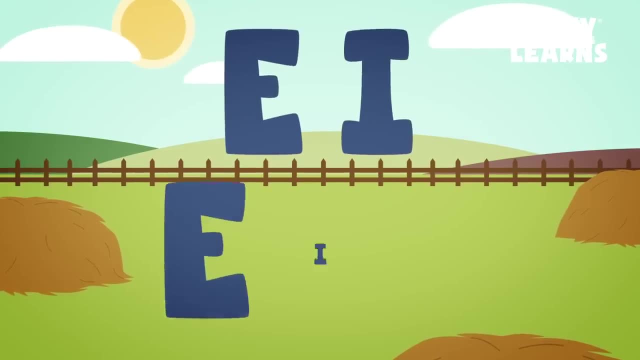 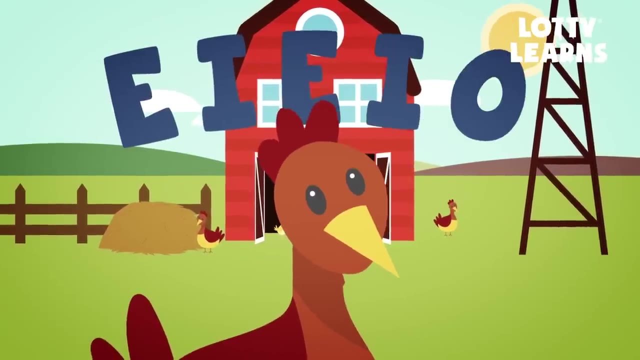 Old MacDonald had a farm E-I-E-I-O. Old MacDonald had a farm E-I-E-I-O And on that farm he had a chicken E-I-E-I-O With a cluck cluck here and a cluck cluck there. Here a cluck, there a cluck, everywhere a cluck cluck. 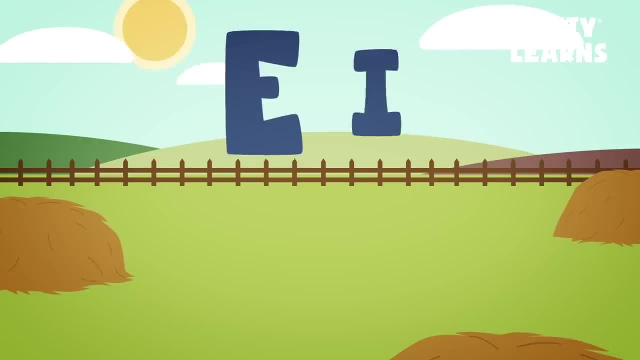 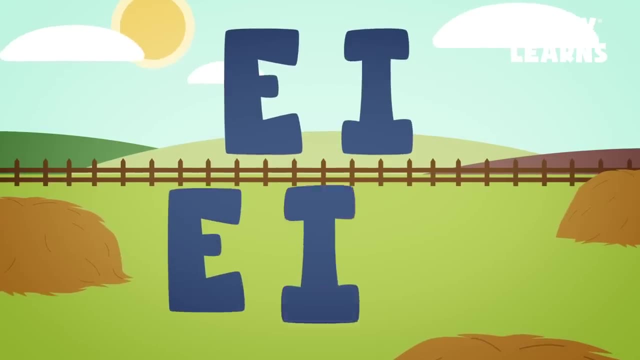 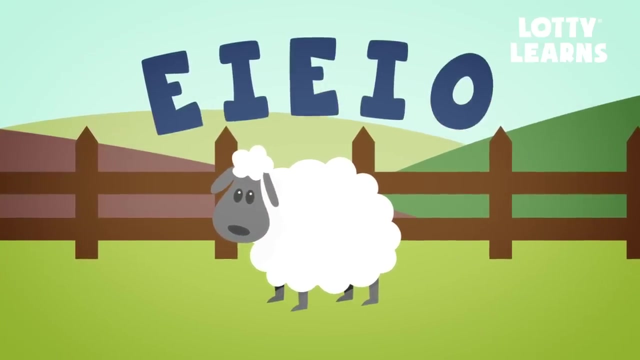 Old MacDonald had a farm E-I-E-I-O. Old MacDonald had a farm E-I-E-I-O And on that farm he had a sheep, E-I-E-I-O, With a bye, bye here and a bye bye there. Here, a bye, there, a bye, everywhere, a bye bye. 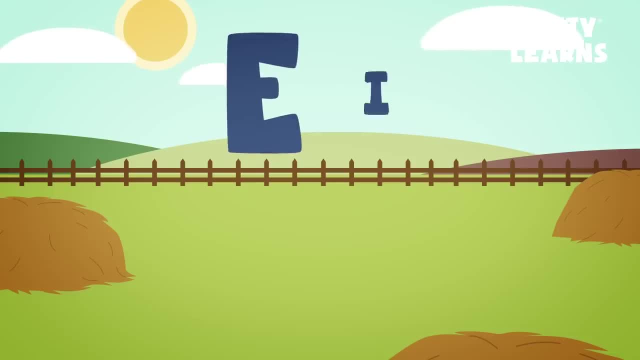 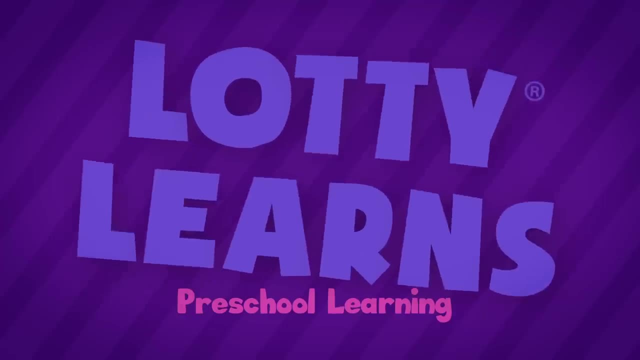 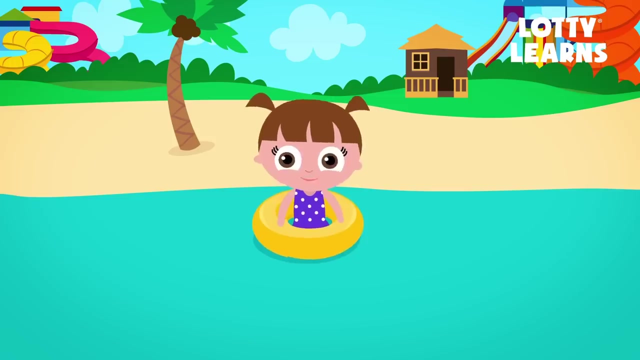 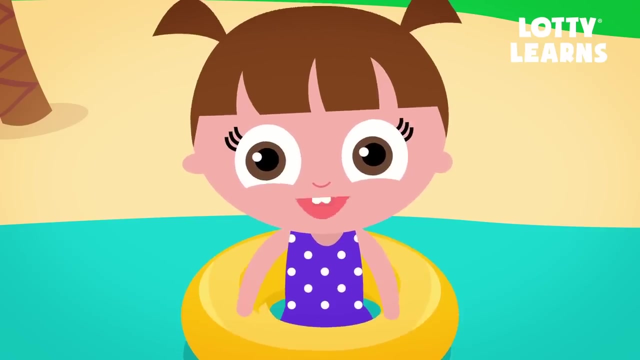 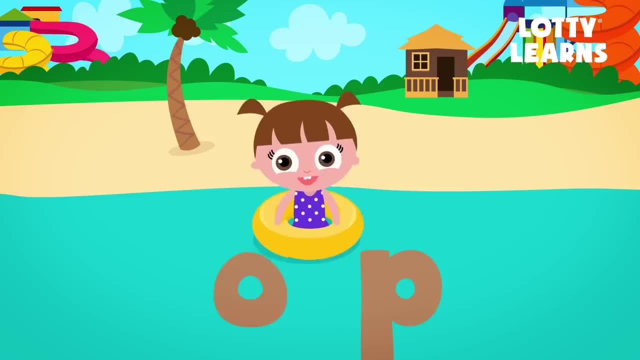 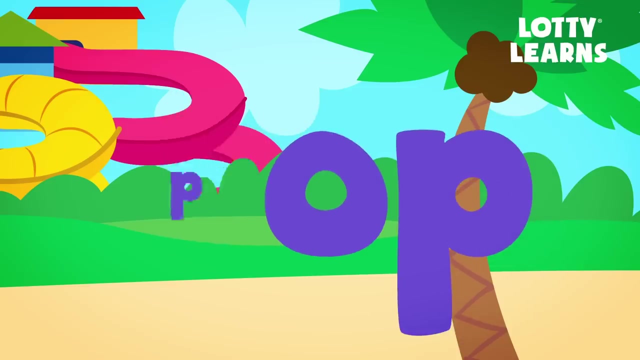 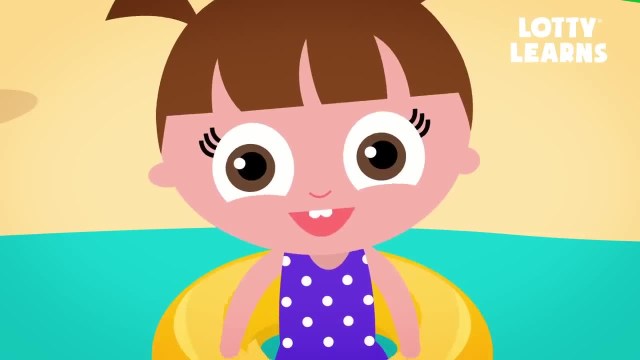 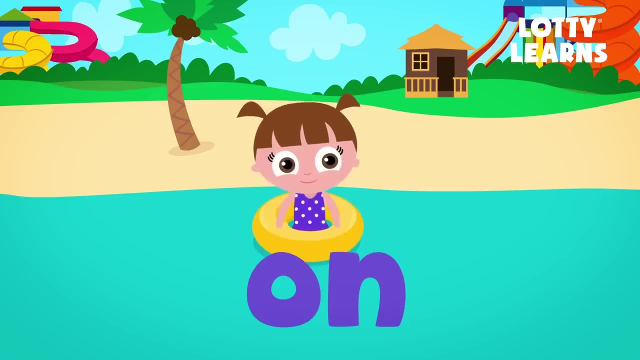 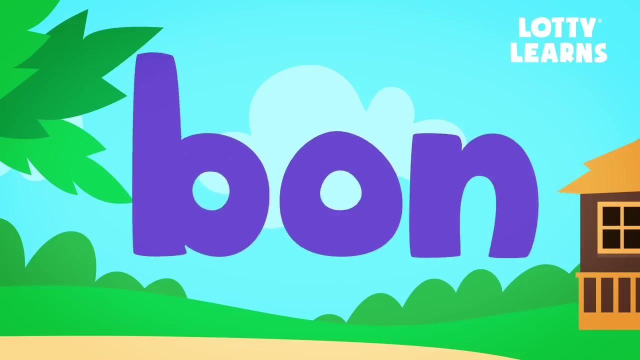 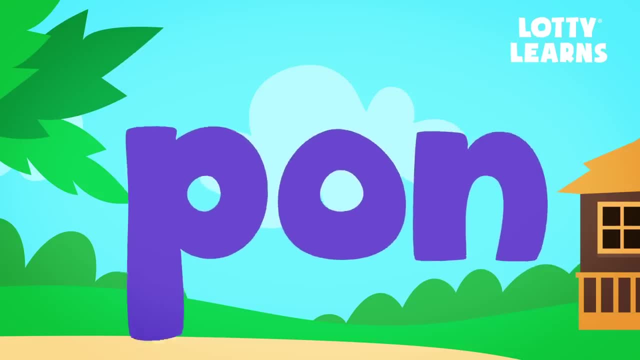 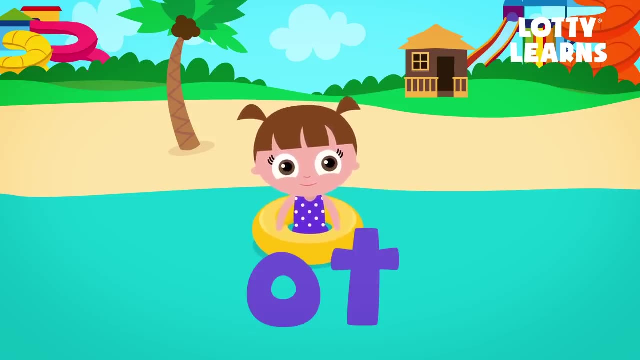 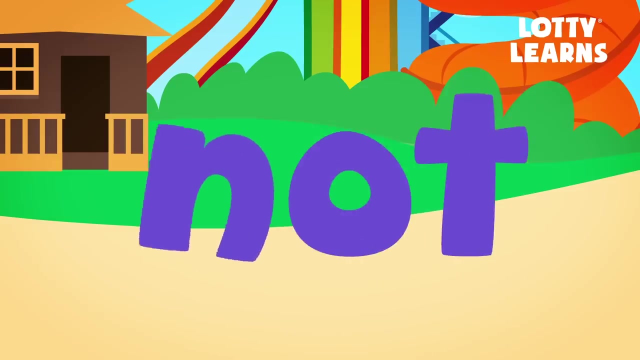 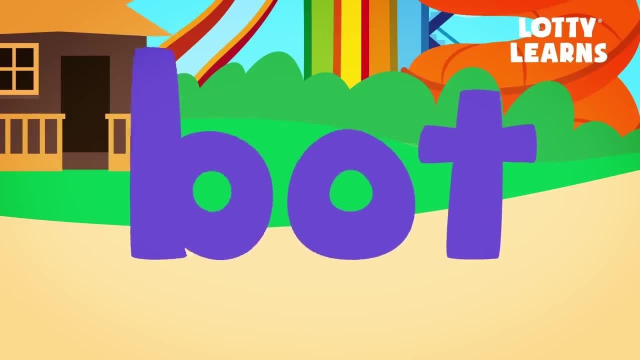 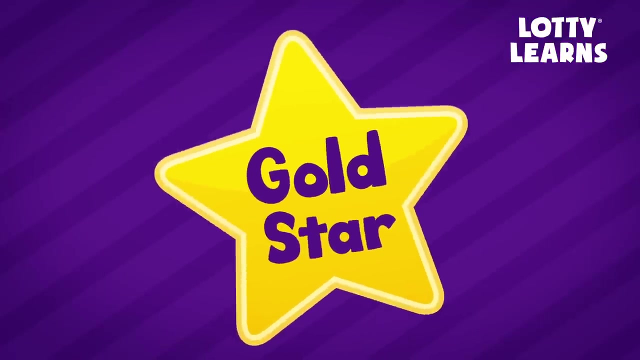 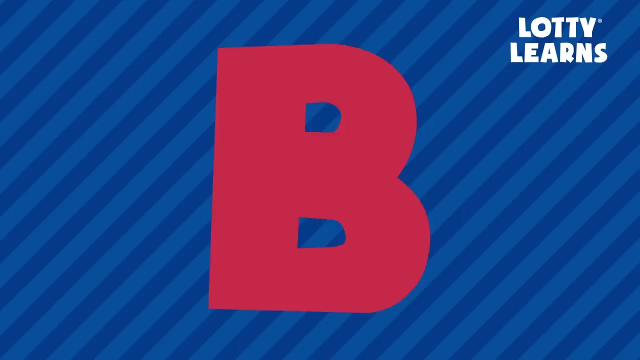 Old MacDonald had a farm. E-I-E-I-O. G Ought Got T Ought Taught H Ought Hot, Amazing Gold star. There was a farmer had a dog and Bingo was his name-o. B-I-N-G-O, B-I-N-G-O, B-I-N-G-O. 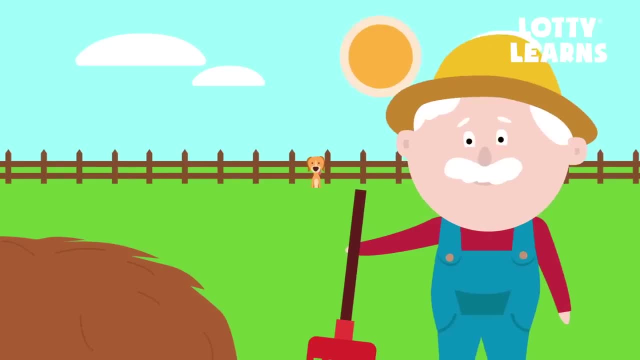 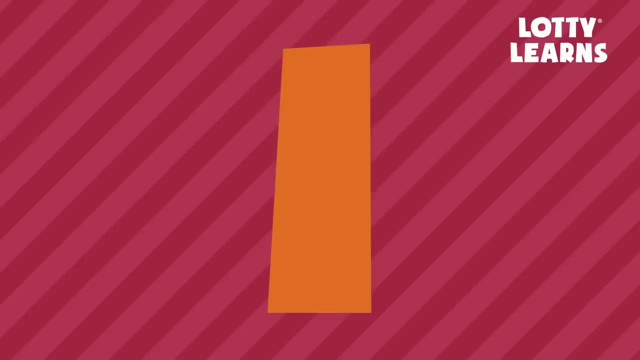 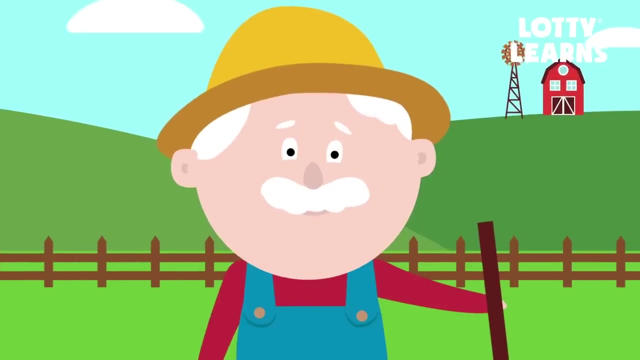 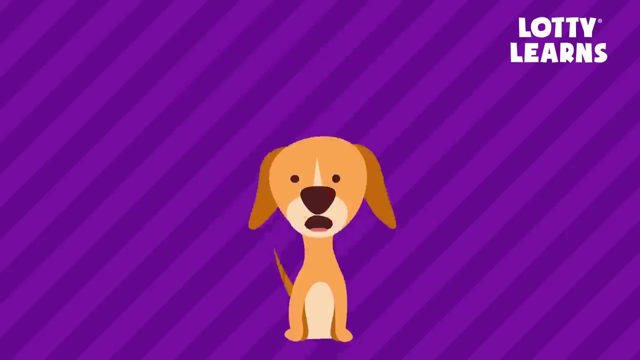 And Bingo was his name-o. There was a farmer had a dog and Bingo was his name-o. I-N-G-O, I-N-G-O, I-N-G-O, And Bingo was his name-o. There was a farmer had a dog and Bingo was his name-o. N-G-O, N-G-O, N-G-O. 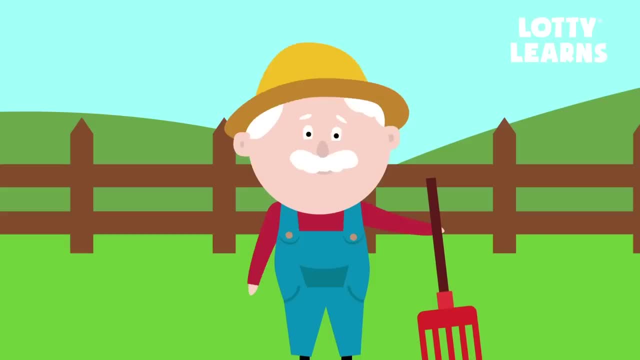 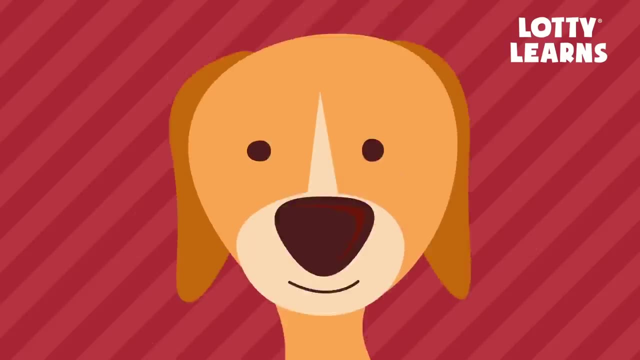 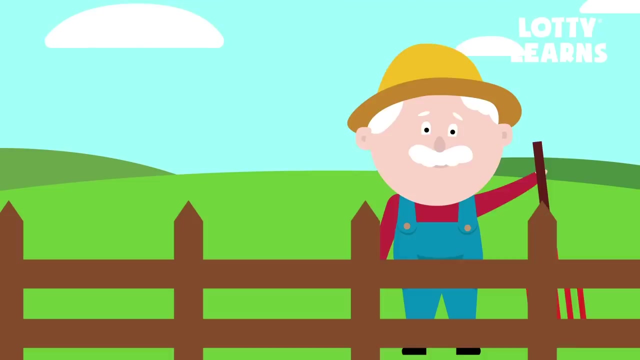 And Bingo was his name-o. There was a farmer had a dog and Bingo was his name-o. N-G-O, N-G-O, N-G-O And Bingo was his name-o. There was a farmer had a dog and Bingo was his name-o. 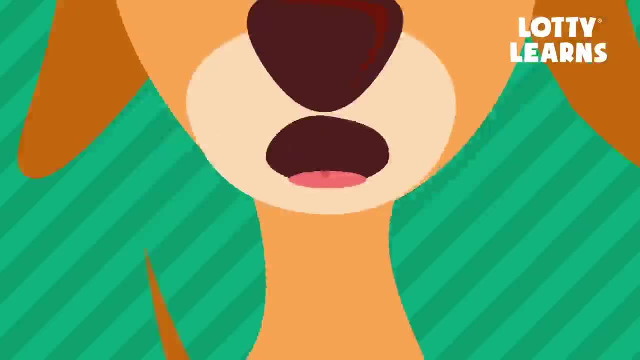 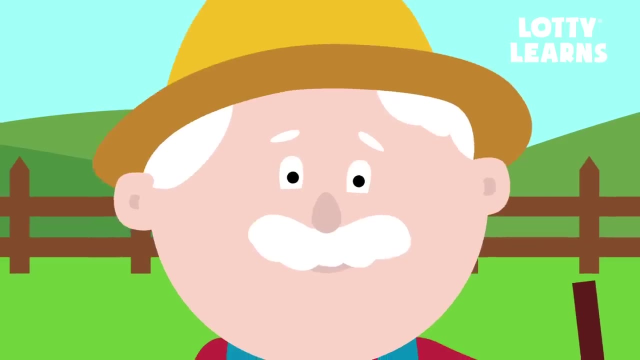 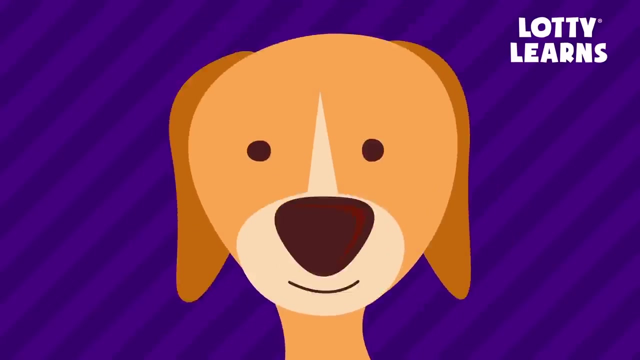 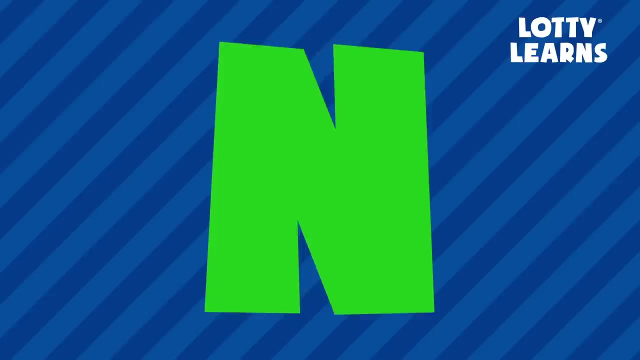 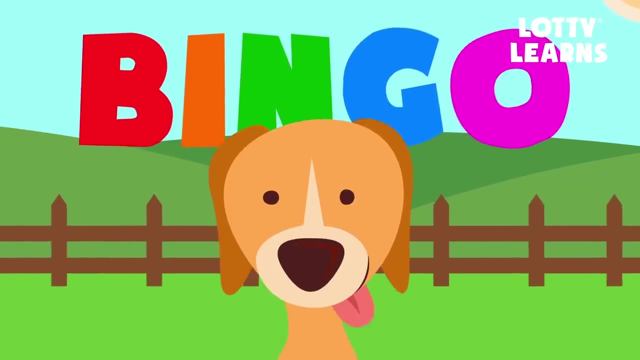 O, O-O, O, and Bingo was his name-o. There was a farmer had a dog and Bingo was his name-o. And Bingo was his name-o B-I-N-G-O, B-I-N-G-O, B-I-N-G-O, and Bingo was his name-o. 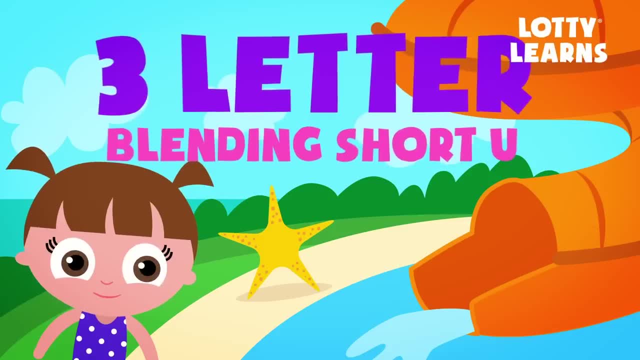 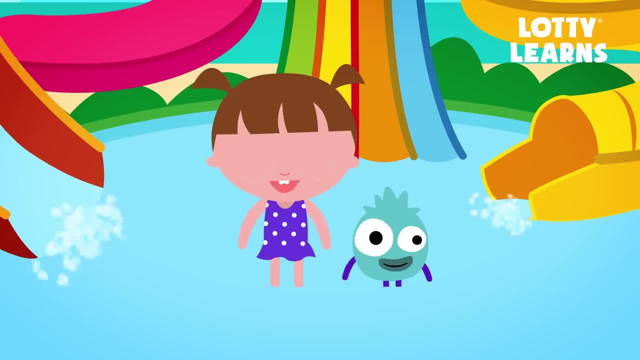 LottieLearnscom. Three-letter blending with a short U. Hi there, You've been doing such a great job. Today we're going to blend three letters together using the short U sound: uh. First we'll put two letters together, like we've done before. 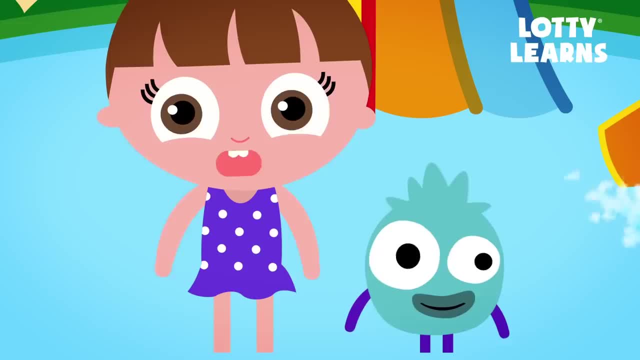 but this time we'll add one more letter to the beginning: Try and do your very best so you can win something amazing and even get to see me do something silly. Here we go. This says: uh t, uh t. 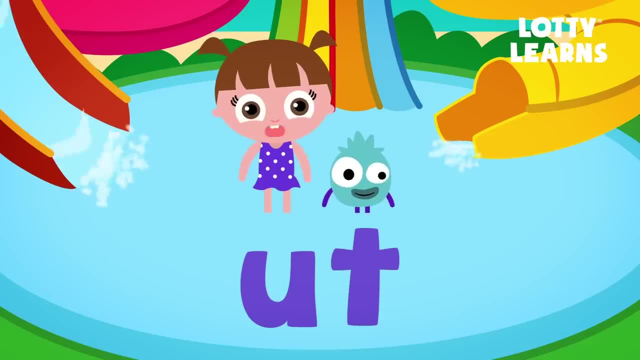 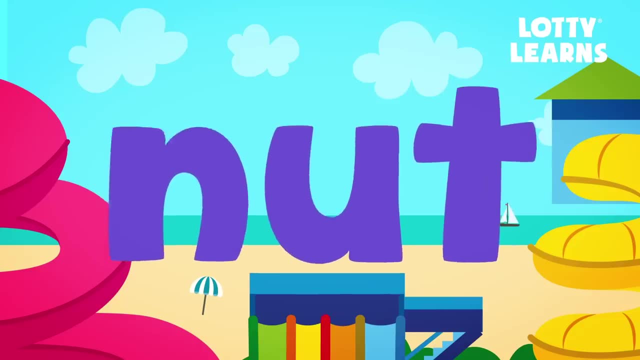 Now let's do it again. Now that we know U and T say uh-t, let's try and put other letters at the beginning: N? uh-t nut, B? uh-t butt, R uh-t rut. 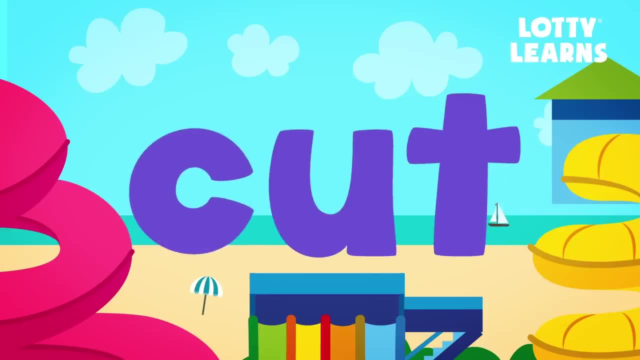 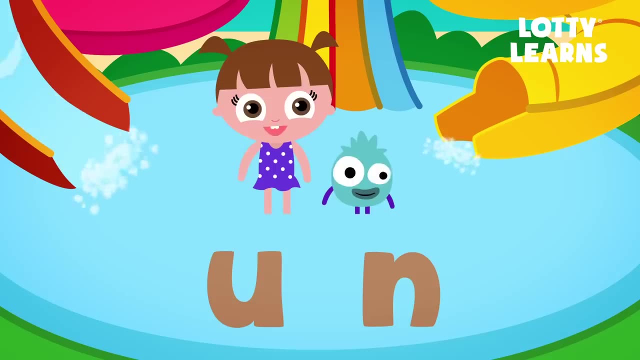 H? uh-t hut K uh-t cut M? uh-t mut. Awesome job. This says uh n. Now that we know U and N say uhn, let's try and put other letters at the beginning. 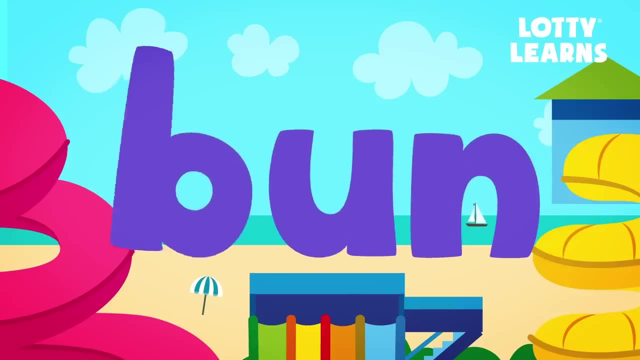 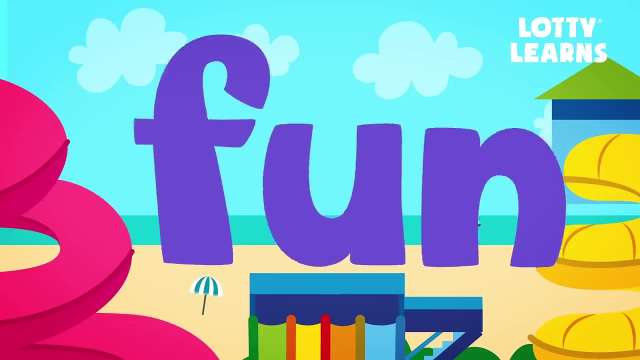 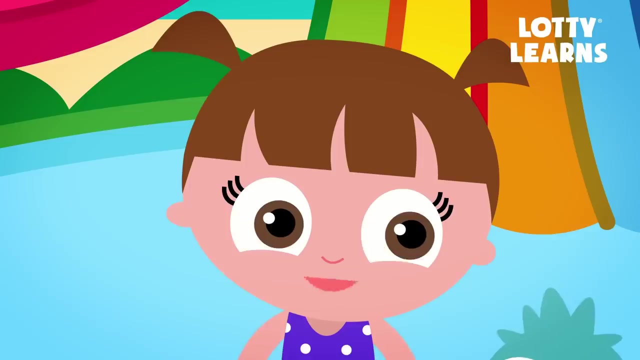 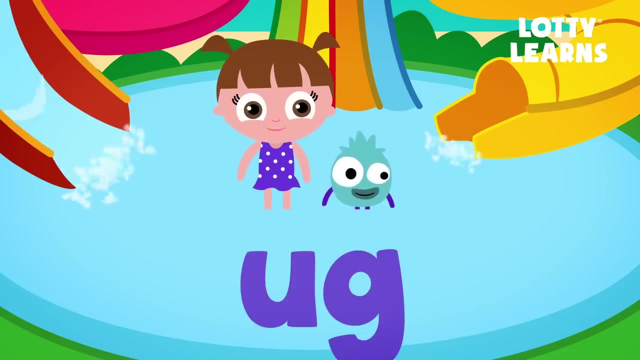 S? uh-t sun. B? uh-t fun. P? uh-t pun, Uh-t fun. R? uh-t run. H uh-t hun Great. This says uh. Now that we know U and G say ugg, let's try and put other letters at the beginning. 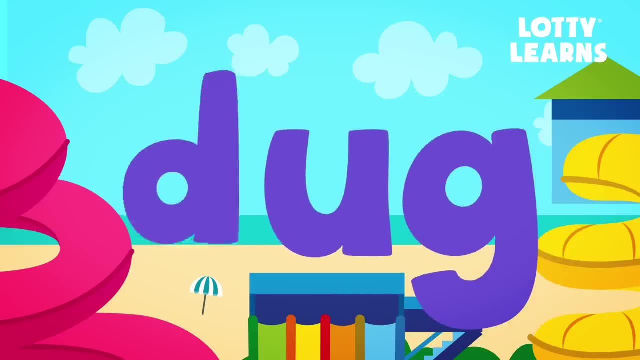 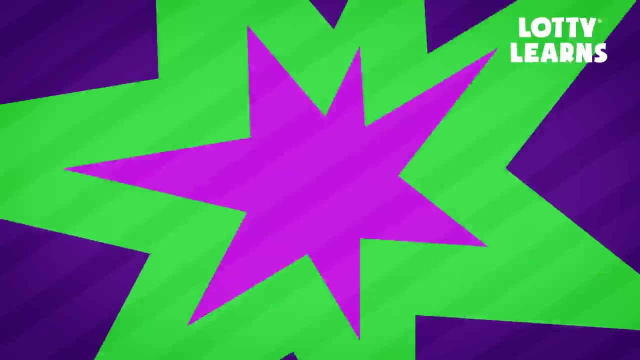 T? ugg tug, D ugg dug, B ugg bug, R ugg rug, M ugg mug, H ugg hug. Amazing Gold star. You should try the next lesson and collect even more stars. 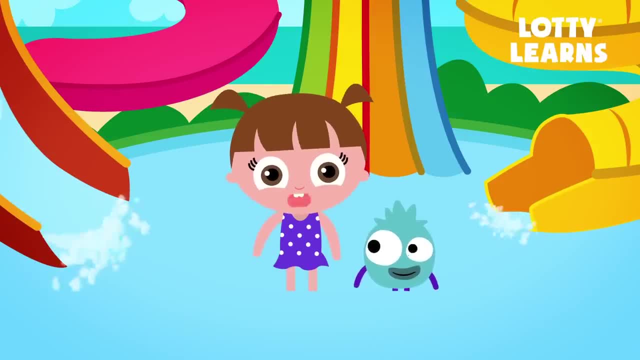 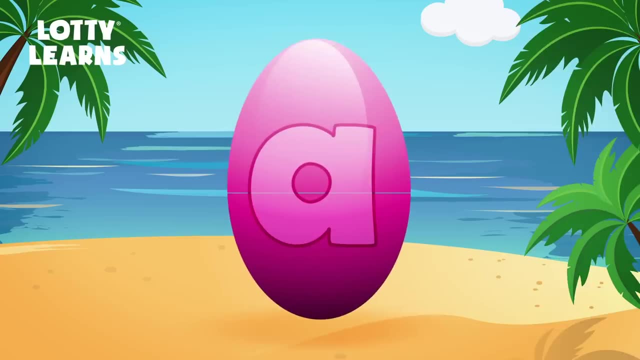 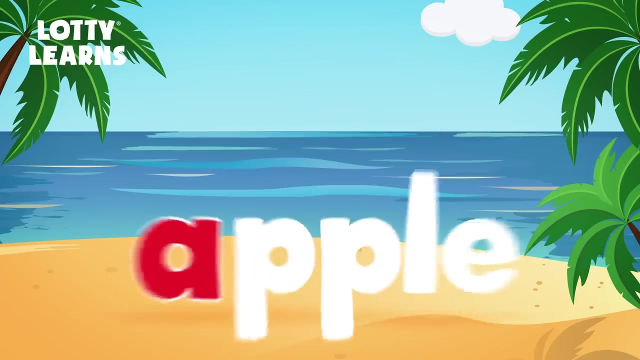 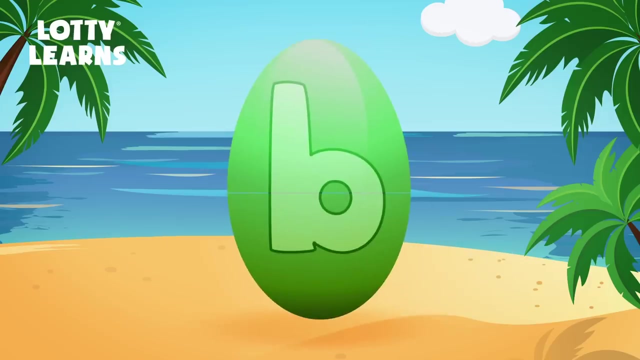 The more stars you collect, the more fun you can have. Remember to subscribe. See you next time. B buh bear. B is for bear C. cake C is for cake D, d, D, d. 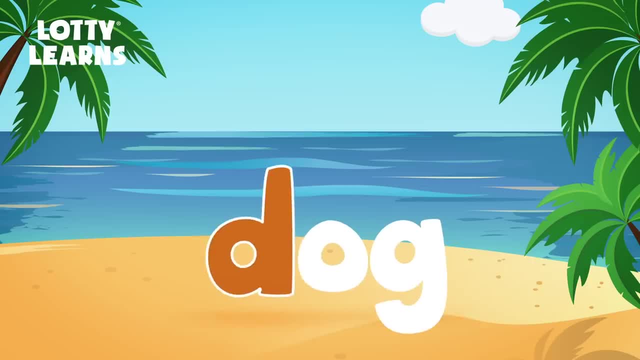 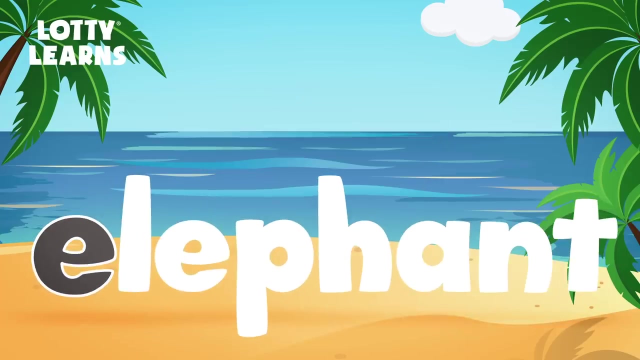 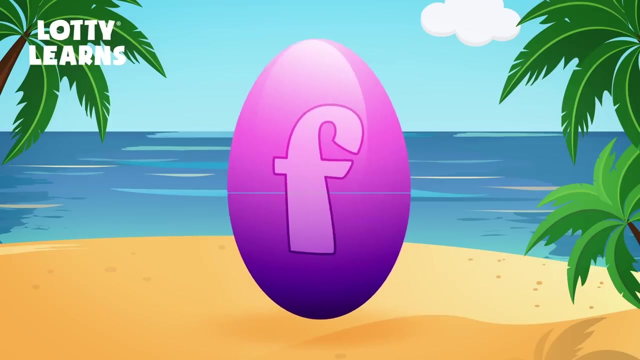 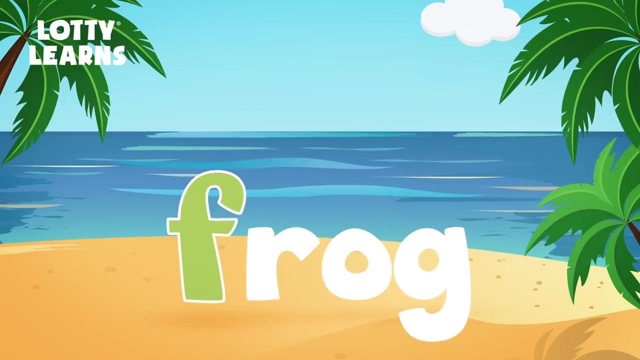 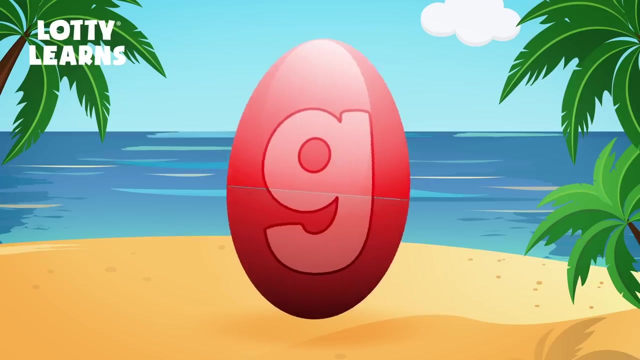 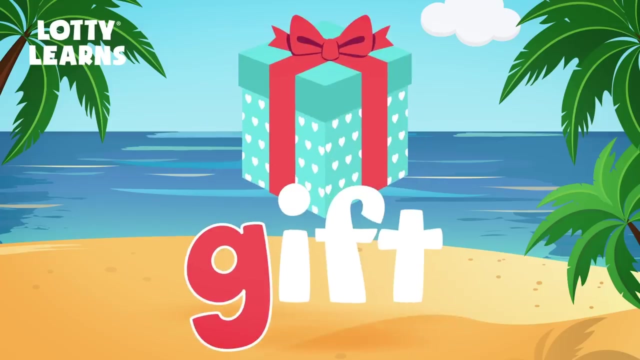 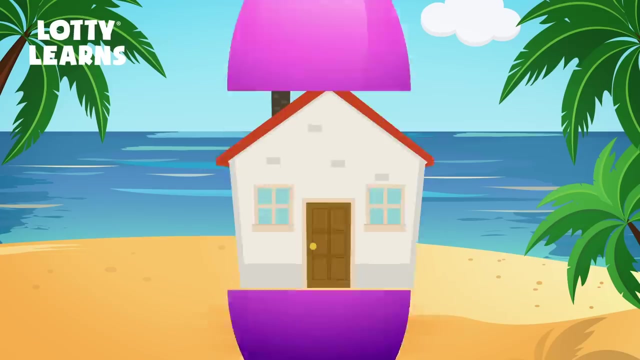 D is for dog, D is for dog E e. Elephant E is for elephant F f. Frog F is for frog G g. Gift G is for gift H h House. House. 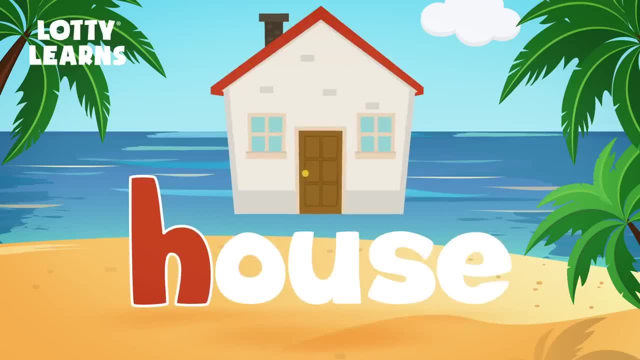 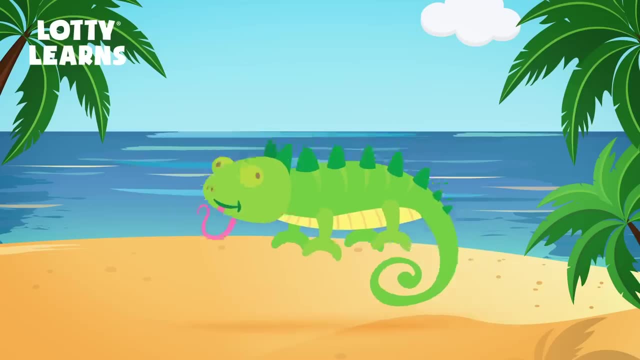 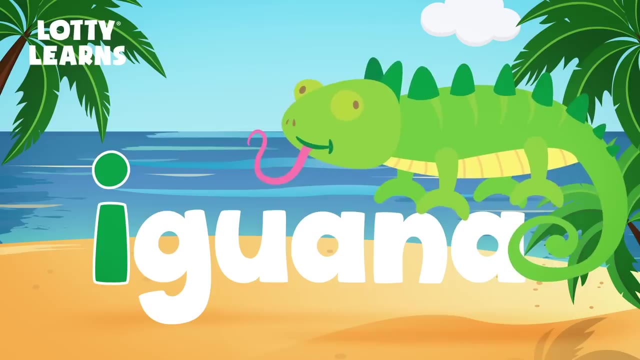 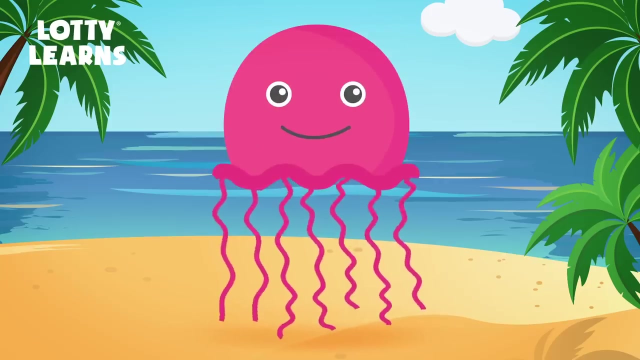 H is for house. Is is for house. I i E iguana. I is for iguana. J zh. Jellyfish. J is for jellyfish. J is for jellyfish. J zh. J is four. 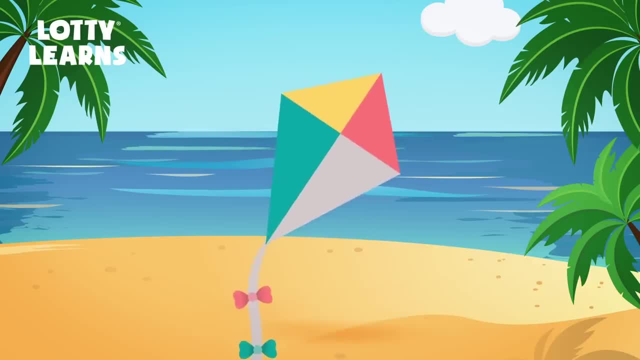 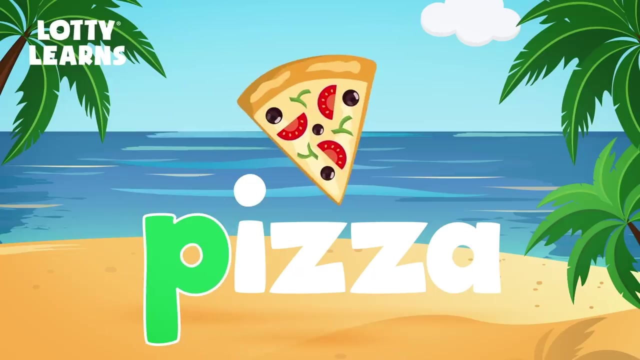 Kite K is for Kite L. Lion L is for Lion M. Monster M is for Monster N. Nose N is for Nose O I. Octopus O is for Octopus, O is for Octopus P. P. Pizza P is for Pizza Q. Queen Q is for Queen. 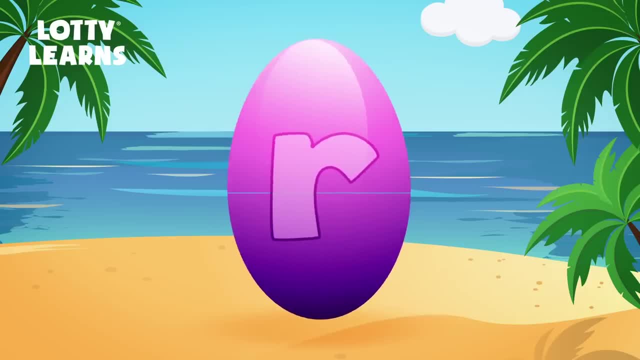 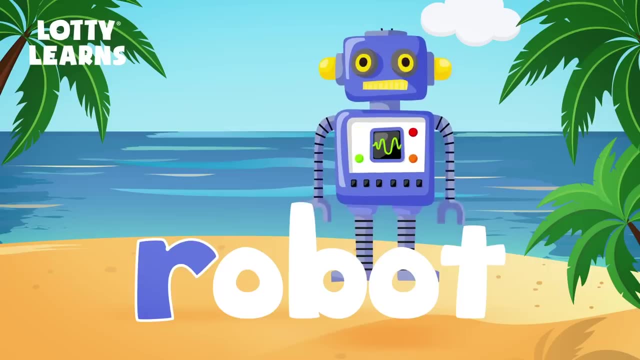 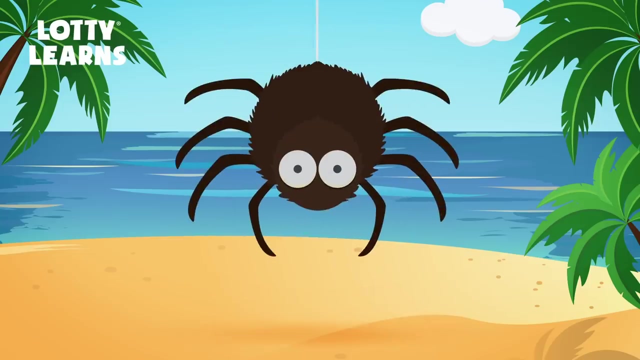 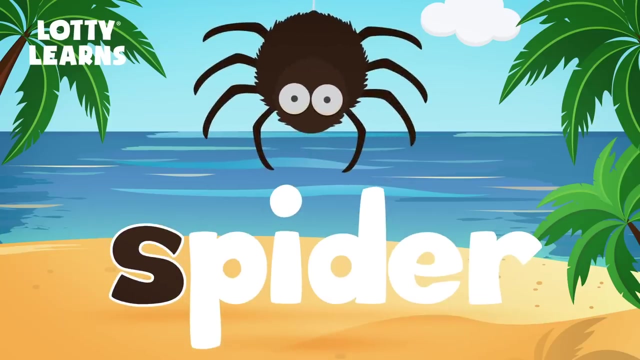 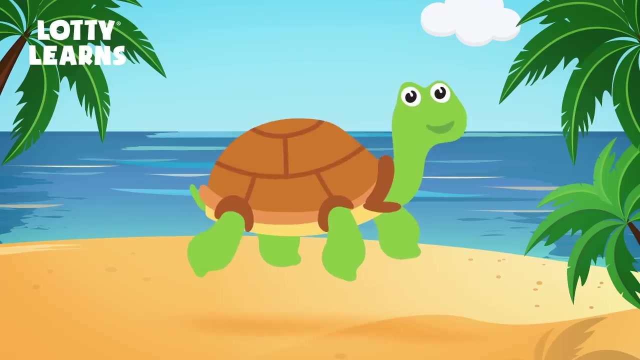 R R Robot: R is for Robot S, Spider S is for Spider T T- Turtle T- T is for T, T is for Turtle. U U Umbrella: U. U is for Umbrella, U is for Umbrella. V V- Vegetables- Vegetables- V is for VEGETABLES. 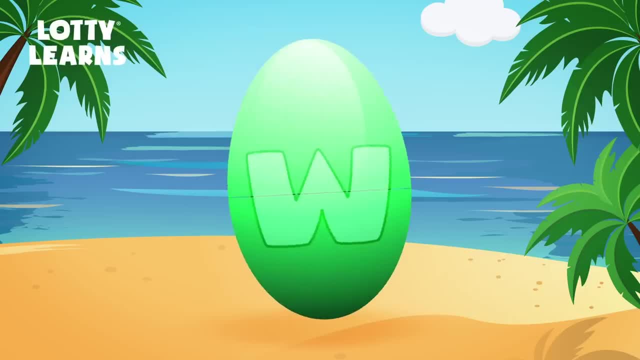 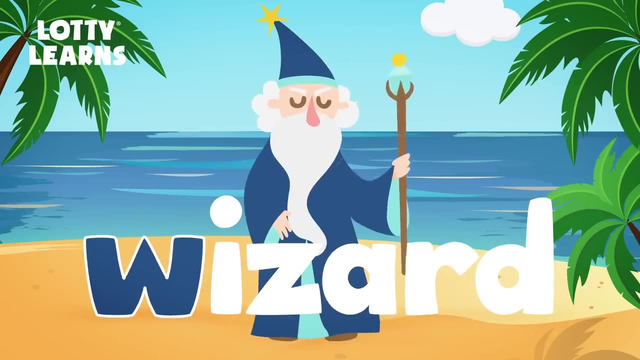 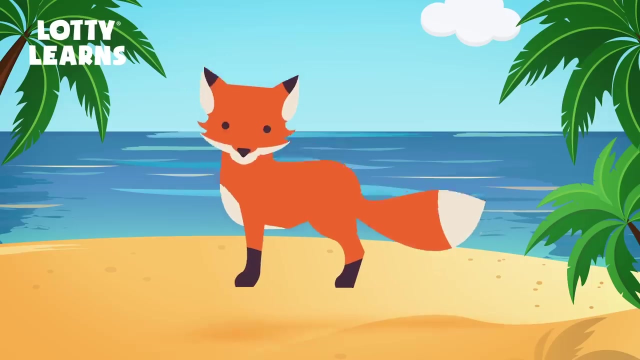 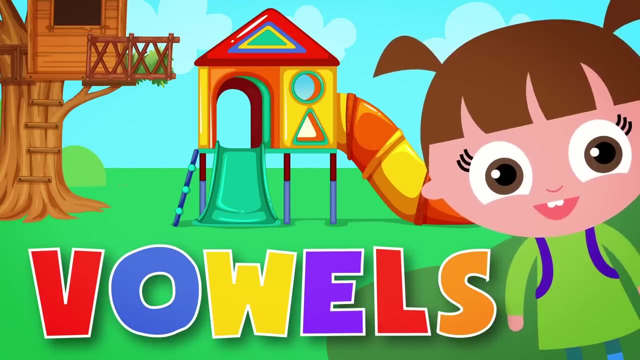 W is for WIZARD, W is for WIZARD, X is for X, FOX X is for FOX, Y is for YELLOW, Y is for YELLOW Z is for ZEBRA, Z is for ZEBRA. Vowels and Consonants. Hi there, My name is Lottie. 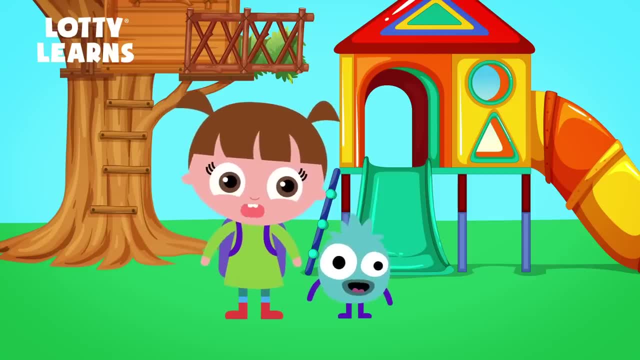 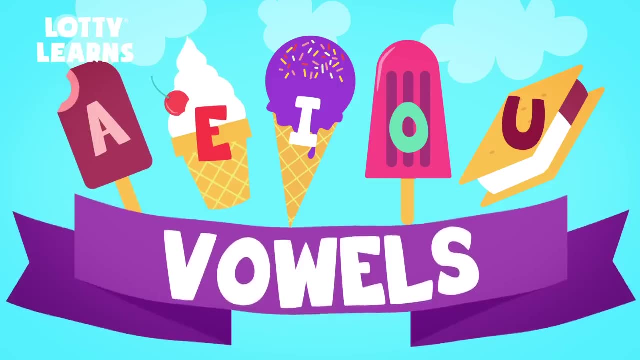 Today we're going to eat some ice cream while we learn about vowels and consonants In the alphabet. there are two different types of letters: Vowels and consonants. A, E, I, O and U are called vowels. 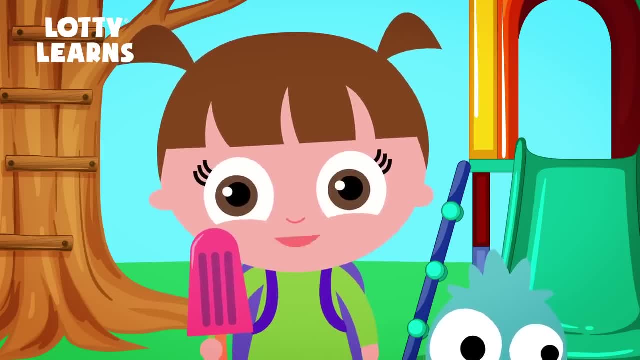 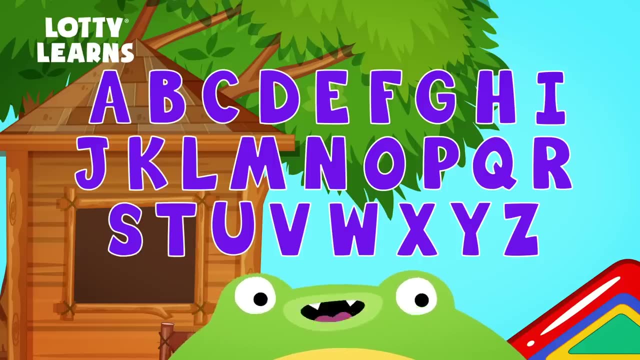 They are very special letters that can make more than one sound. Consonants are what you call all of the other letters in the alphabet. Let's look at the alphabet with me. Hi there, Do you remember which of the letters are vowels? 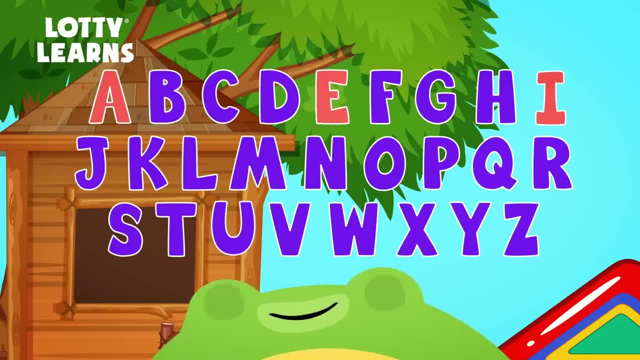 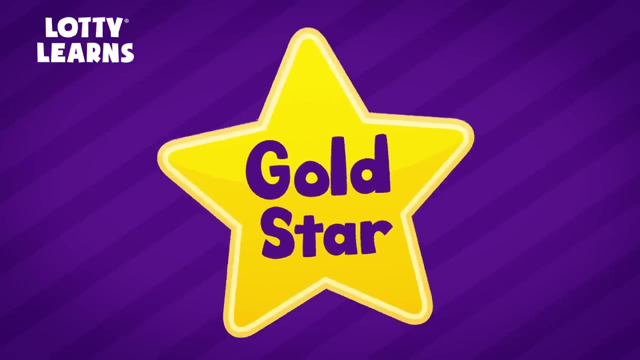 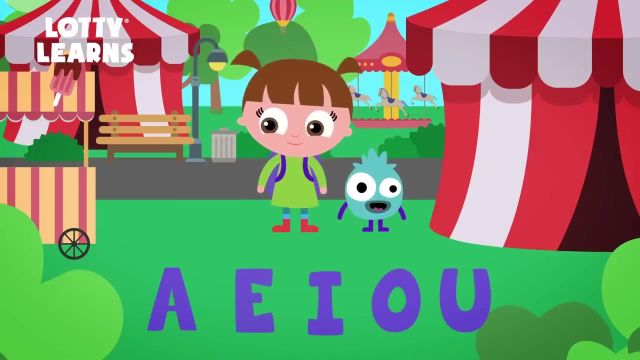 That's right: A, E, I, O and U. Now let's take out the vowels and see what's left. Great, These letters are called consonants. You're doing awesome. Gold star Learning Vowel Sounds. Do you remember the vowels from our last lesson? 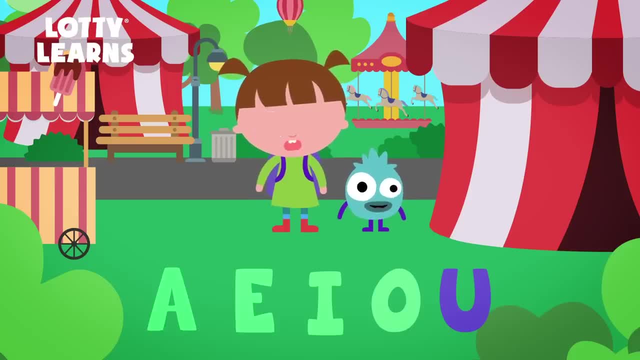 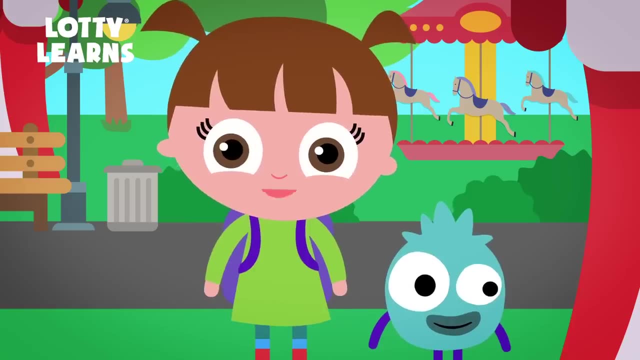 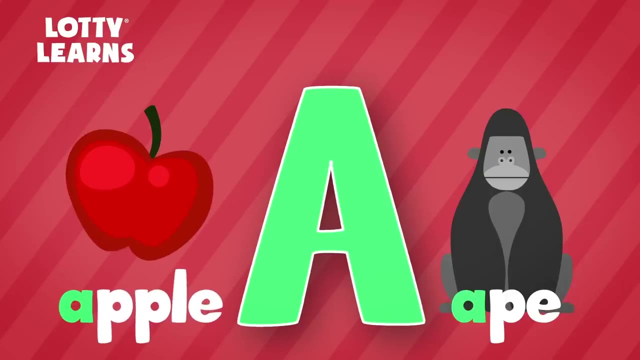 That's right: A, E, I, O, U. Well, today we're at the circus and we want to show you how these vowels can make short and long sounds. Here we go. The short A sound says like an apple. 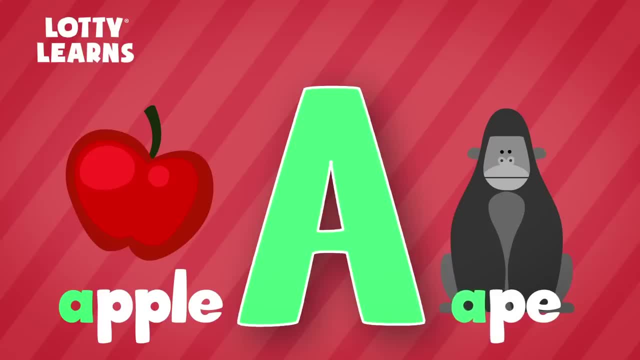 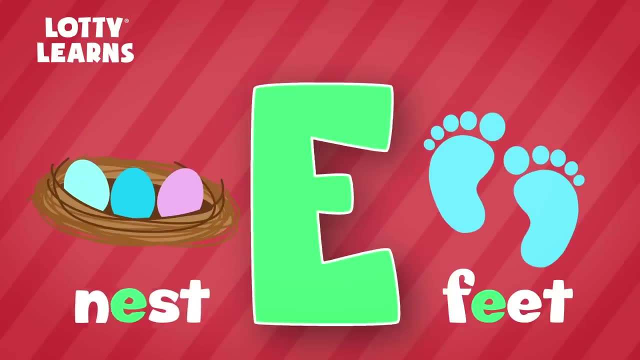 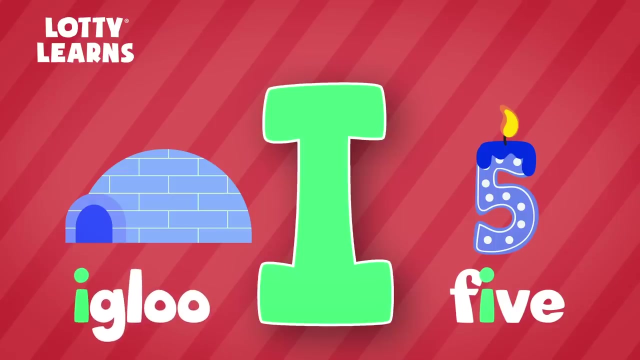 The long A sounds like its own name, like in the word eight. The short E sound says like a nest. The long E sounds like its own name, like in the word feet. The short I sound says like an igloo. The long I sounds like its own name, like in the word five. 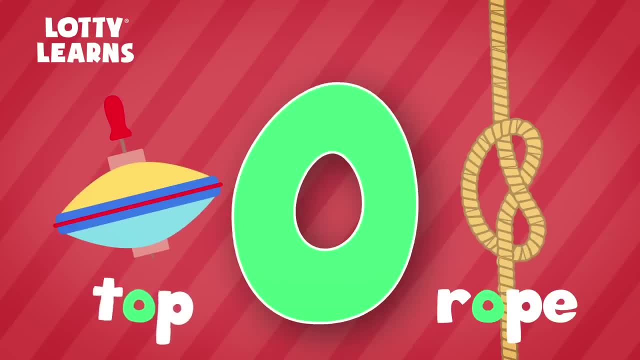 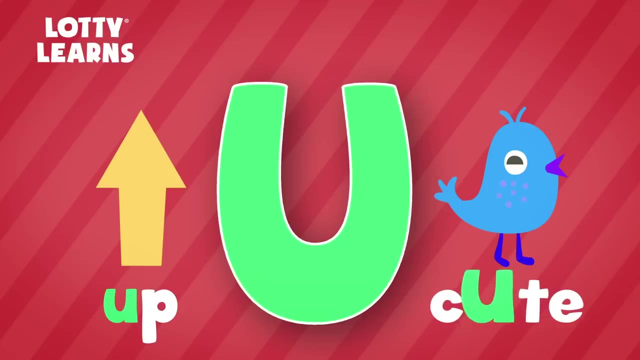 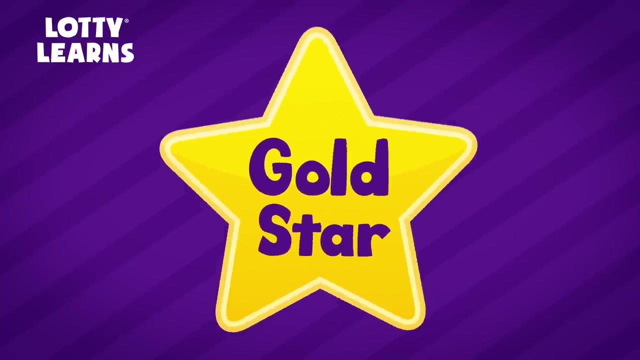 The short O sound says like in talk. The long O sounds like its own name, like in the word rope. The short U sound says like an up. The long U sounds like its own name, like in the word cute Gold star. 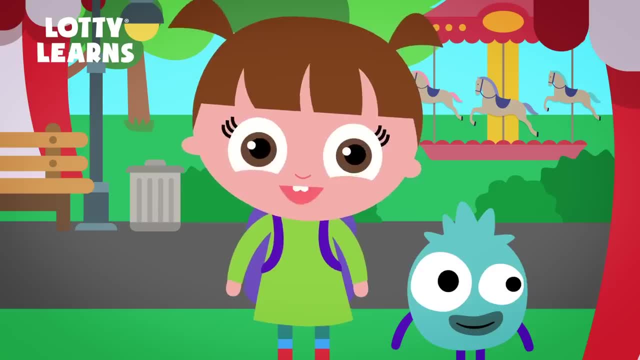 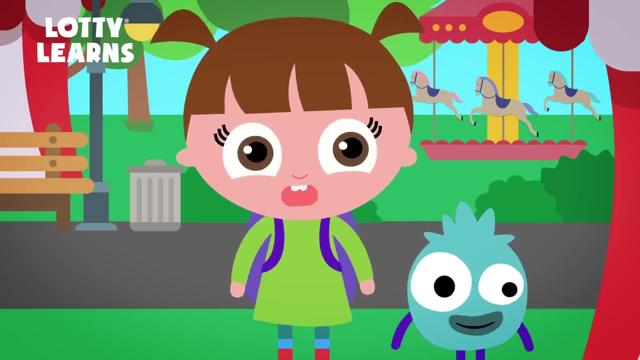 Whoa, That was awesome. I love the circus. Don't forget these vowel sounds. They're very important to remember, So watch this lesson whenever you have trouble remembering what sounds they make. Remember to practice everything you learned today with your parents. 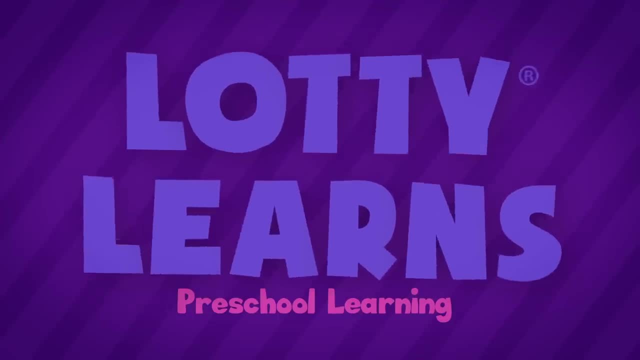 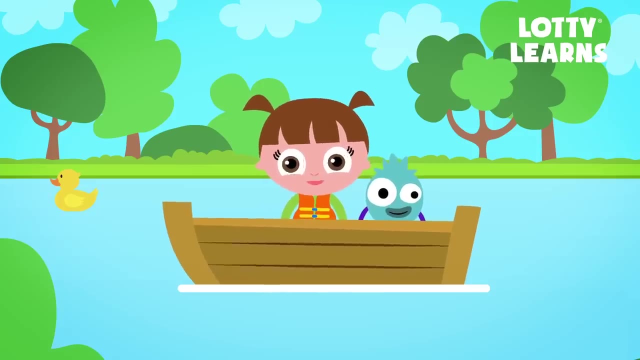 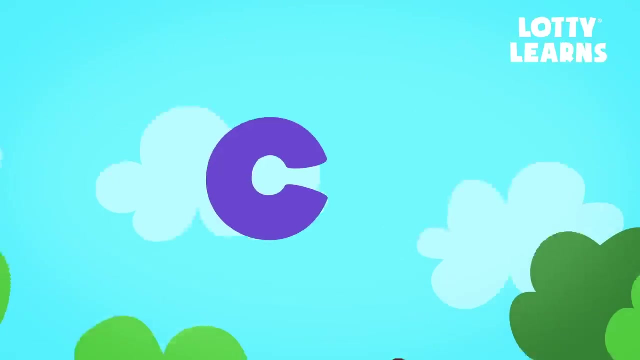 Goodbye, Hi there. My name is Lottie and this is Fuzz. Did you know that some letters like to be best friends with each other? When they're together, they make new, special sounds. Let me show you. When you see a, C and H next to each other, they make the sound ch. 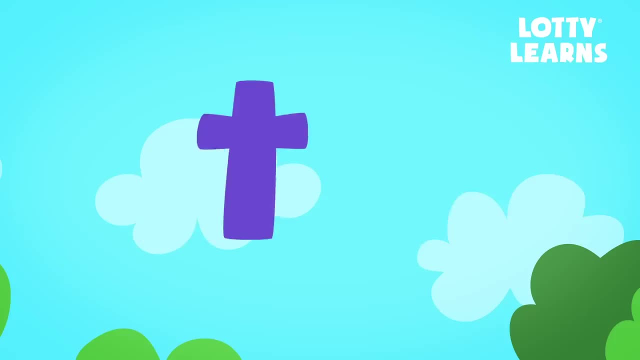 like in the word cherries. The T and H make the sound f like in the word thunder. The S and H make the sound sh like in shoe. The C and K make the sound k like in sock. The I, N and G make the sound in like in ring. 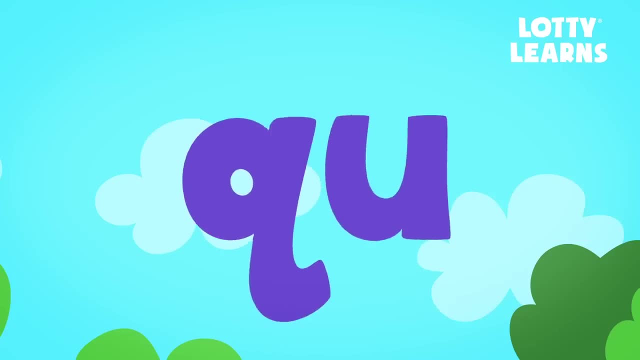 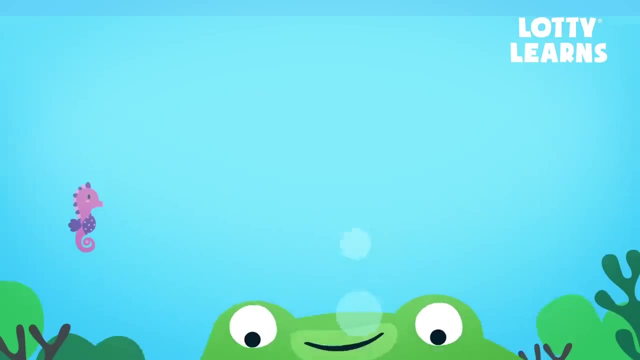 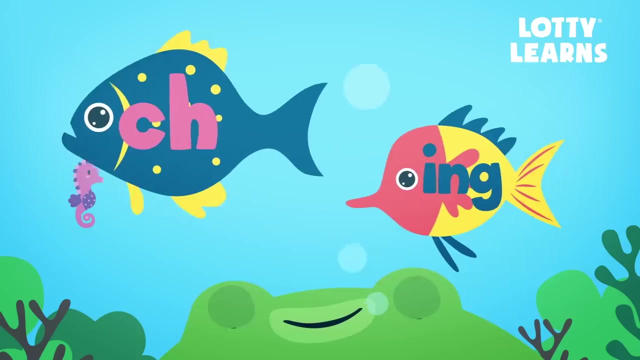 And when the Q and U are together they make the sound w Like in the word whack Great. Now let's help Chip find the special sounds. Do you remember which letters say ch, Perfect, Which letters say ing? You're doing great. 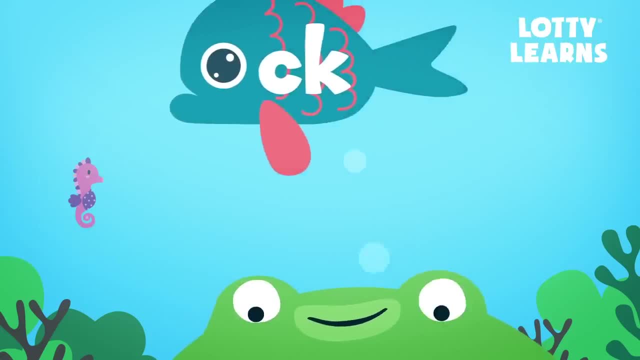 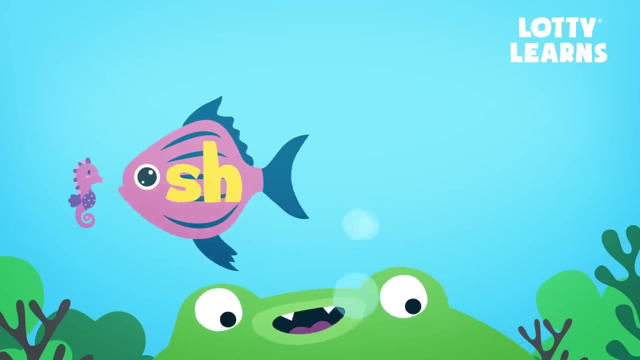 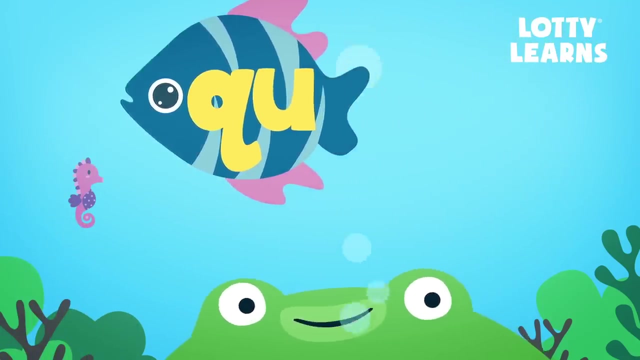 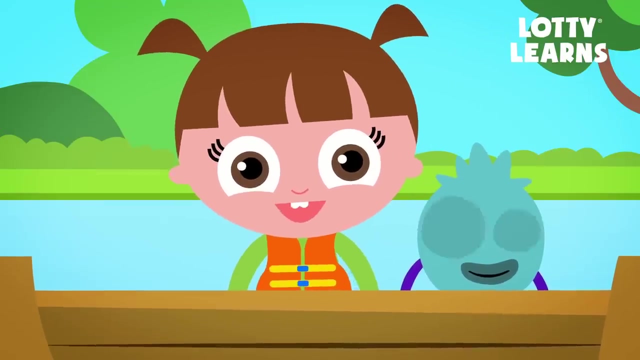 How about k- Excellent. How about sh- Cool. Which letters say f? You're doing great. And how about kwa- Amazing, That was pretty cool. Gold star, You should try the next lesson and collect even more stars. Thanks for learning with us. We had such a fun time with you. 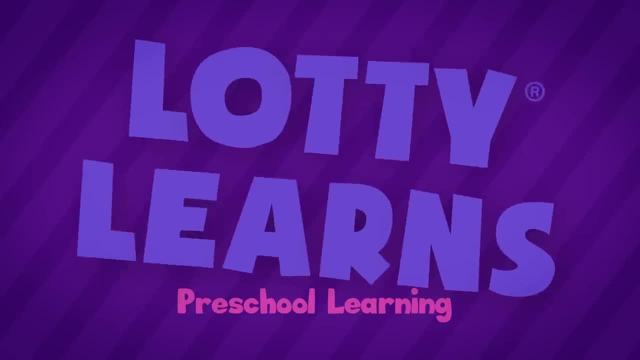 Hope you visit us again soon. LottieLearnscom Sight Words 1.. Hello friend, I'm Lottie And these are my friends Fuzz, Chuck and Chip. Today we're going to learn some new words. 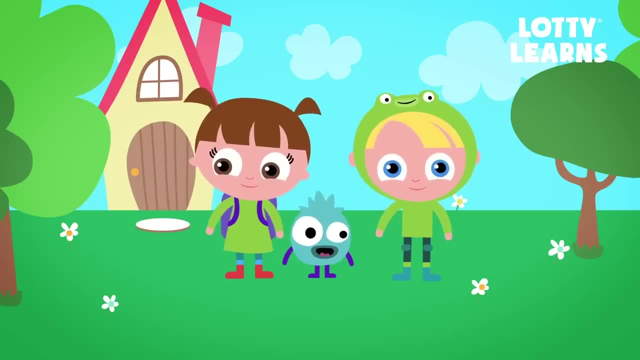 All you have to do is remember how these words look and how they sound. Say them with me. This first word is and A-N-D, And This word is we, W-E, We, This is the word: we, We. 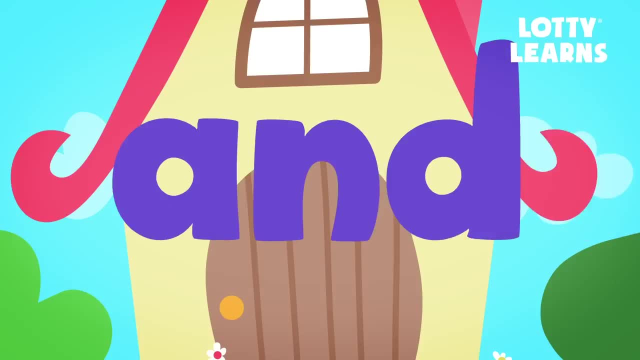 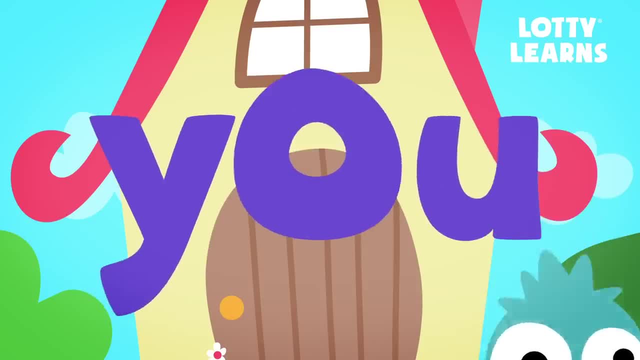 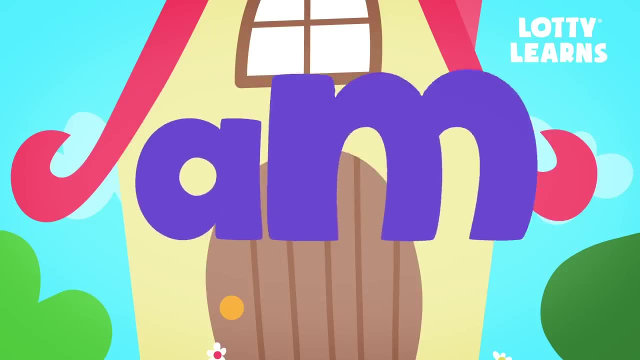 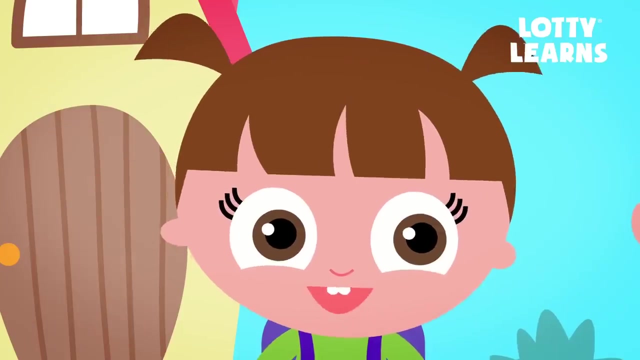 U And the last word is: am A-M? Am Gold star. It's time to review. Is there anything in my backpack that can help us? Hmmmm, What should I be looking for? Hmm, Here you go, Okay. 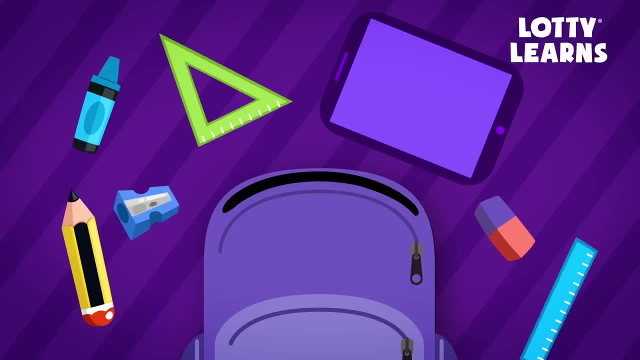 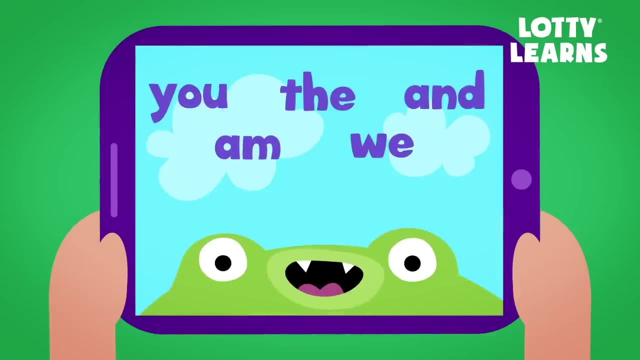 Hmm, what should we use? Awesome pick, Let's play a Lottie Learns app. Which word says you, Yep? how about and? Can you find we Great? Which word says am, And how about the? 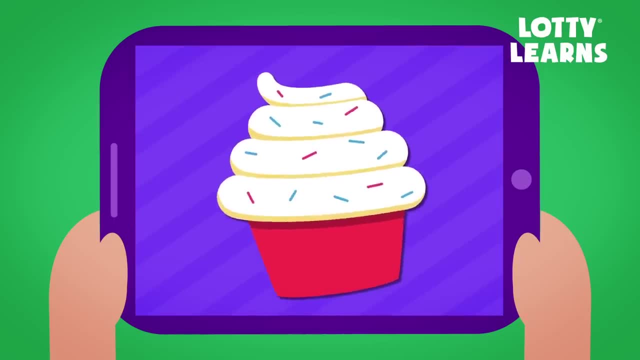 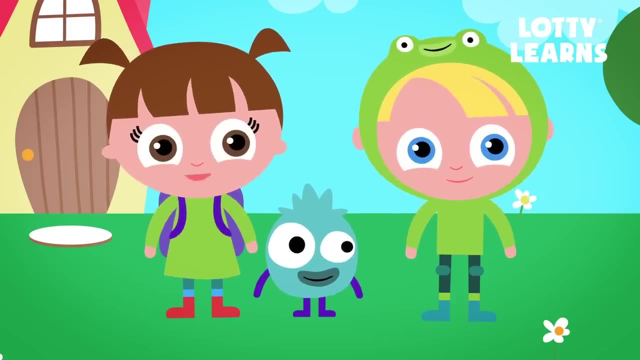 Amazing, Nice job. You just won a sticker. We had such a fun time with you. If you forget any of these words, just watch the video again to practice. See you soon, LottieLearnscom Sight words too. 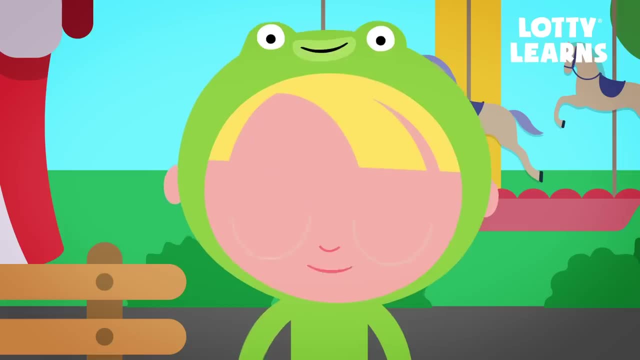 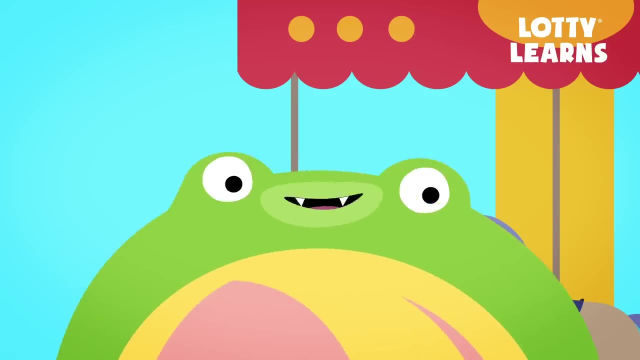 Hi there, friend. I'm Chuck and this is Chip. Hi there, Today we're going to learn a few new words. It's easy. All you have to do is remember how these words look and how they sound. Here we go. 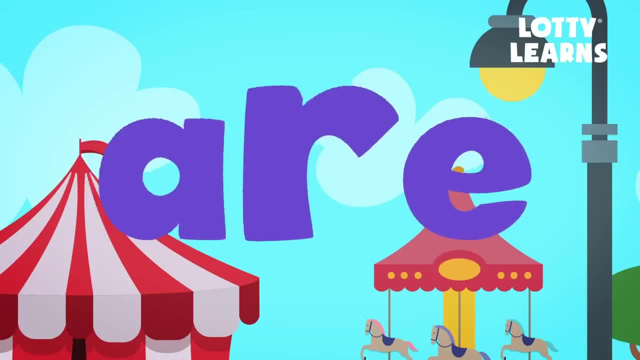 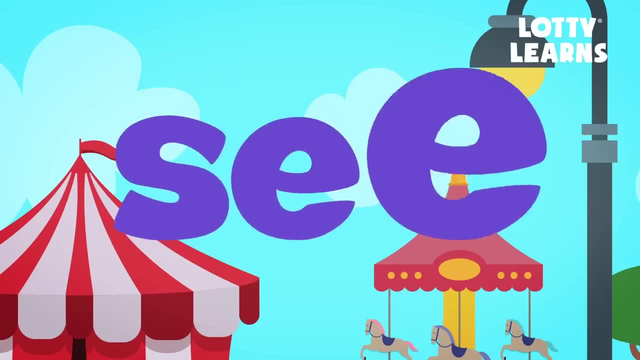 This first word is: are A R E are. This word is see S E E, See. This is the word not N O T, not. This word is with W I T H. 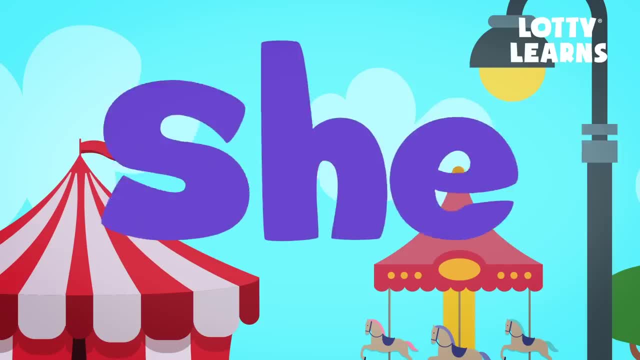 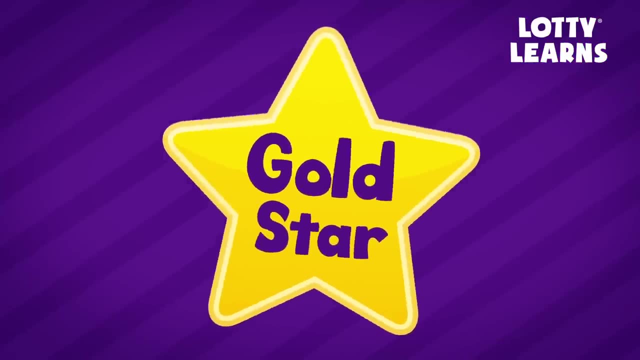 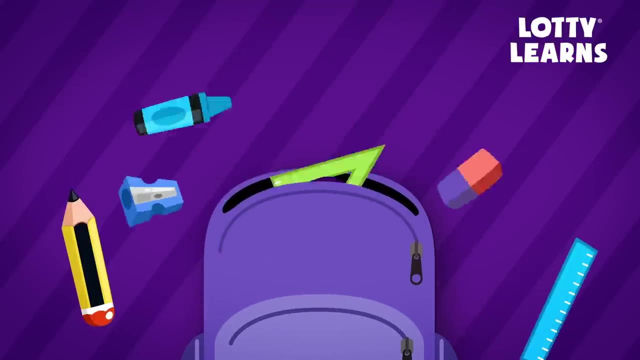 with. And the last word is she S-H-E, She Gold star. It's time to review. Is there anything in my backpack that can help us? Hmm, what should we use? Awesome pick, Let's play a game. 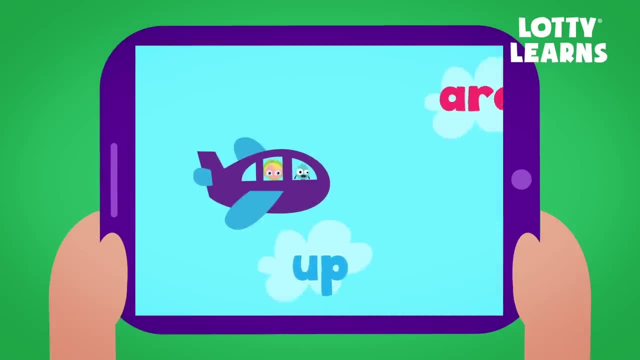 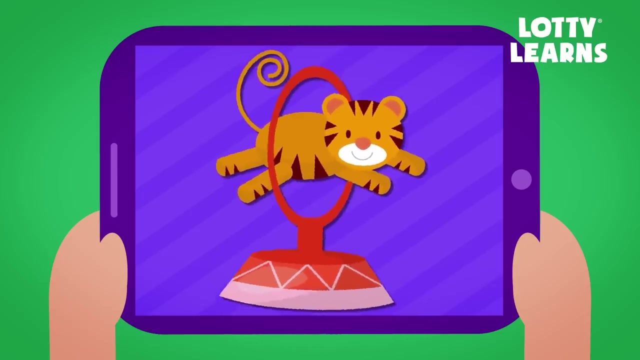 Which word says R? Yep, How about she? Can you find not Great? Which word says C? And how about? with Amazing, Nice job, You just won a sticker. We had such a fun time with you, If you forget. 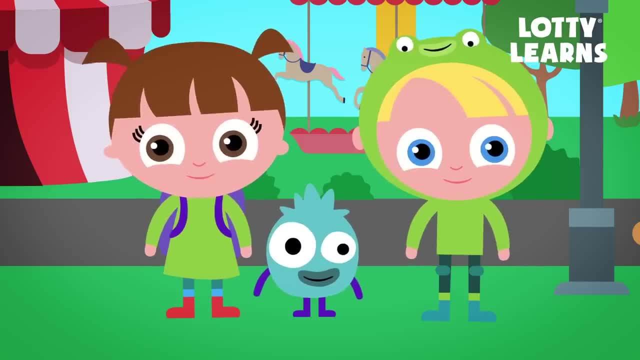 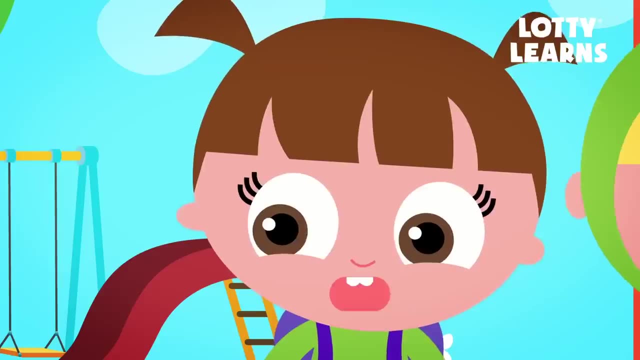 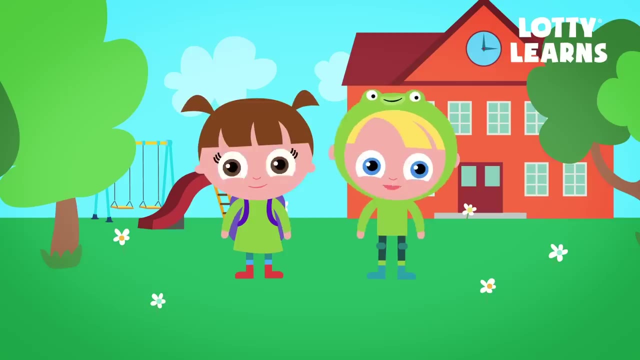 any of these words. just watch the video again to practice. See you soon. LottieLearnscom Sight- Words 3.. Hello friend, I'm Lottie and today we're going to learn a few new words. All you have to do is remember how to say them. 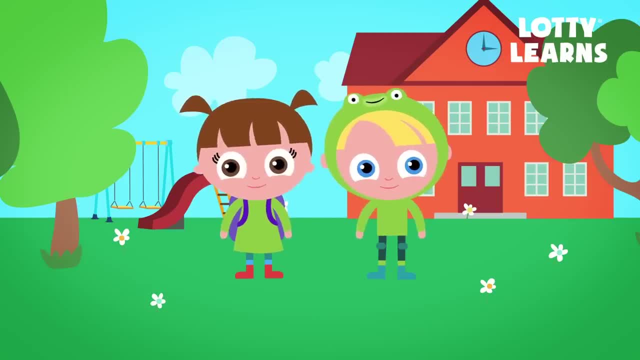 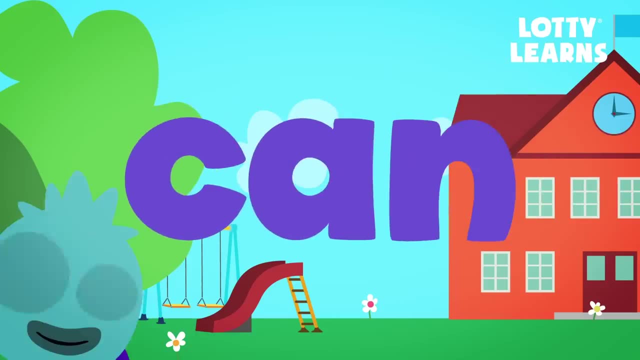 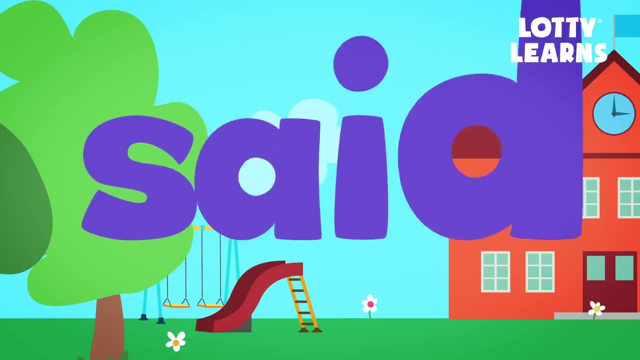 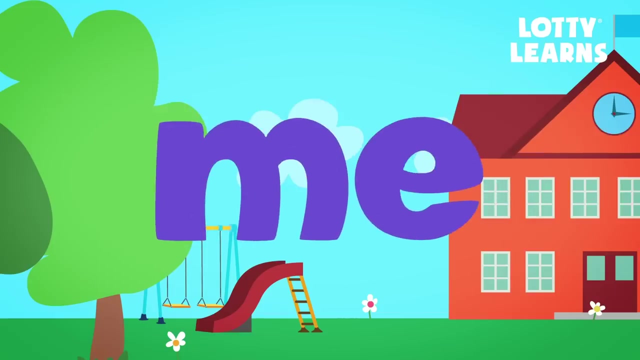 Say them with me. Here we go. This first word is can, C-A-N, Can. This word is said S-A-I-D Said. This is the word: me, M-E, Me. This word is got G-O-T, Got, Got, Got, Got. 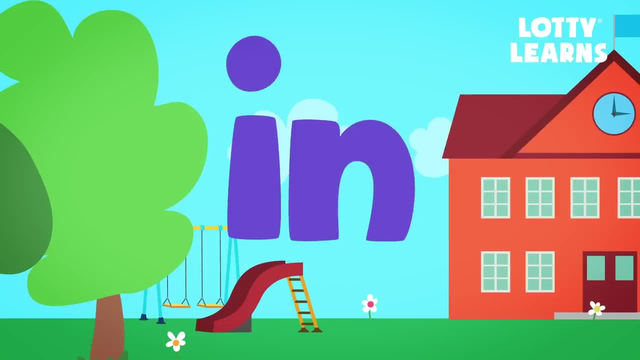 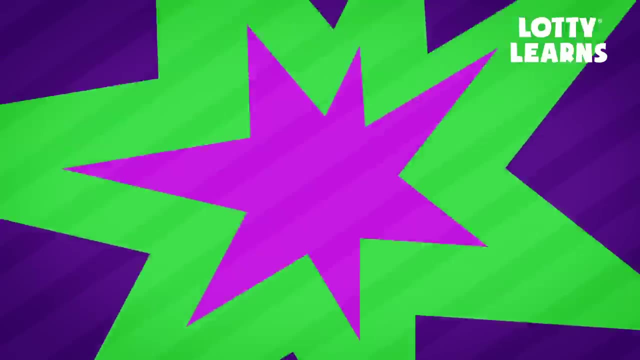 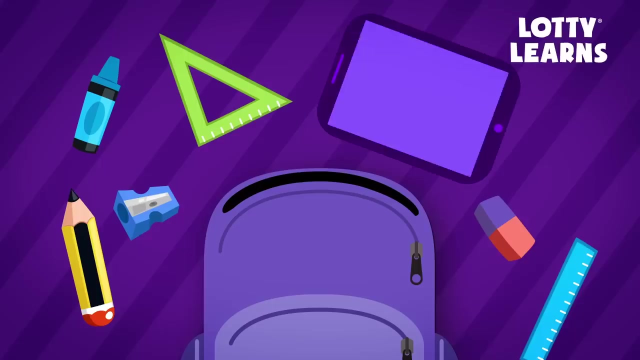 And the last word is in I-N In Gold star. It's time to review. Is there anything in my backpack that can help us? Hmm, What should we use? Awesome pick, Let's play a Lottie Learns app. 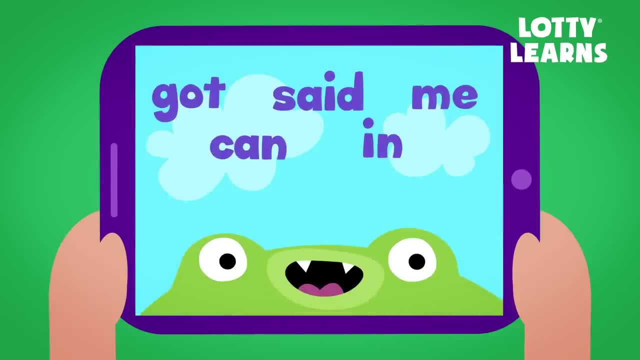 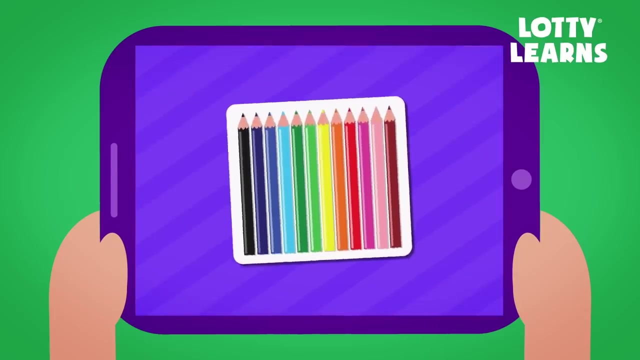 Which word says got Yep? How about me? Can you find in Great? Which word says can? And how about said Amazing, Nice job, You just won a gold star I-N. What should we use? You just won a sticker. 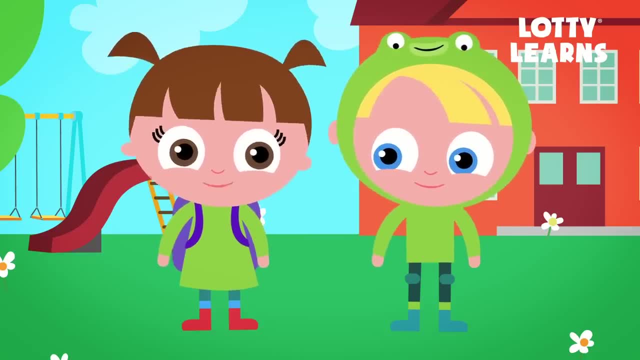 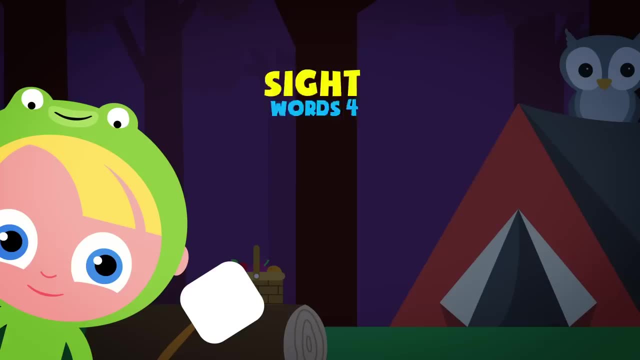 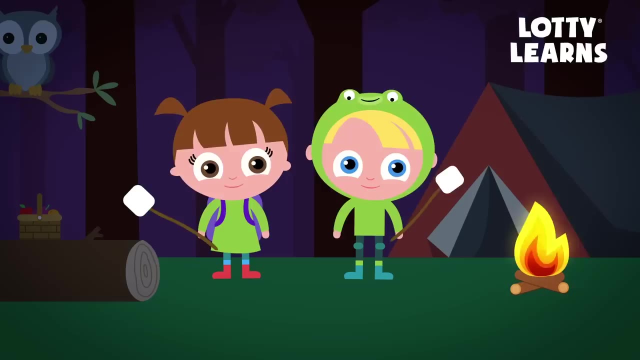 We had such a fun time with you. If you need more practice, go to our website or check out our free apps in the link below. LottieLearnscom. Sight Words 4. Hello friend, I'm Lottie And I'm Chuck. 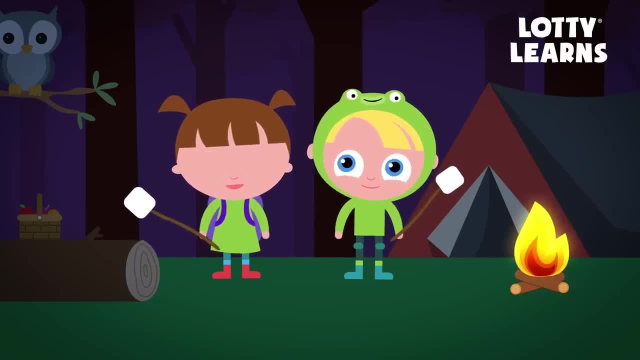 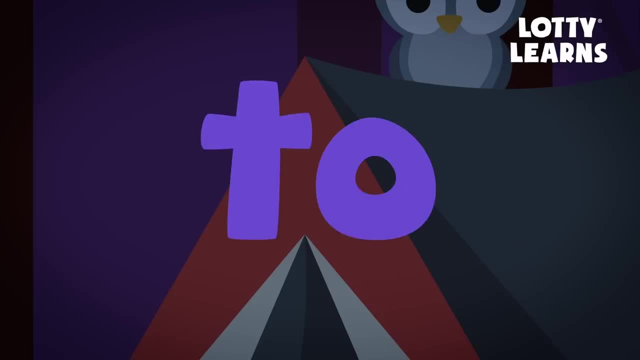 And today we're going to learn a few new words. All you have to do is remember how these words look and how they sound. Say them with me. Here we go. This first word is to T-O. To. This is the word is. 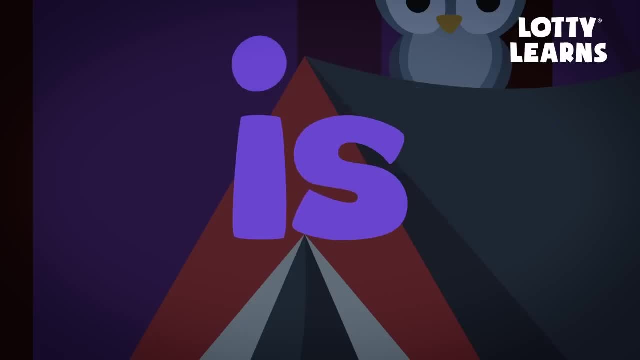 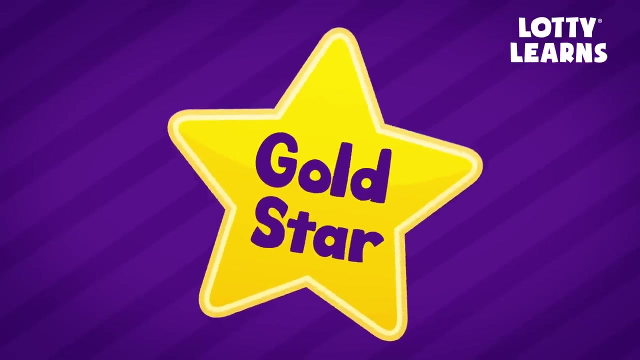 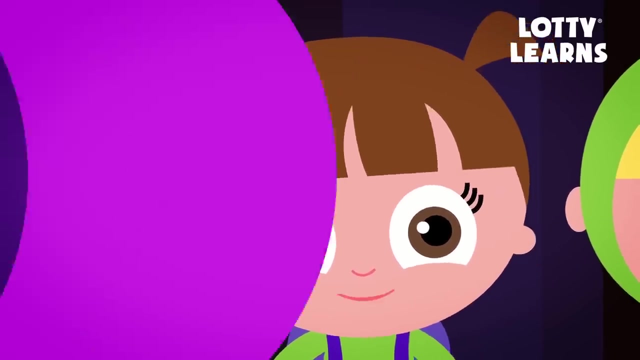 I-S Is. This word is but B-U-T, But This word is get, G-E-T, Get. And the last word is has H-A-S. Has Gold star, Gold star. It's time to review. Is there anything in my backpack that can help us? 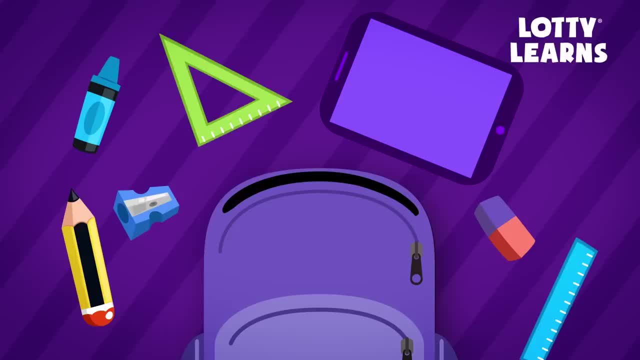 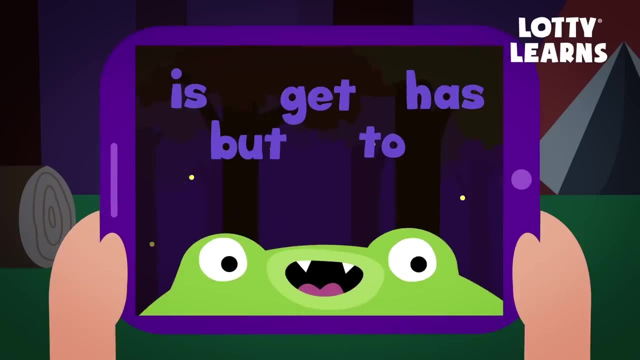 Hmm, What should we use? Hmm, What should we use? Awesome pick. Let's play a game. Which word says is? Which word says is Yep? How about has? How about has? Can you find two? Can you find two? 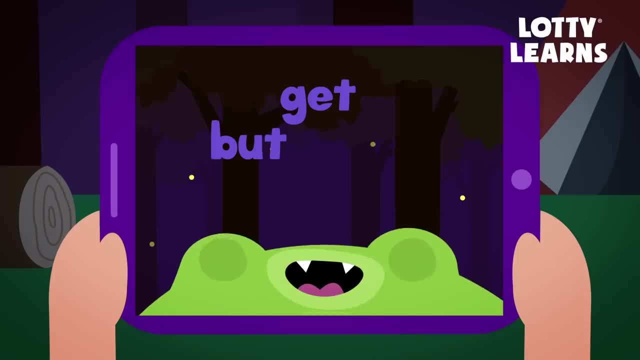 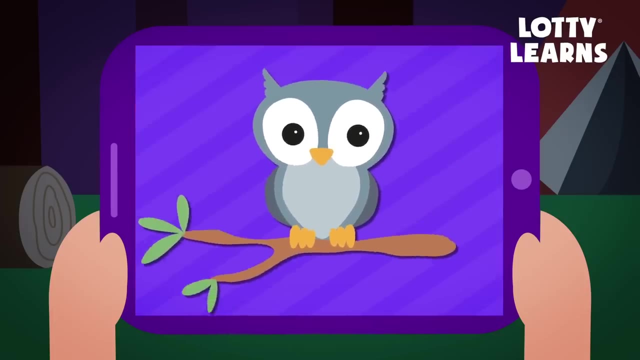 Great. Which word says, but. Which word says but. Which word says but? And how about get? And how about get? Amazing, Nice job, You just won a sticker. We had such a fun time with you. We had such a fun time with you. 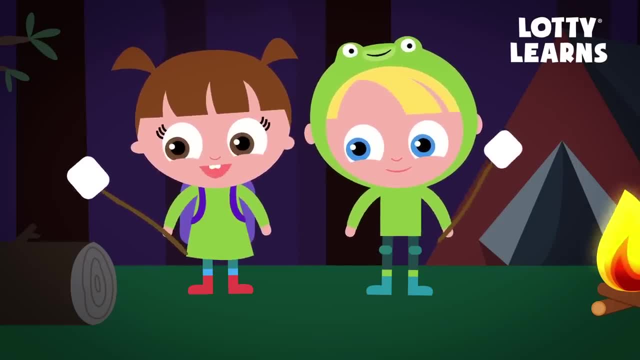 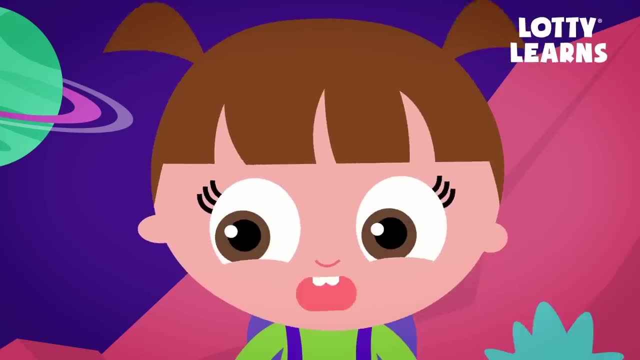 If you need more practice, go check out our free apps in the link below. LottieLearnscom Sight Words 5. Hello friend, I'm Lottie And these are my friends Fuzz, Chuck and Chip. Hello. 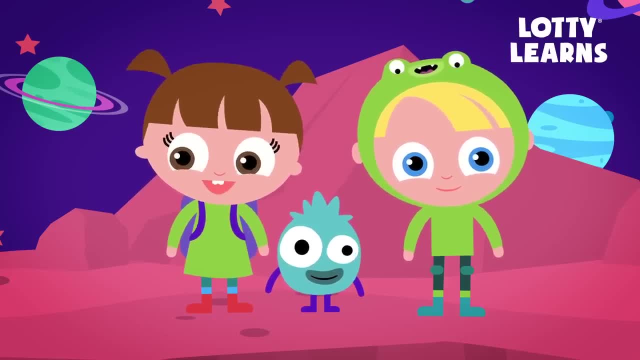 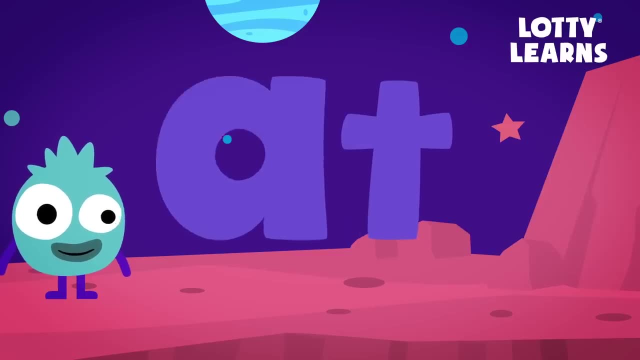 Today we're going to learn some new words. All you have to do is remember how these words look and how they sound. Say them with me. This first word is at A-T At. This word is did, D-I-D Did. This is the word my 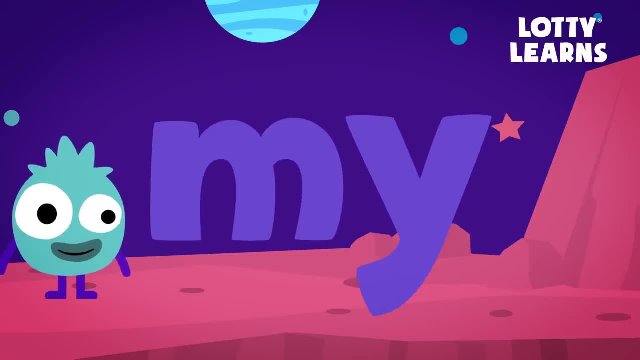 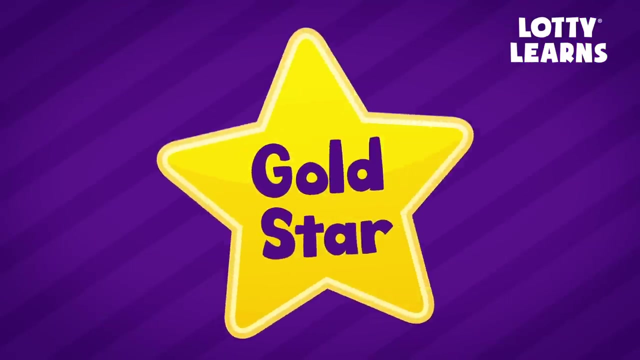 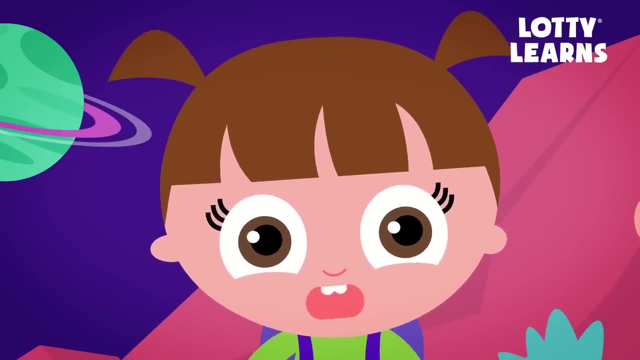 M-Y, My. This word is for F-O-R, For, And the last word is up U-P, Up Gold star. It's time to review. Is there anything in my backpack that can help us? Hmm, What should we use? Awesome pick. 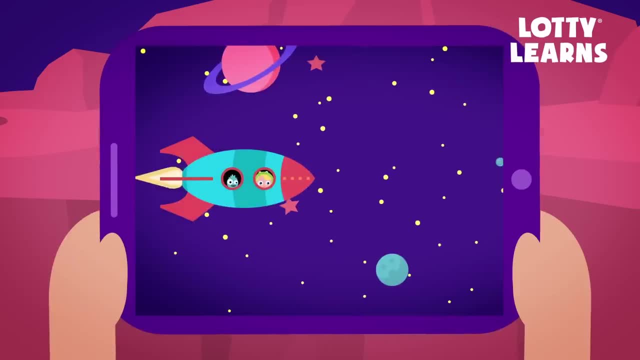 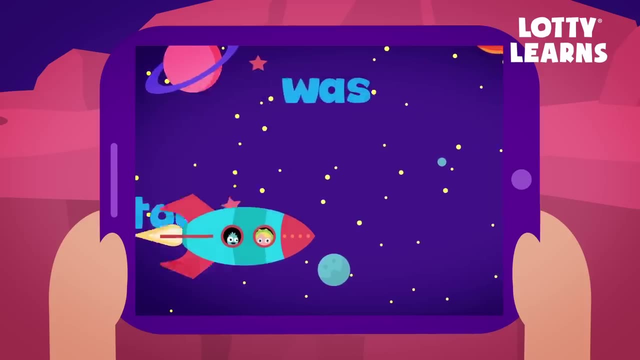 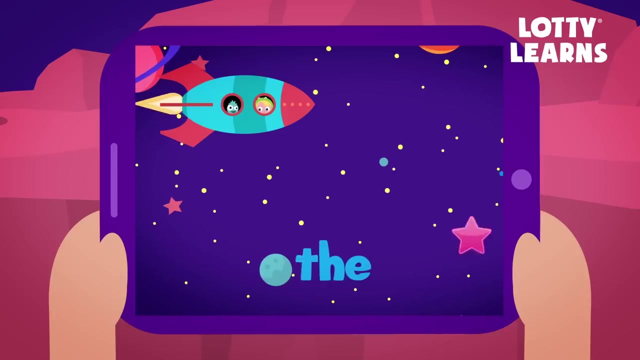 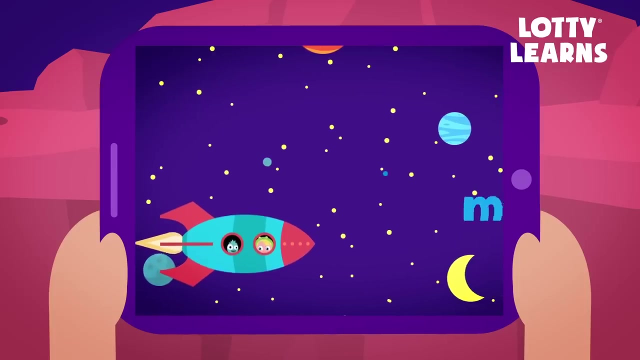 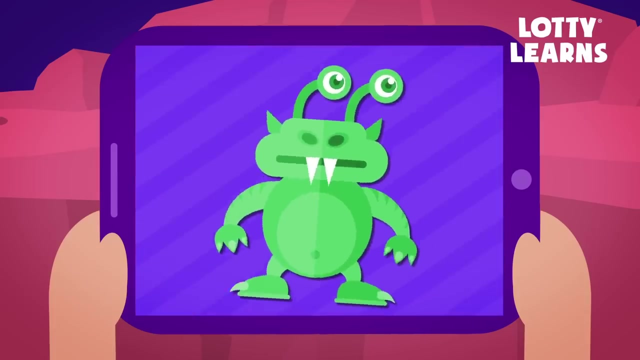 Let's play a game. Which word says did, Did Great. How about for, For, For, For, Yep? Can you find at At Nice job? Which word says my, My Yep. And how about Up, Up, Amazing Nice job? 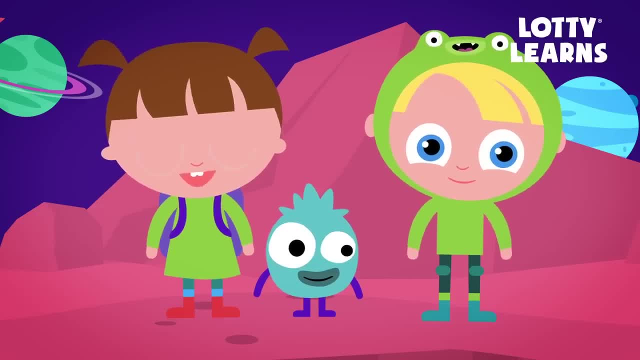 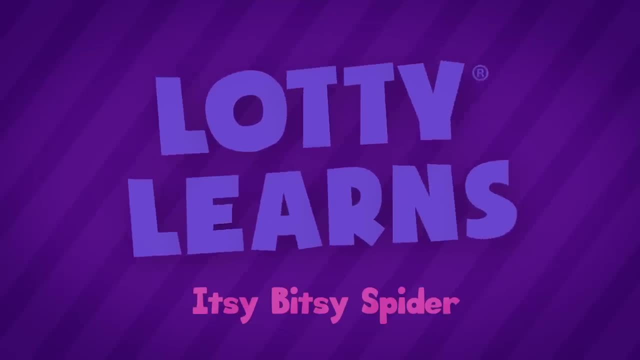 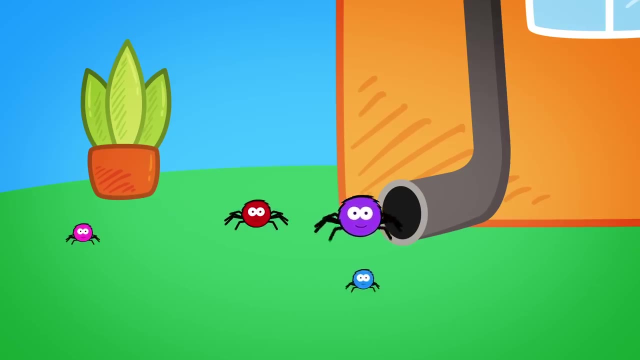 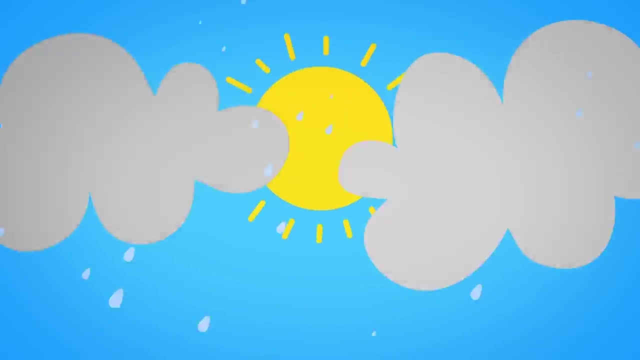 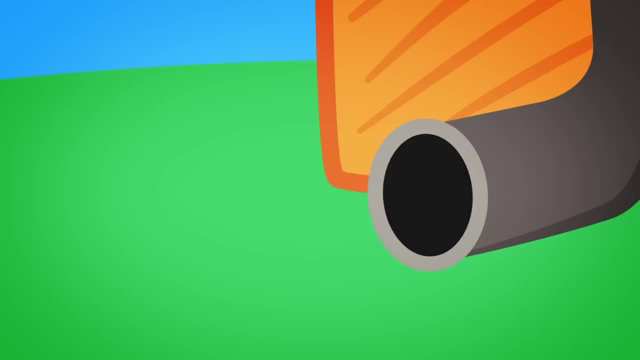 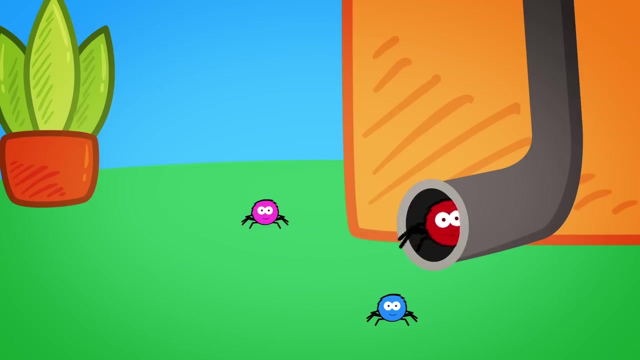 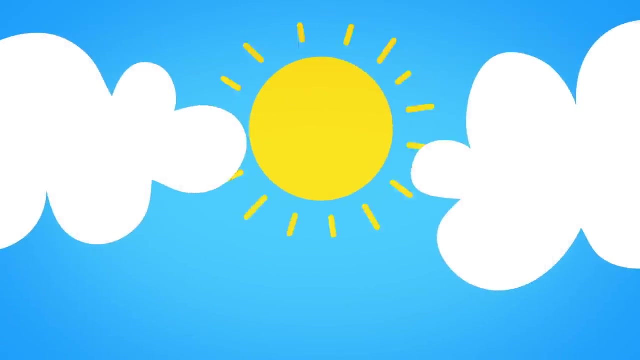 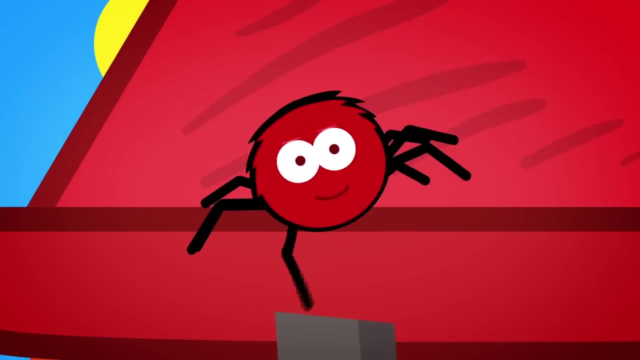 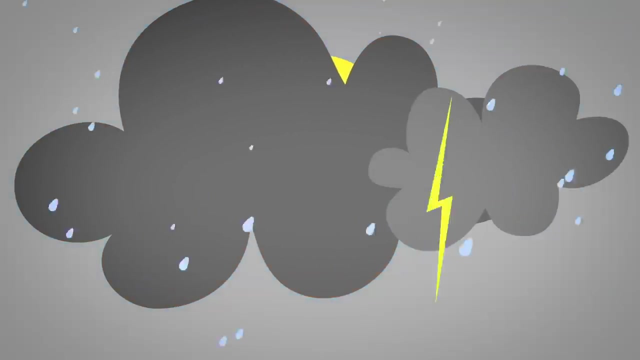 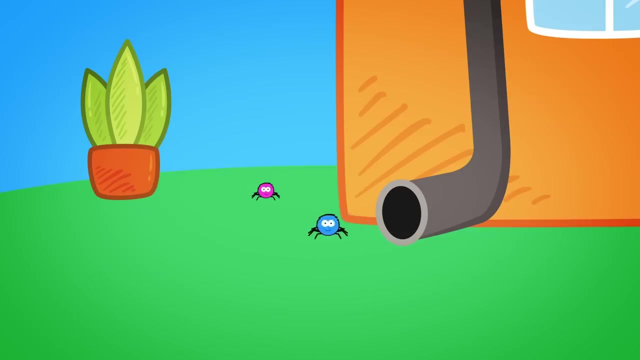 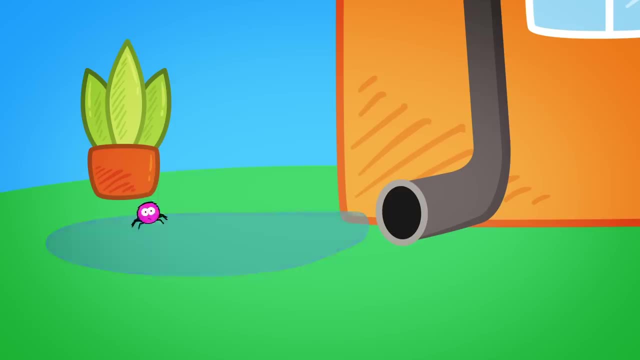 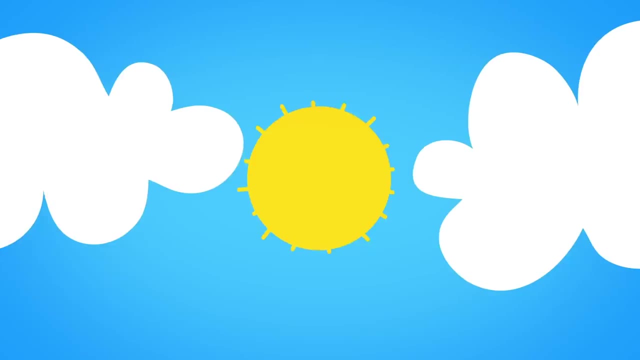 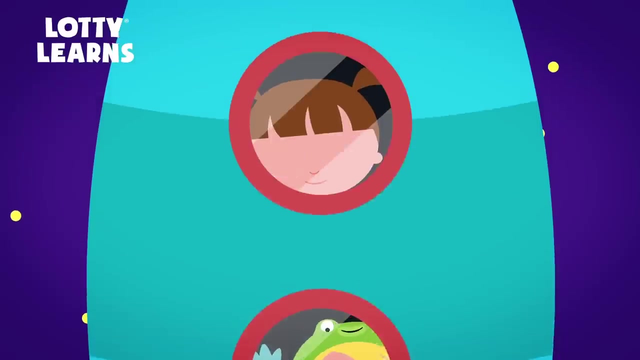 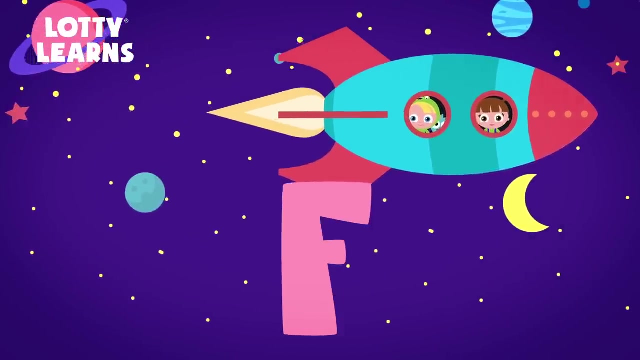 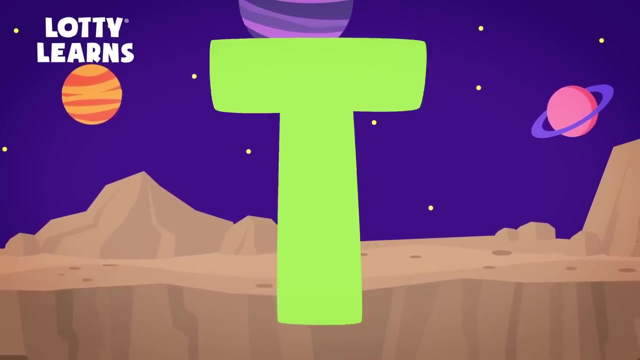 Up came the sun and dried up all the rain. So the itsy bitsy spider went up the spout again. A, B, C, D, E, F, G, H, I, J, K, L, M, N, O, P, Q, R, S, T, U, V, W, X, Y and Z. 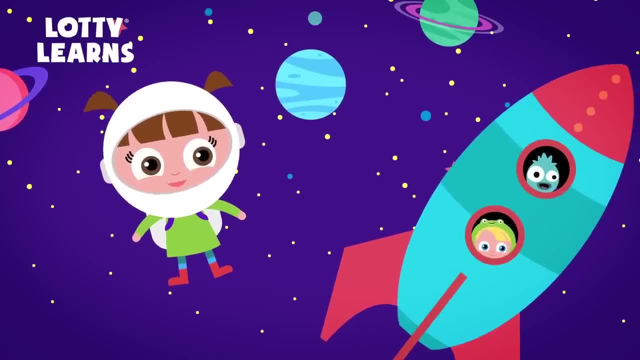 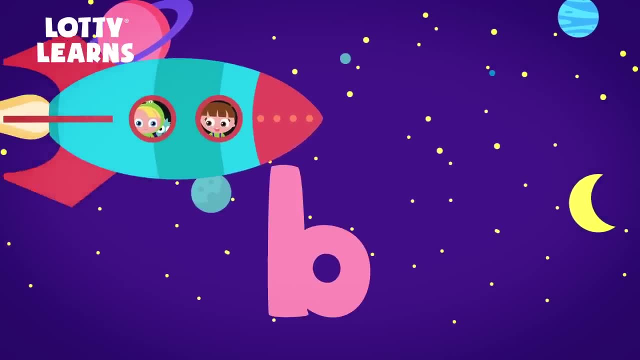 Now I know my ABCs. next time won't you sing with me Lowercase A, B, C, D, E, F, G, H, I, J, K, L, M, N, O, P, Q, R, S, T, U, V, W, X, Y and Z. 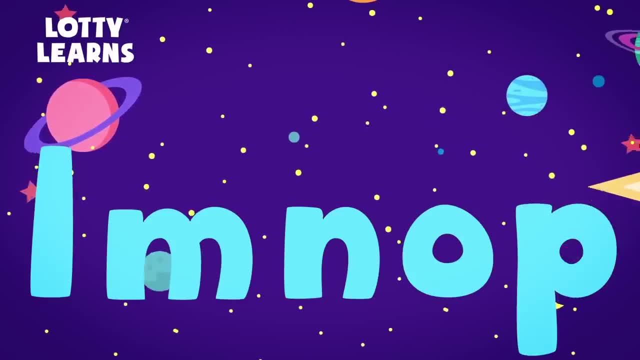 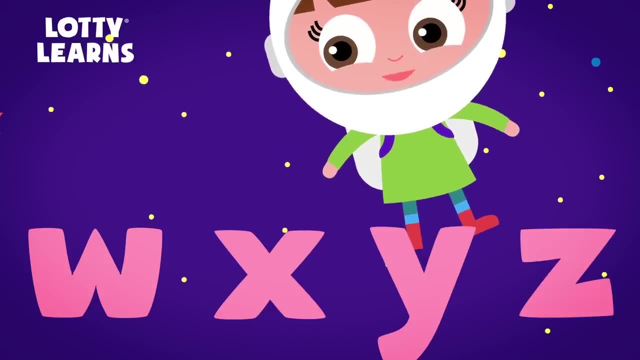 Lowercase A, B, C, D, E, F, G, H, I, J, K, L, M, N, O, P, Q, R, S, T, U, V, W, X, Y and Z. 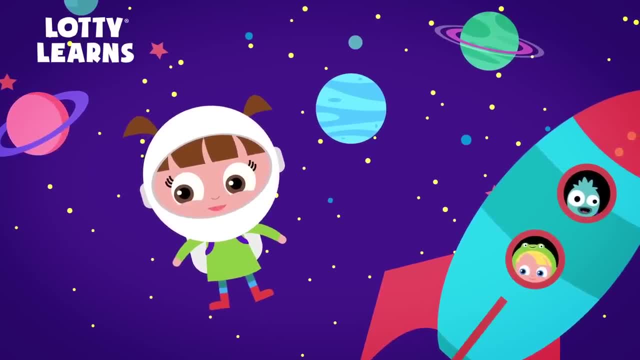 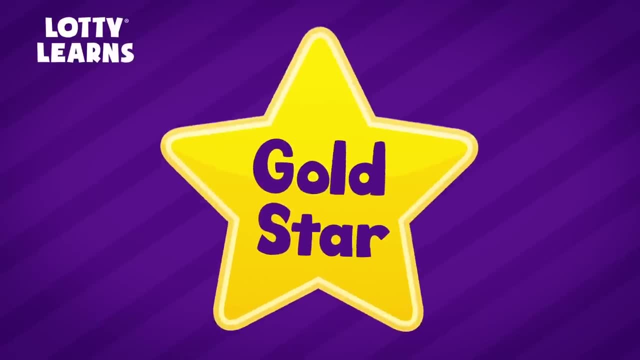 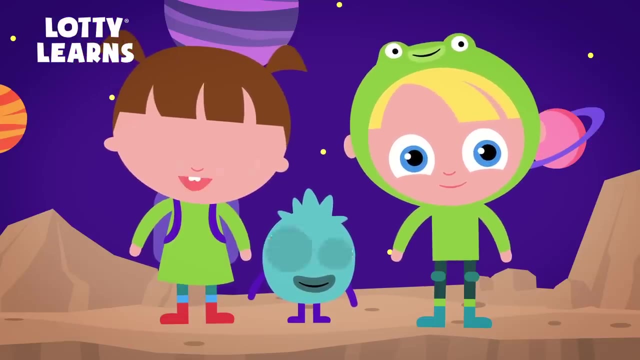 Now I know my ABCs. next time won't you sing with me, Gold star? That was all of the upper and lowercase letters. Great job, If you ever forget what the letters mean, they're always in the upper and lowercase. Great job. If you ever forget what the letters mean, they're always in the upper and lowercase. 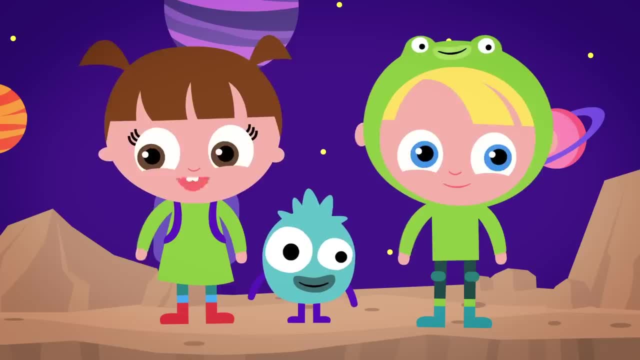 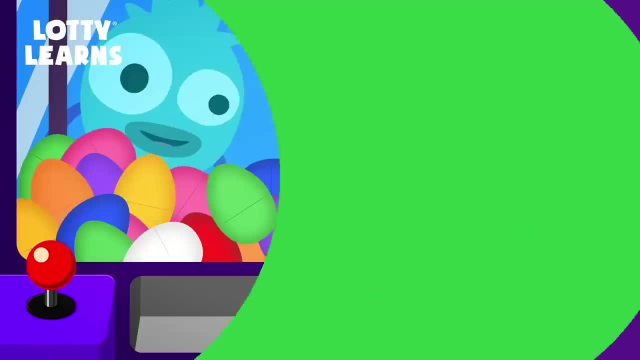 So american learners learn the letters like the numbers on paper. We have a lot of hard work to get done and are glad you could all watch this video, because the numbers aren't enough to help. Thanks for learning with us. We had such a fun time. 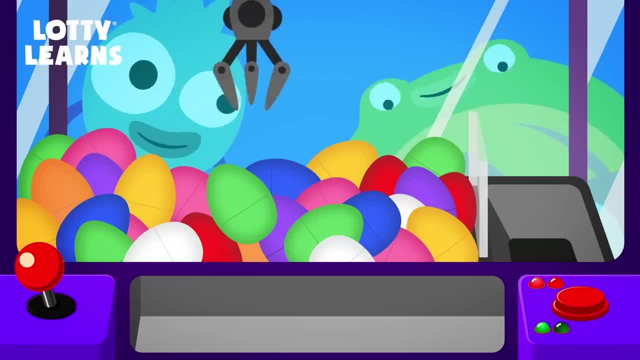 Hope you visit us again soon. jemand conoc campers livelihood. Who are the colonists in one? Can you guess what color the egg will be? Can you guess what color the egg will be? Can you guess what color will the egg be? Once we get one, we can see what's inside. 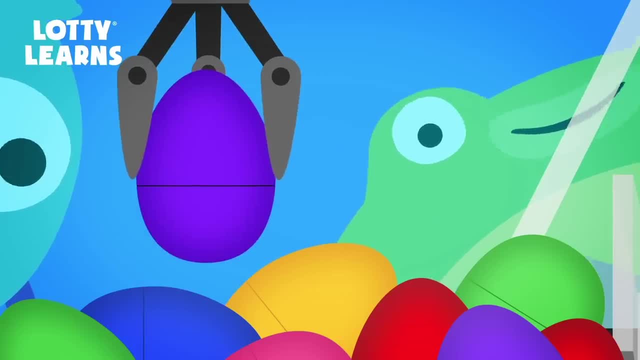 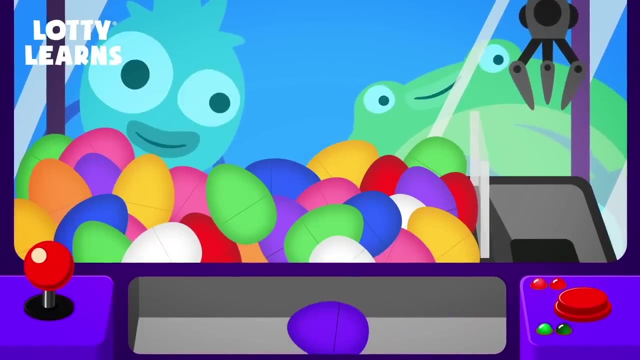 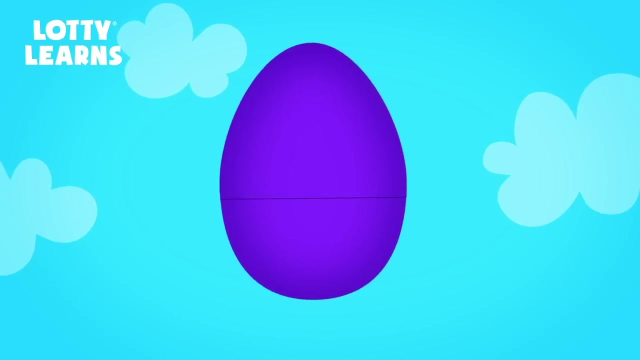 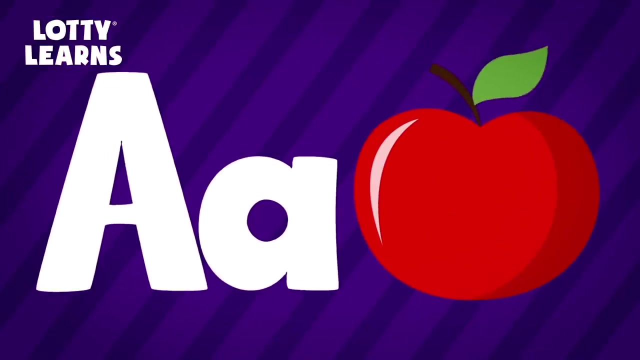 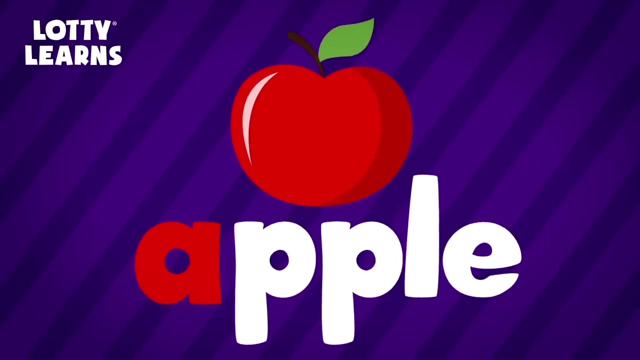 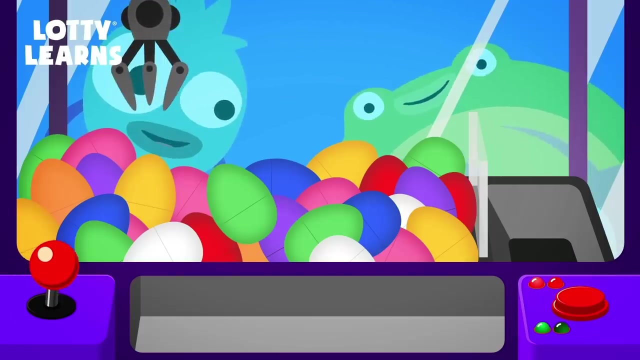 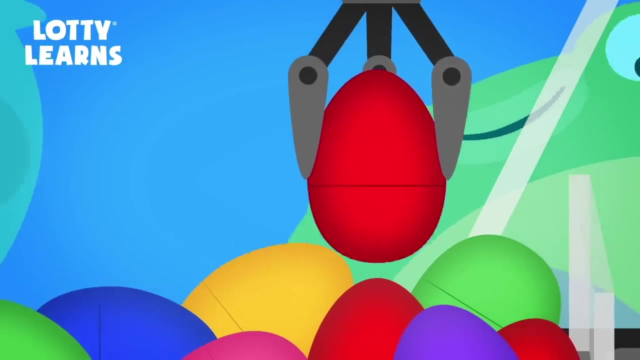 Can you guess what color the egg will be? Ooh, a purple egg. I wonder what's inside. A Apple A is for apple. Let's play again. Can you guess what color the egg will be? I grabbed a red egg. 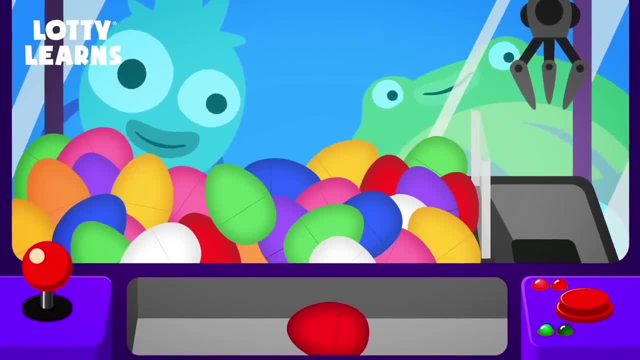 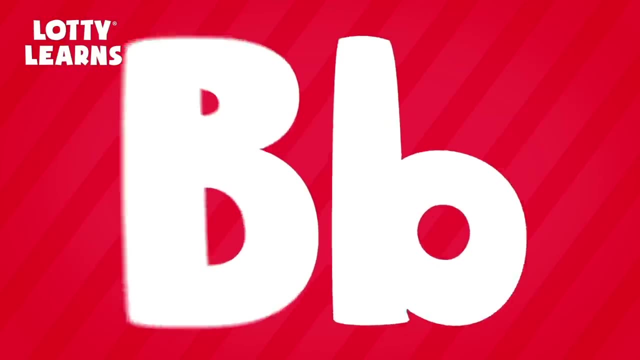 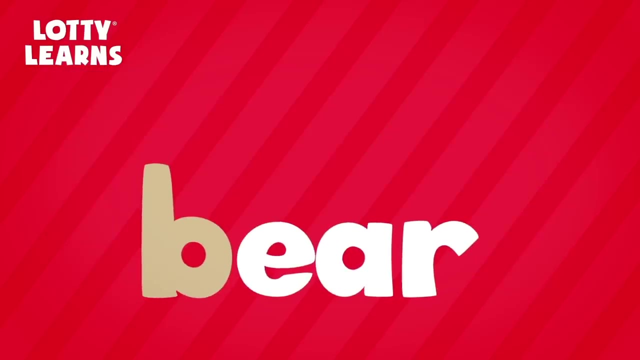 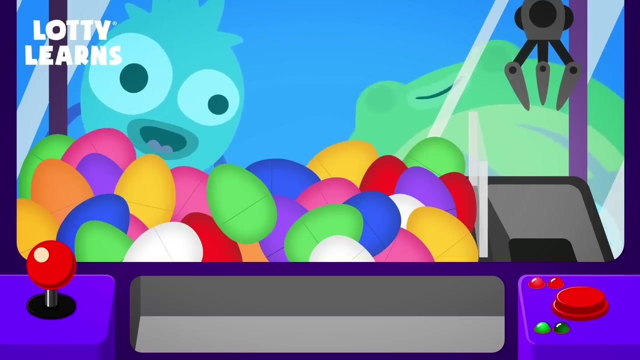 I wonder what's inside this egg. A, B, B, B, B, B, B. B is for bear, B is for bear. Let's play again. Let's play again. Once we get one, we can see what's inside. 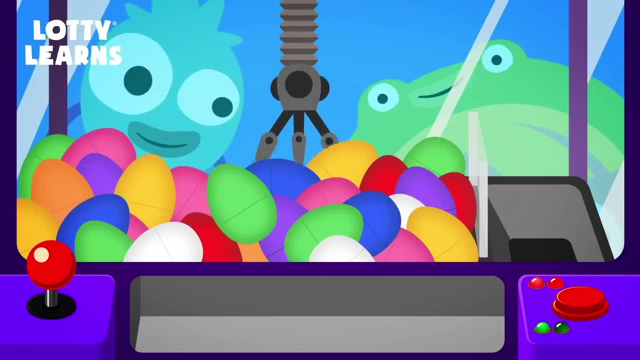 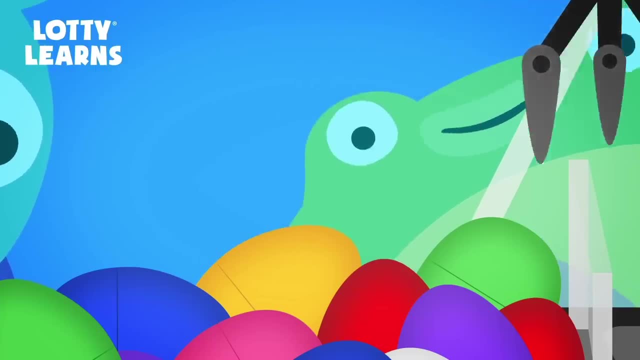 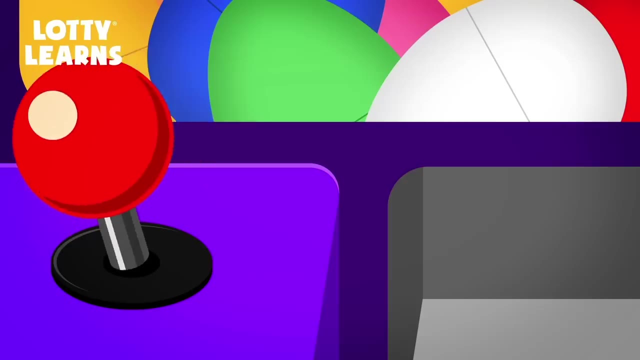 Once we get one, we can see what's inside. Once we get one, we can see what's inside. Uh, try again, Let's play again. I wonder what color we'll get this time. I wonder what color we'll get this time. 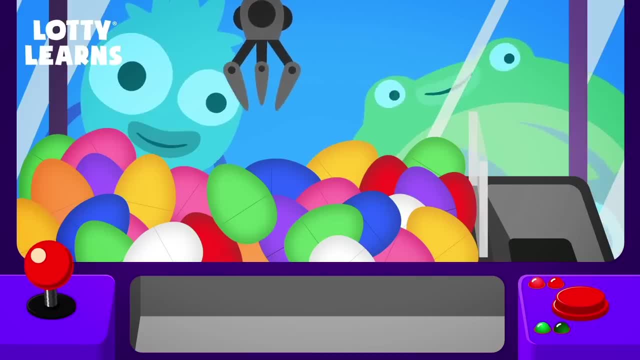 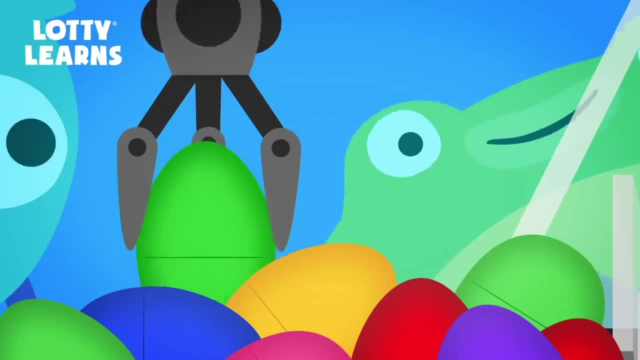 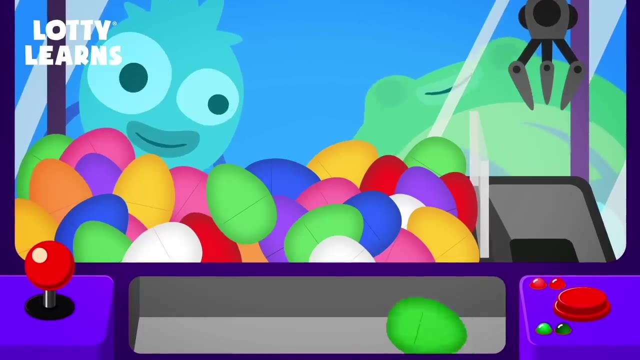 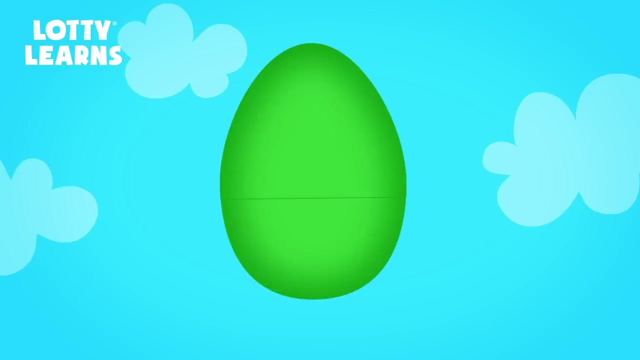 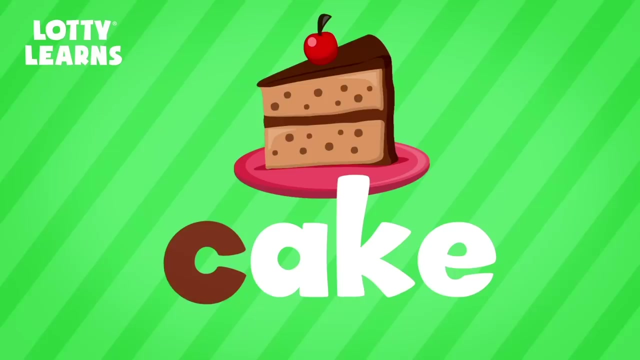 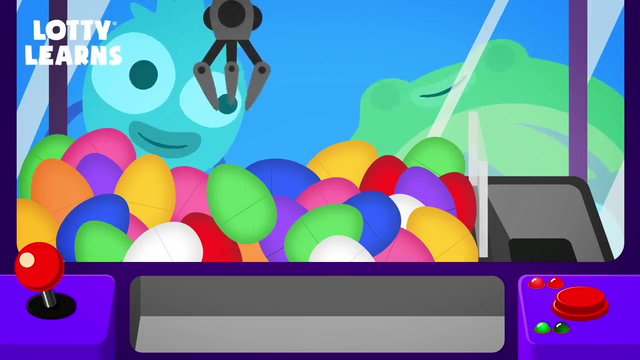 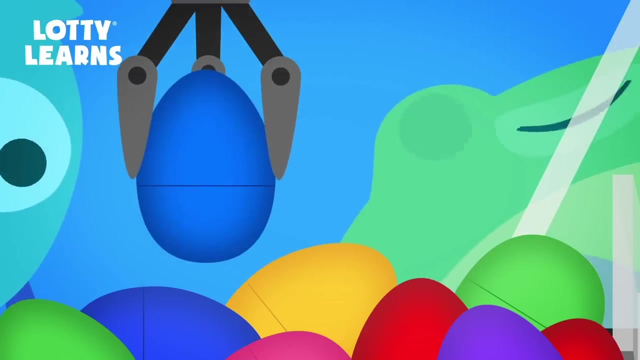 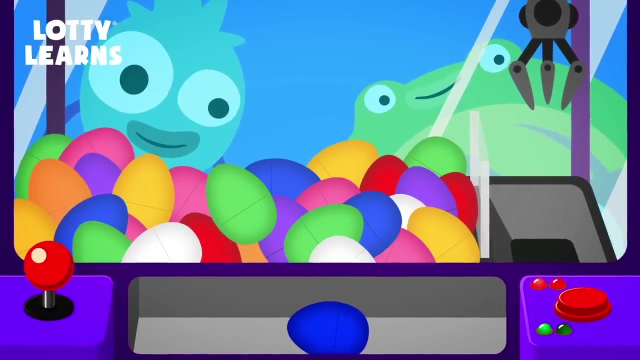 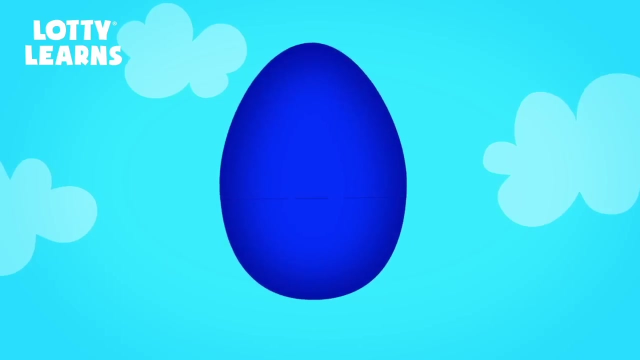 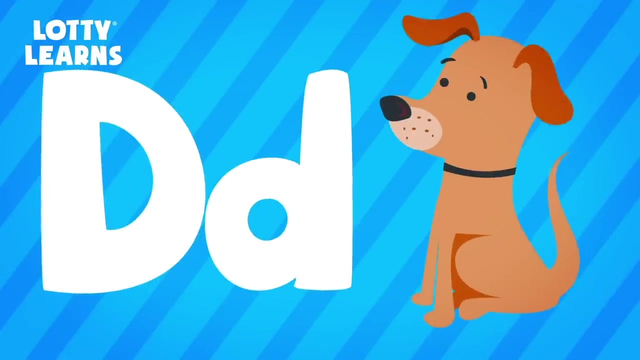 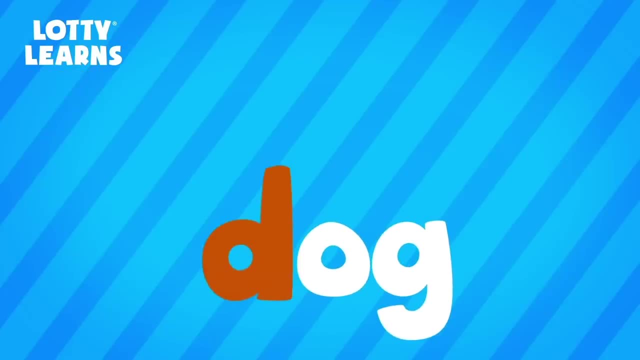 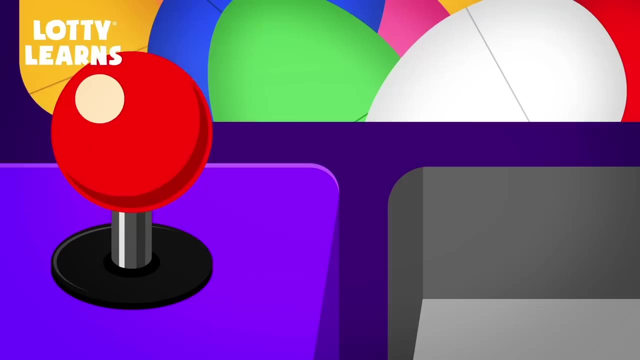 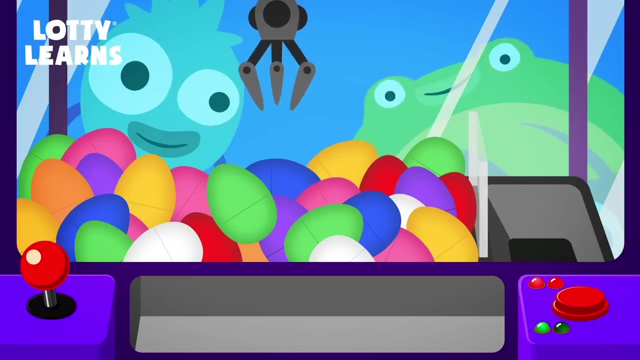 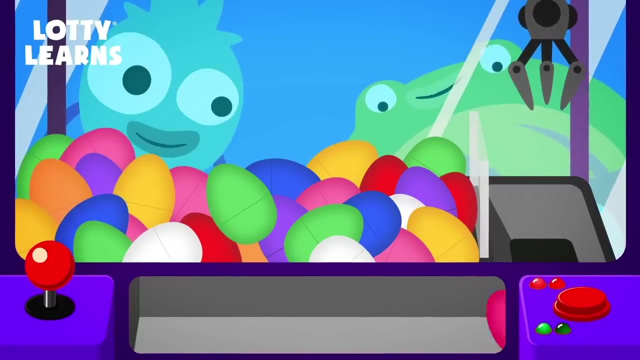 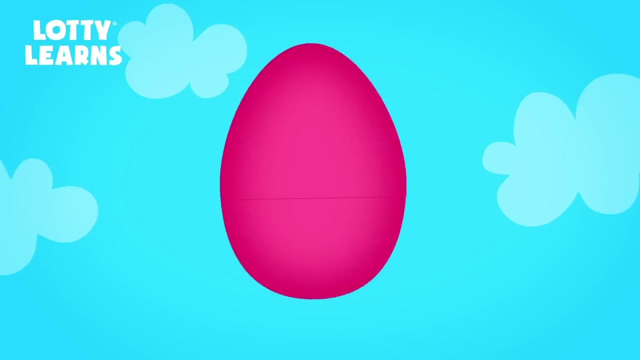 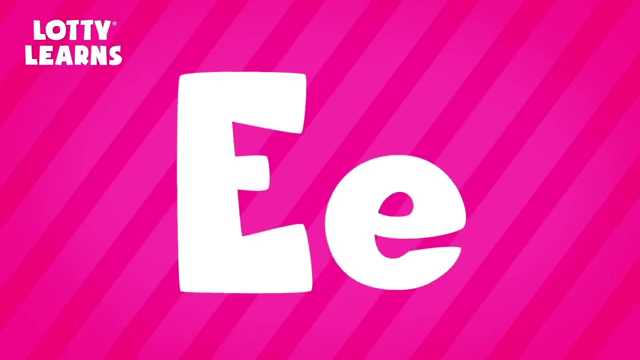 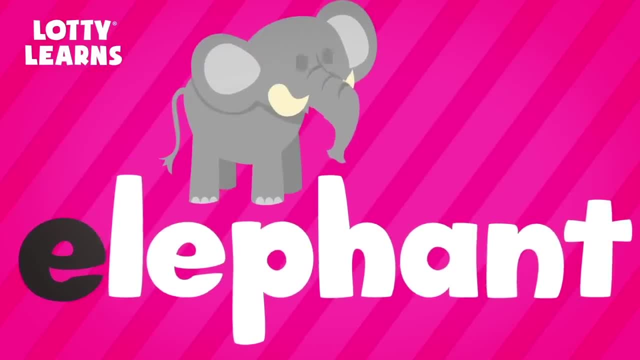 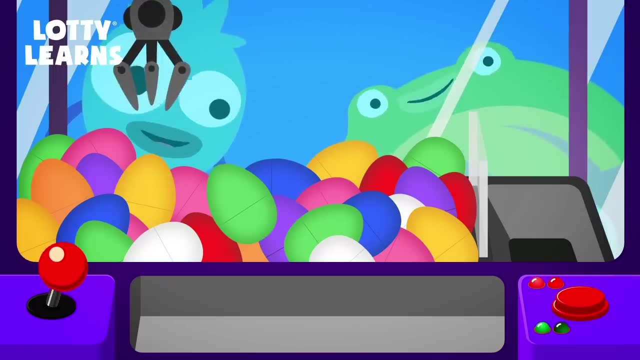 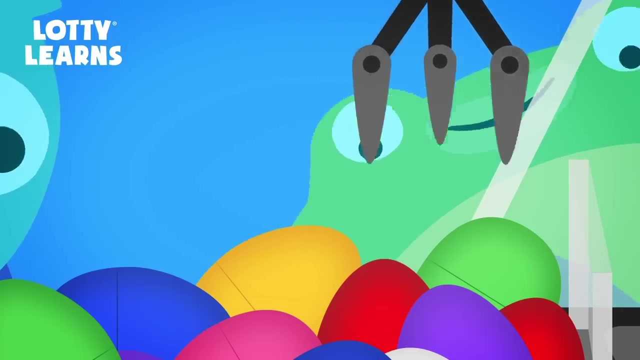 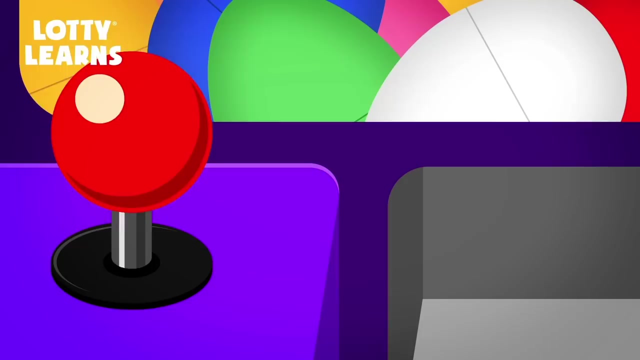 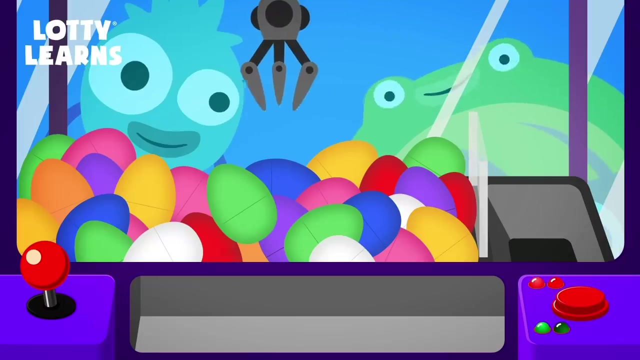 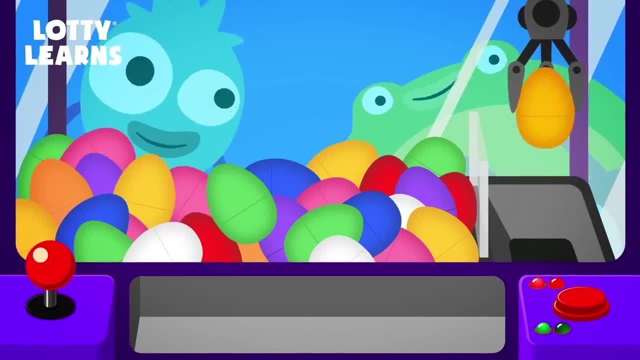 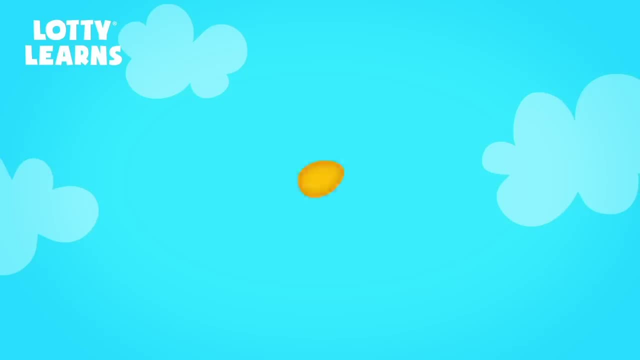 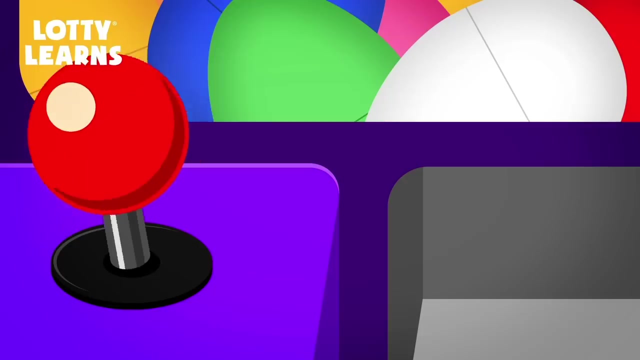 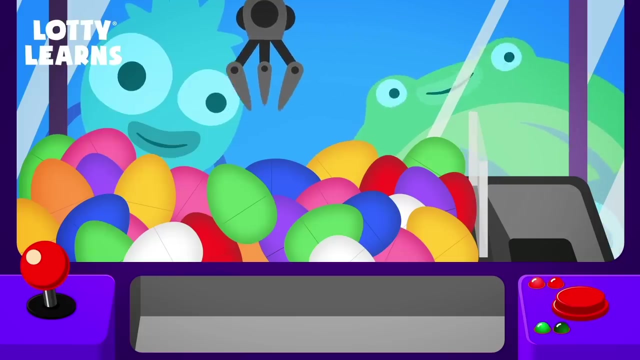 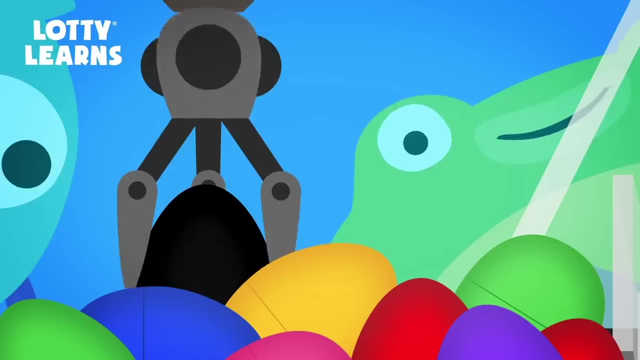 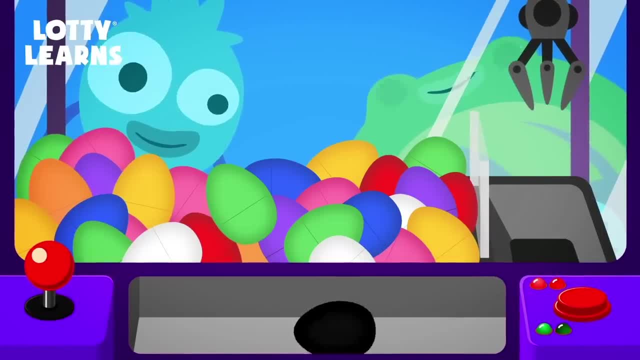 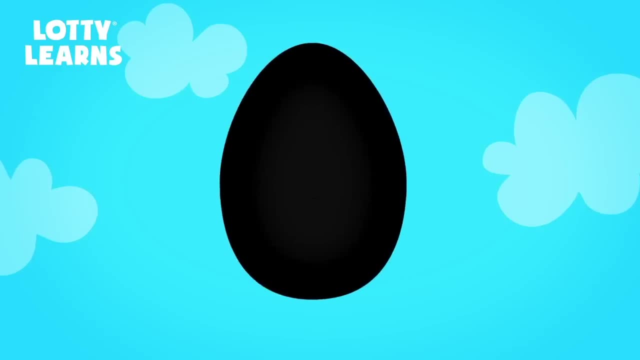 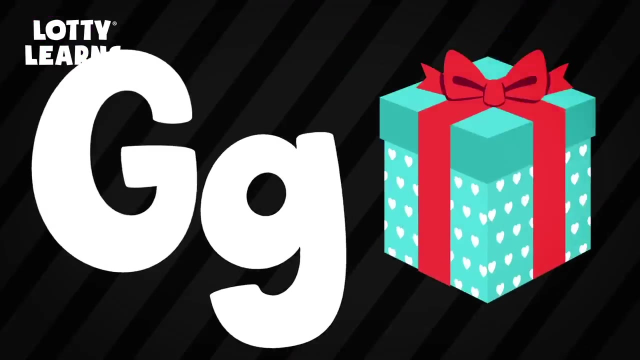 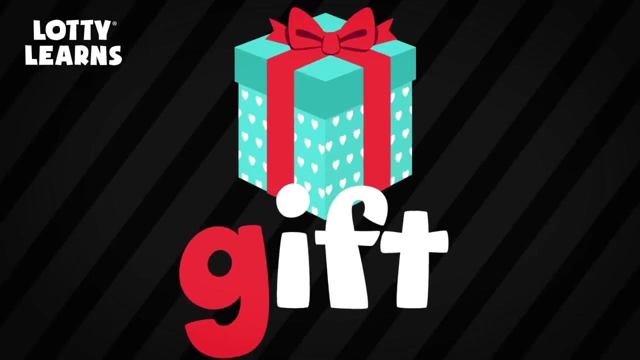 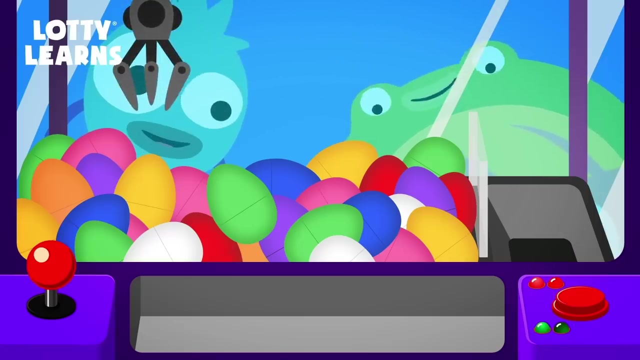 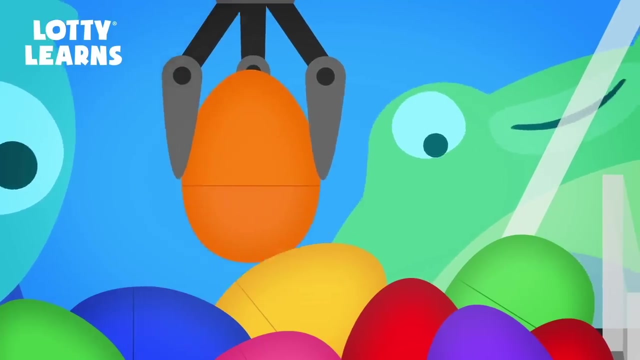 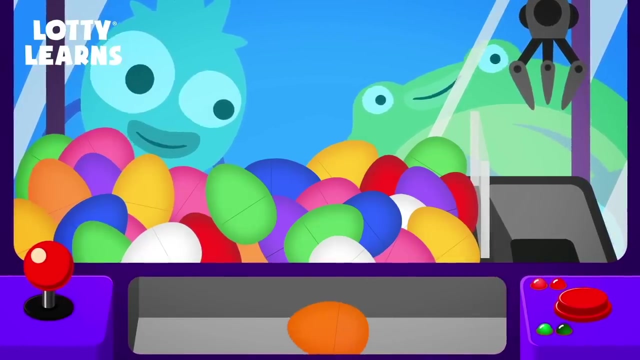 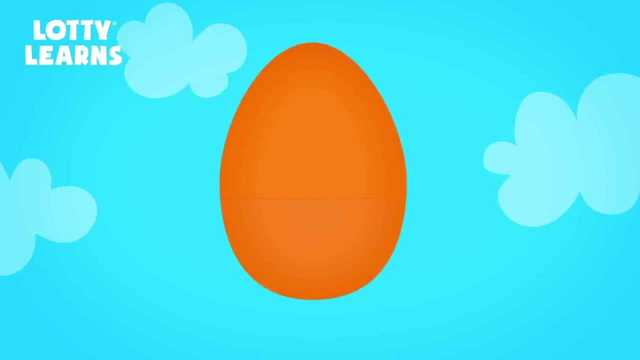 I wonder what's inside G G gift G is for gift. I wonder what color will get. this time we grabbed an orange egg. I wonder what's inside this gift G gift G is for gift. G is for gift. we grabbed an orange egg. G gift G is for gift. 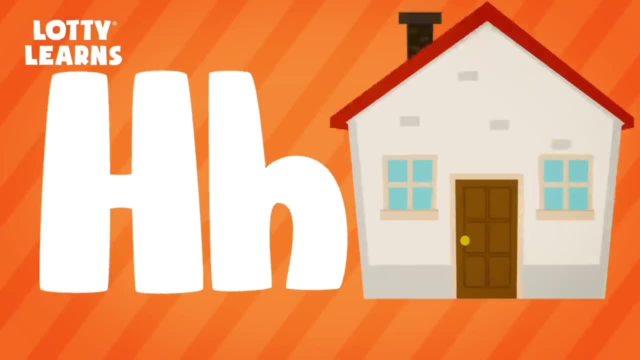 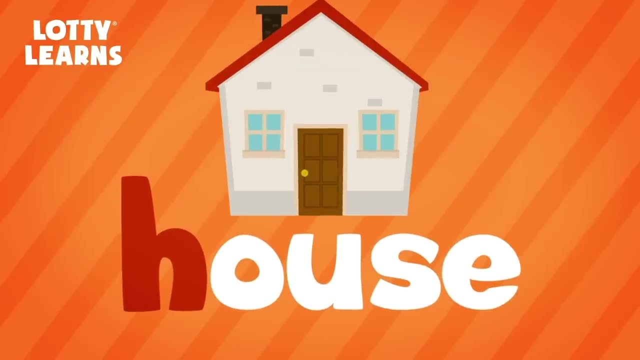 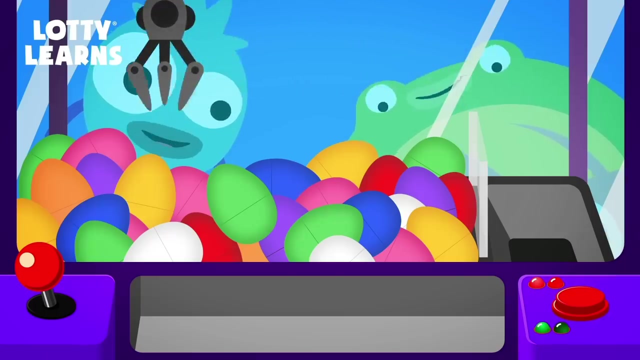 I wonder what's inside. G G gift G is for gift. let's play again. I wonder what color we'll get this time. once we get one, we can see it's inside G G gift. G is for gift. we grabbed an orange egg. G gift G is for gift. G is for gift. 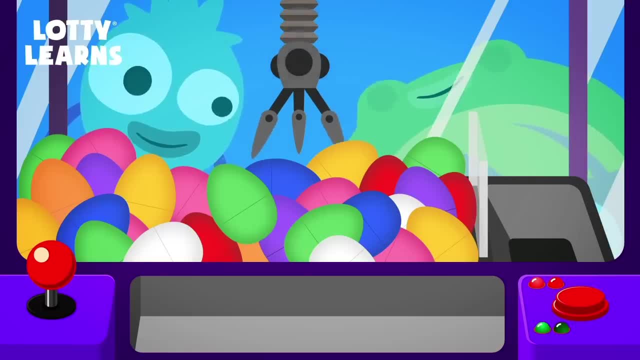 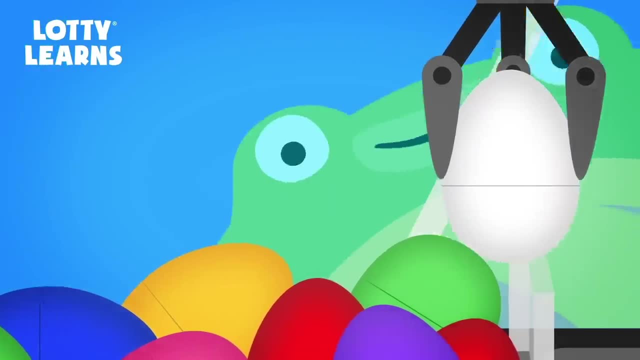 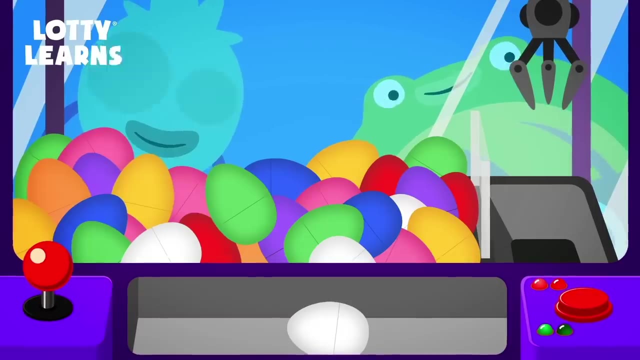 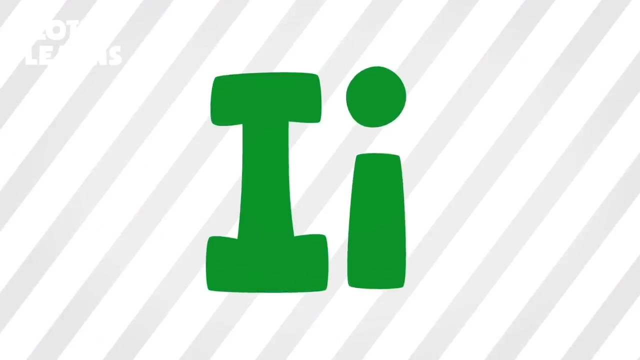 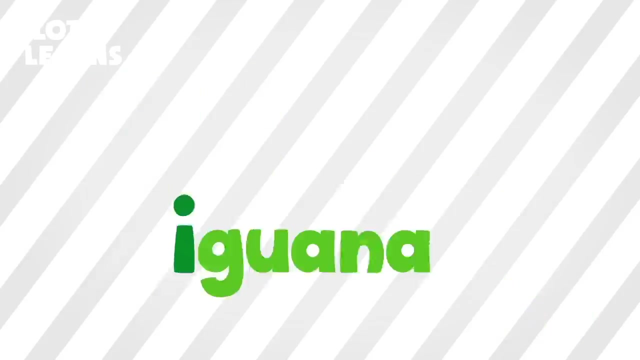 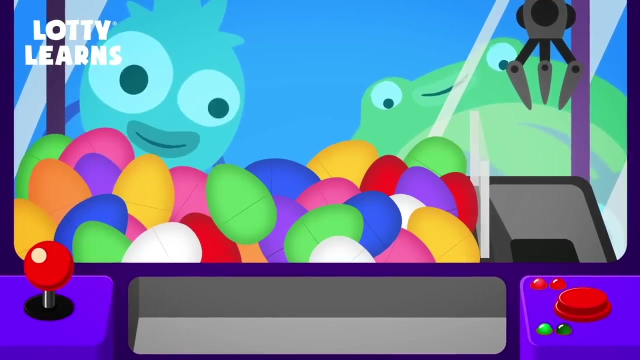 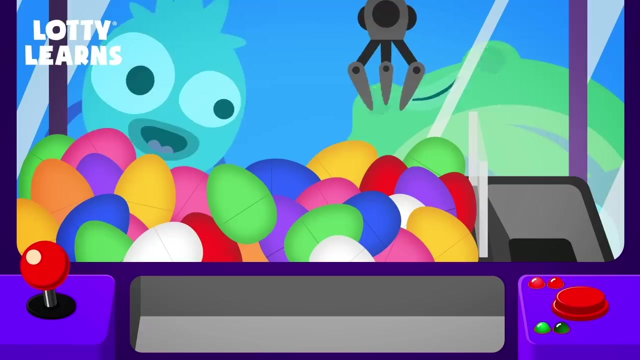 Let's see what's inside. Ooh white, I wonder what's inside. I I Iguana, I is for Iguana. Let's play again Once we get one. we can see what's inside Blue Blue itself. 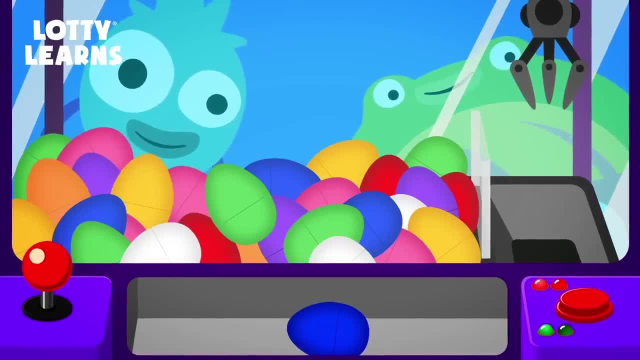 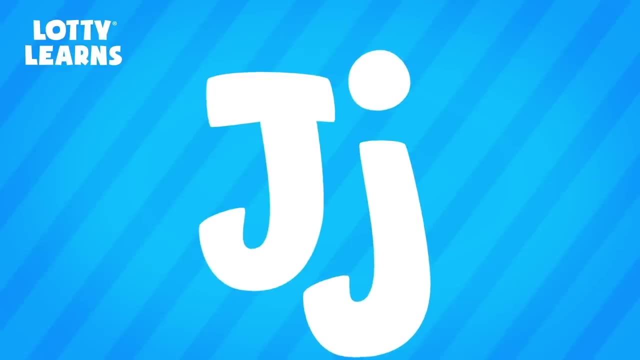 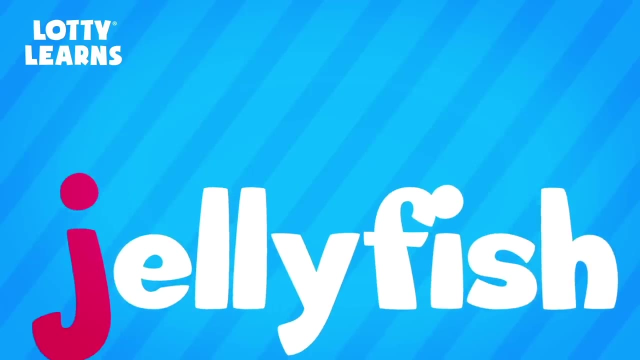 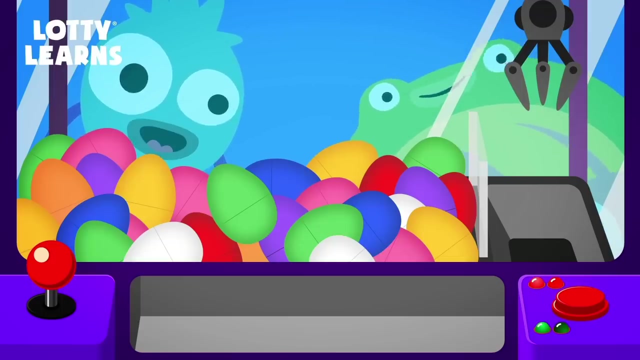 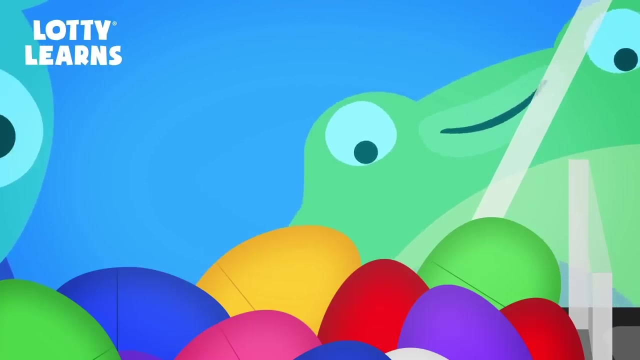 I wonder what's inside J? J, It's the jellyfish. J is for It's the jellyfish. Let's play again. Once we get one, we can see what's inside. Oop, Try again. Let's play again. 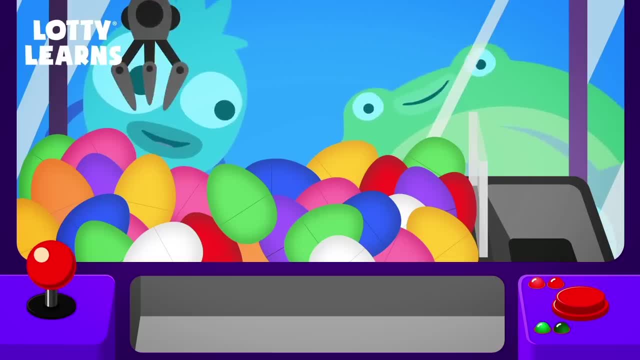 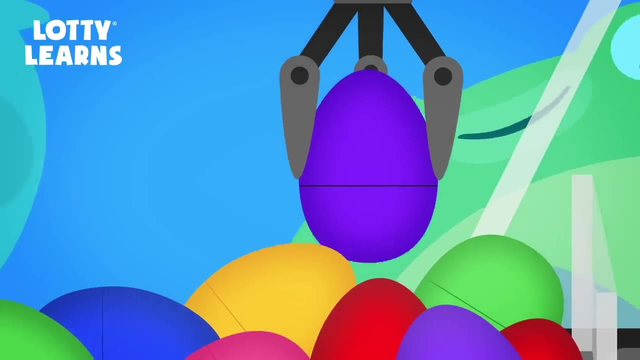 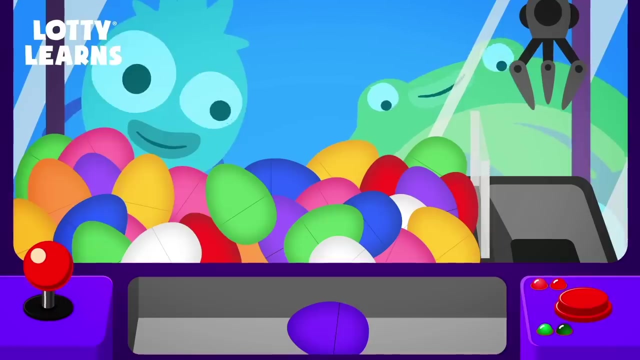 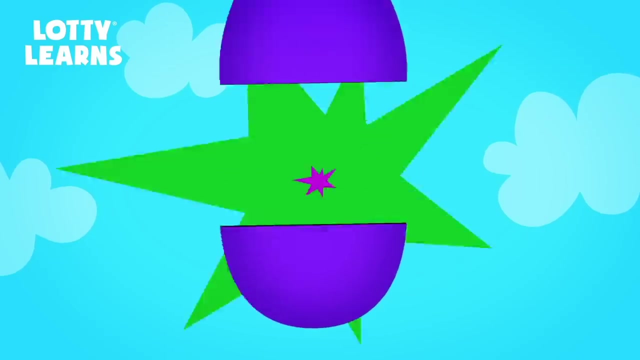 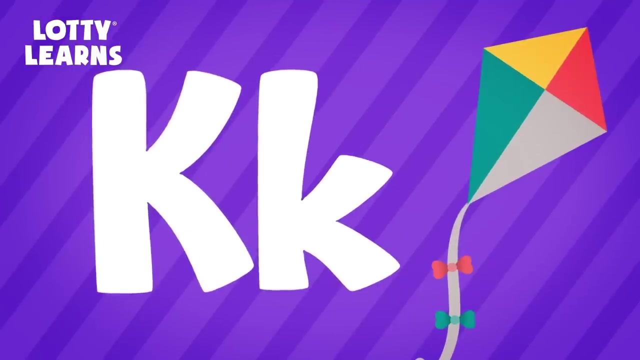 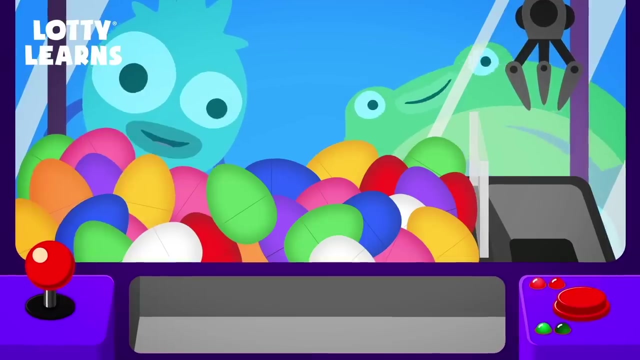 I wonder what color we'll get this time. Ooh, a purple egg. I wonder what's inside. I wonder what's inside K K, Kite, Kite. K K is for kite. Let's play again. 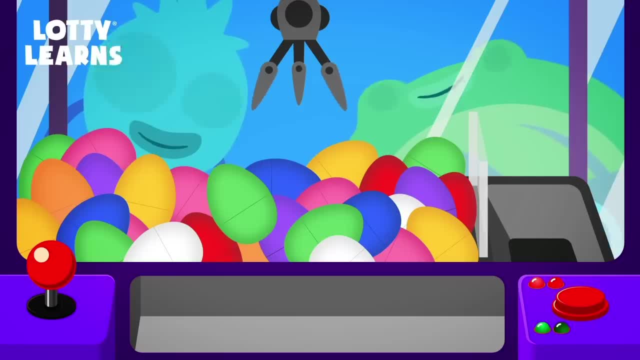 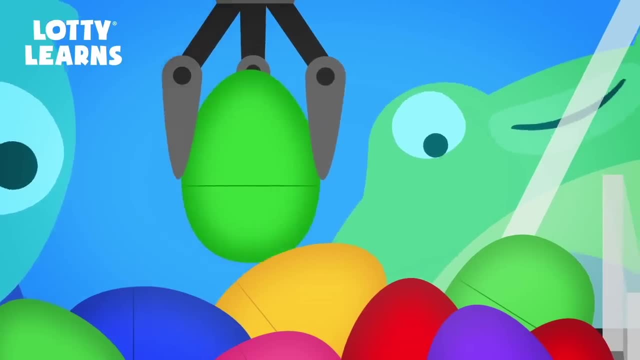 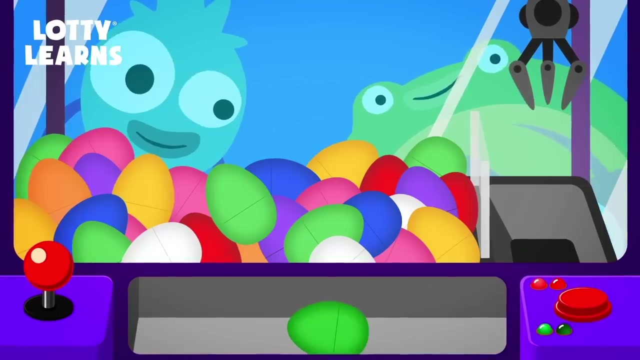 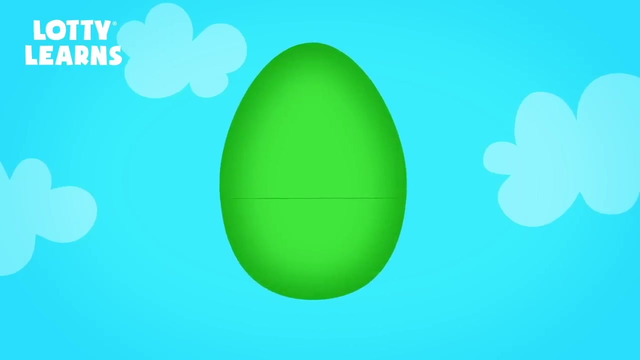 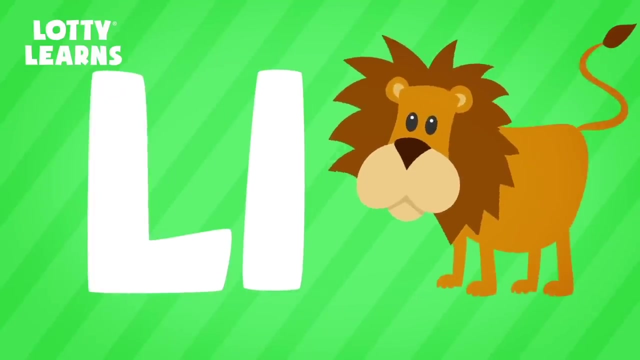 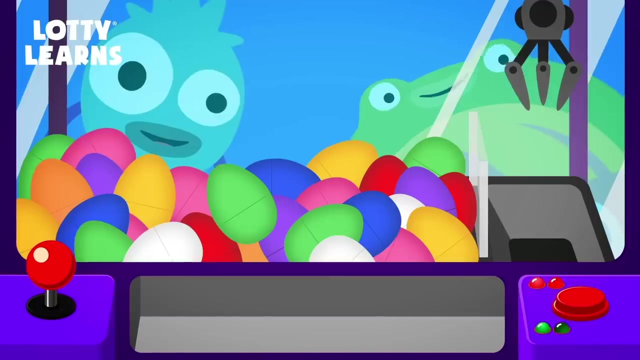 Once we get one, we can see what's inside. Oop, Let's play again. Green. I wonder what's inside. L Lion, Elephant, Lion, Let's play again. Can you guess what color the egg will be? We grabbed a purple egg. 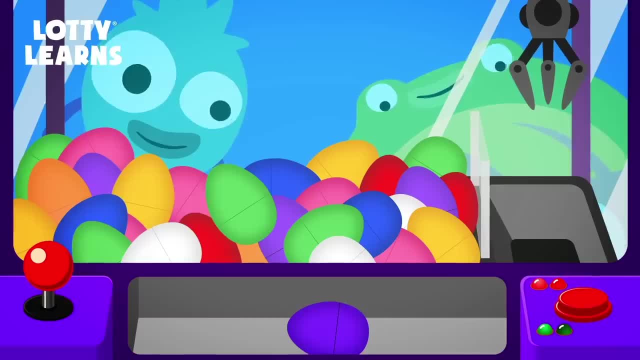 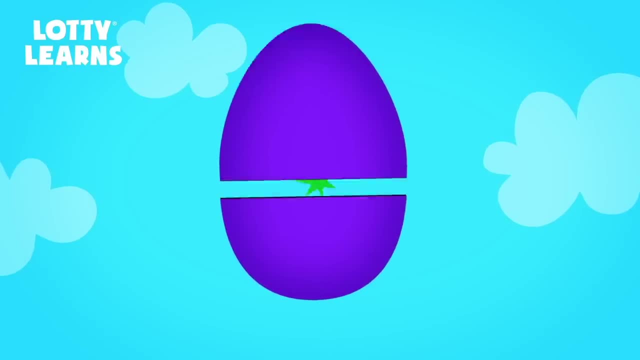 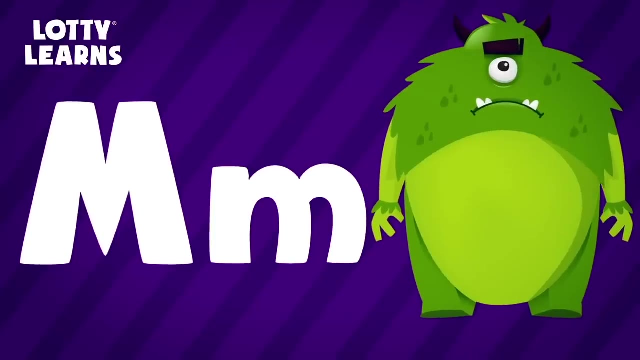 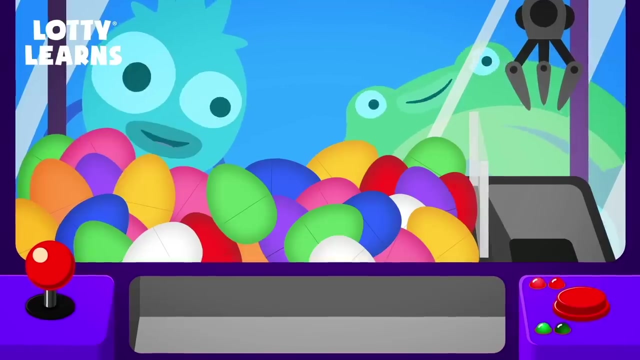 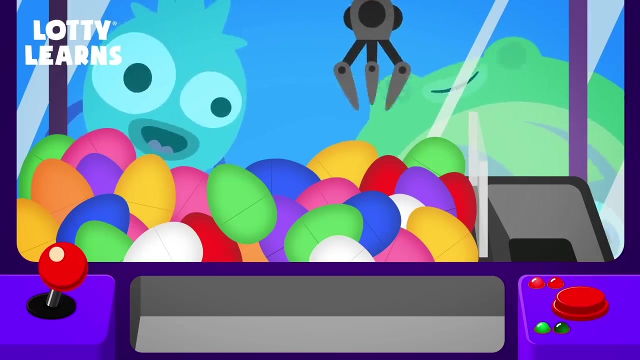 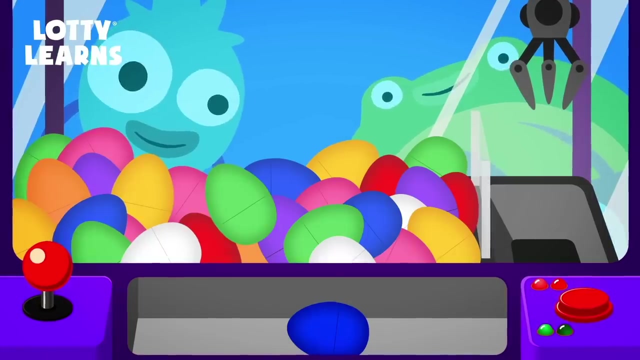 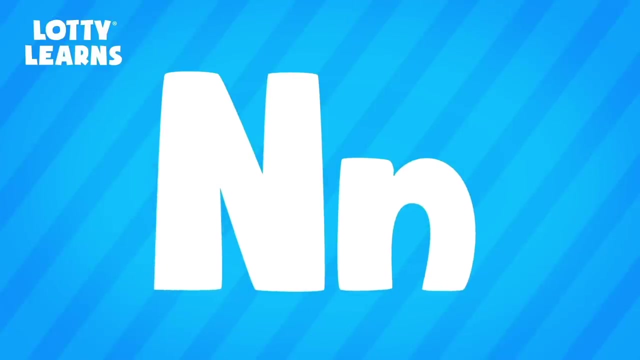 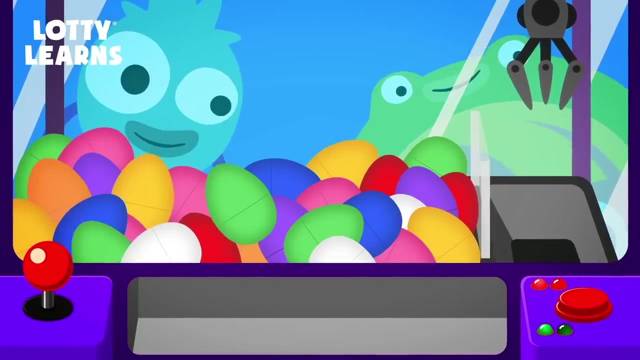 I wonder what's inside M Monster- M is for Monster. Let's play again. Once we get one, we can see what's inside. We grabbed a blue egg. I wonder what's inside. Yellow, Yellow, Blue N Nose- N is for nose. Let's play again. Can you guess what color the egg will be? 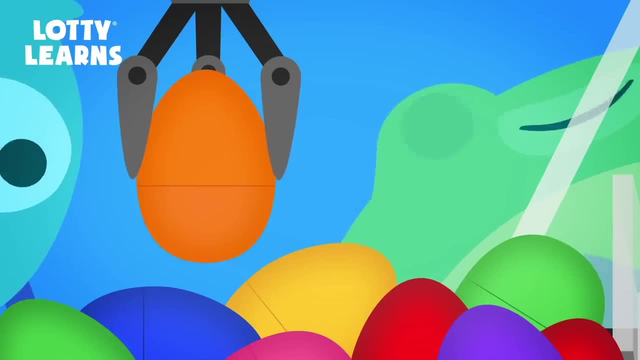 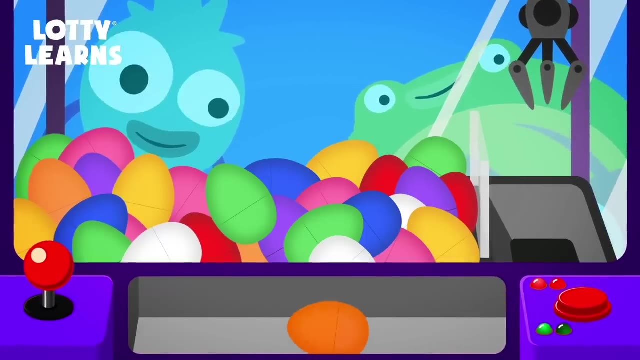 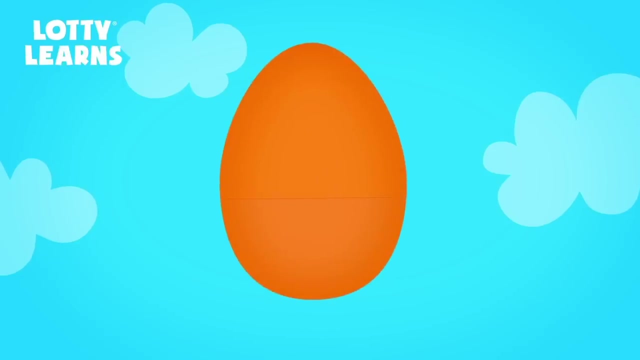 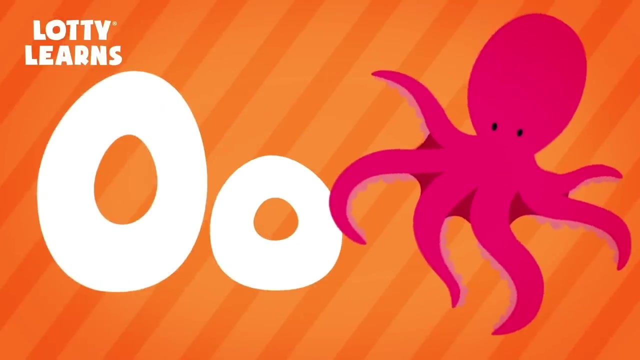 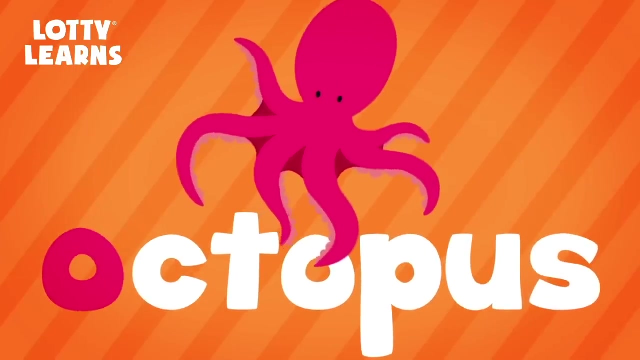 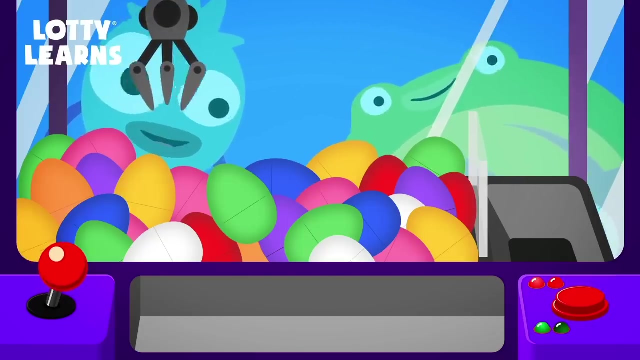 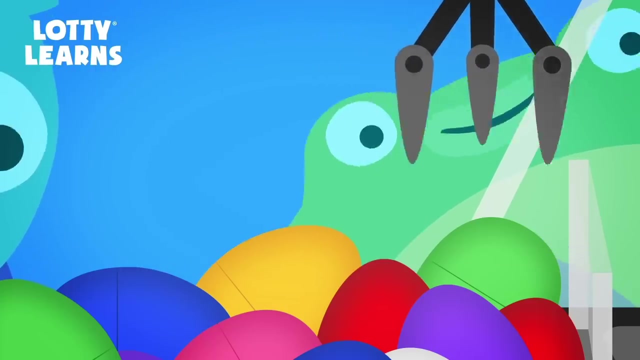 Oh, an orange egg. I wonder what's inside. O A Octopus. O is for octopus, Octopus. Let's play again. Once we get one, we can see what's inside. Oop, Try again. 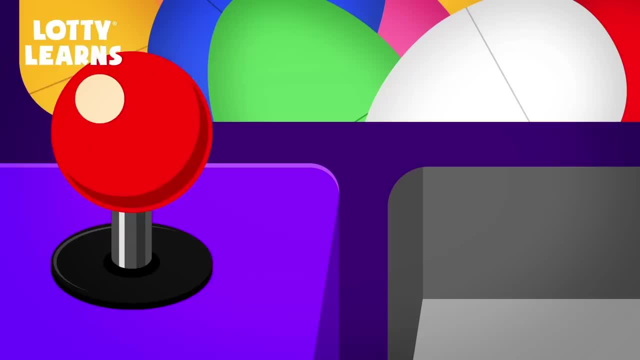 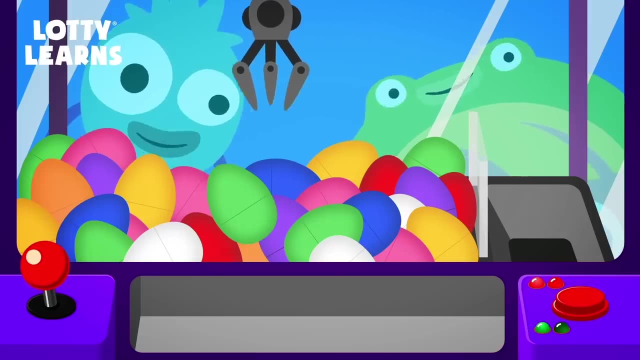 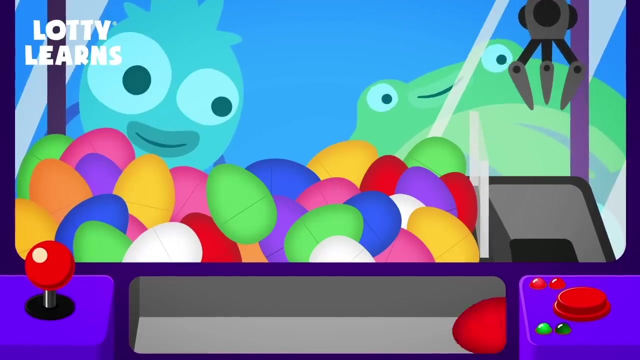 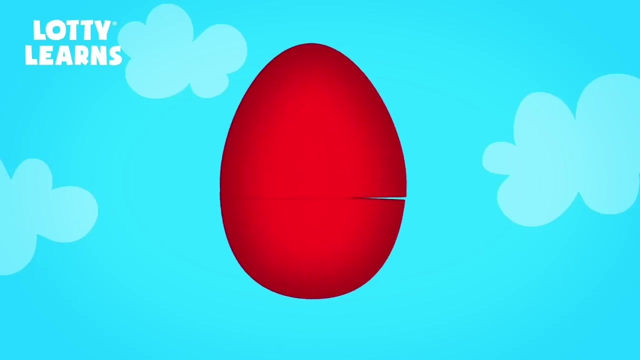 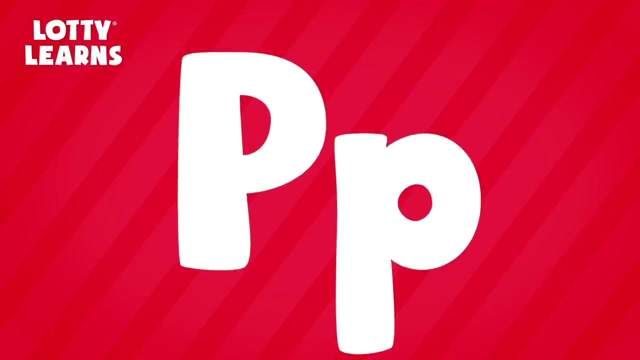 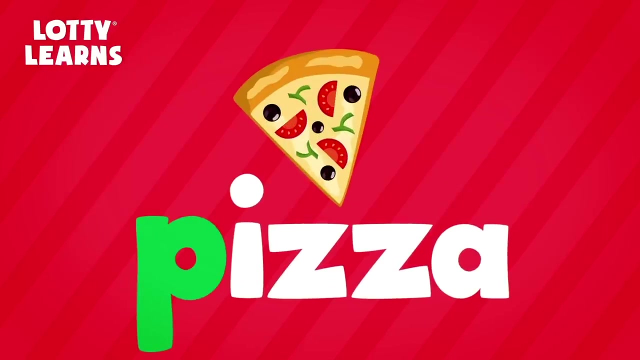 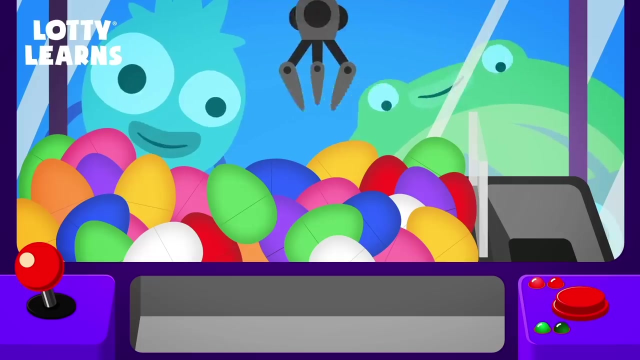 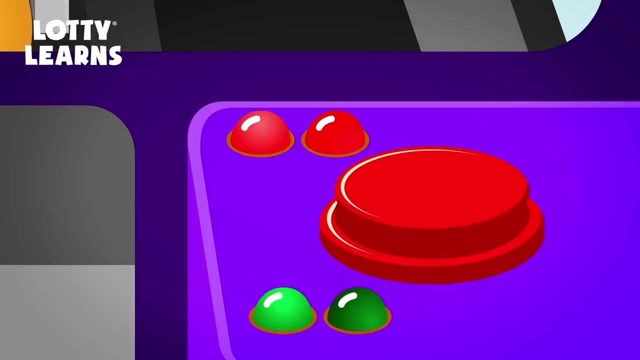 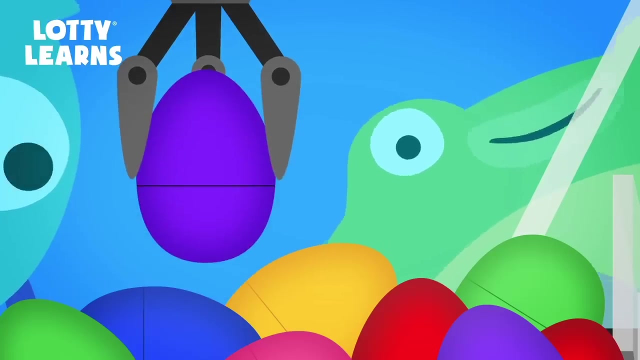 Let's play again. O A Octopus- O is for octopus, Octopus, P, P, P, P, P, P. Pizza- P is for Pizza. Let's play again. Can you guess what color the egg will be? Oh, a purple egg. 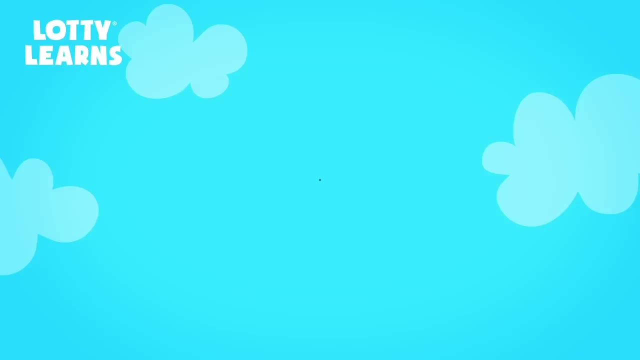 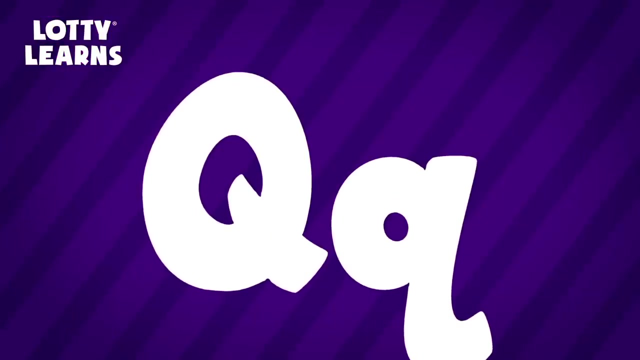 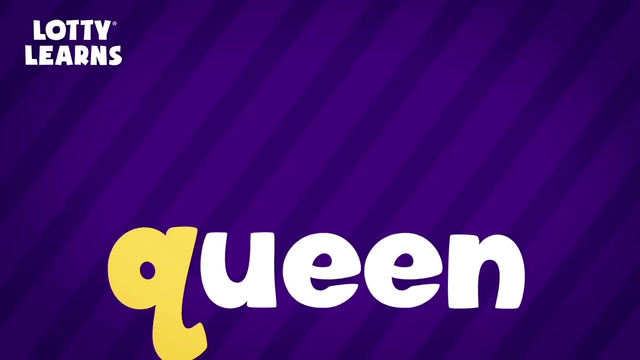 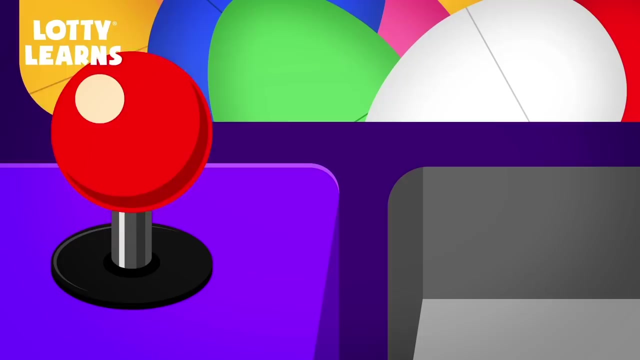 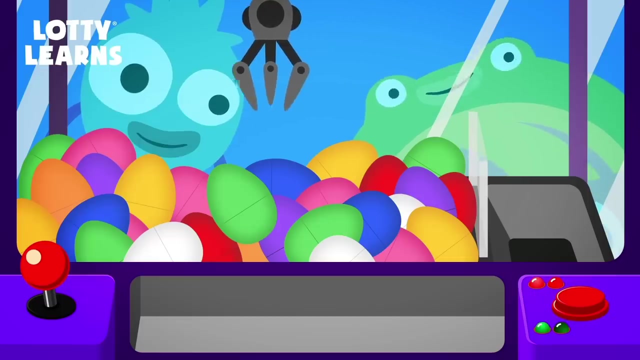 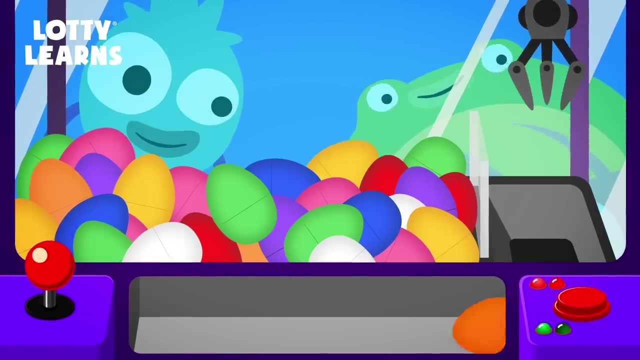 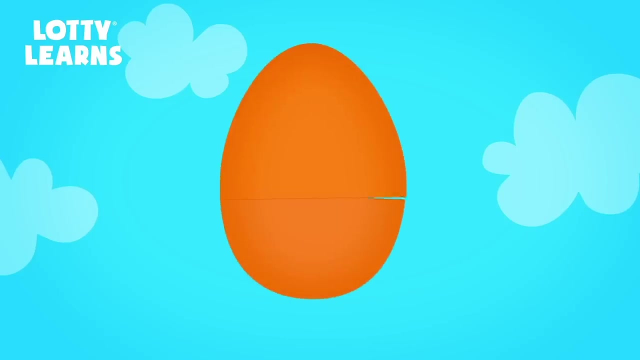 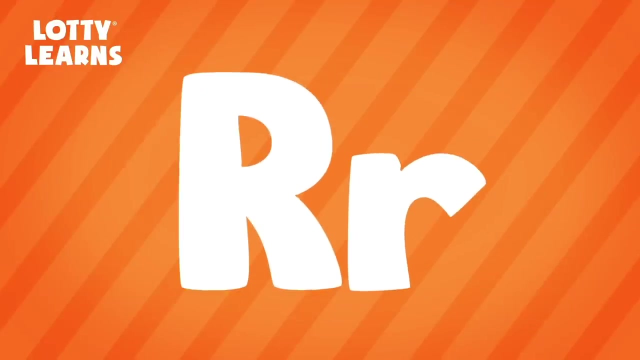 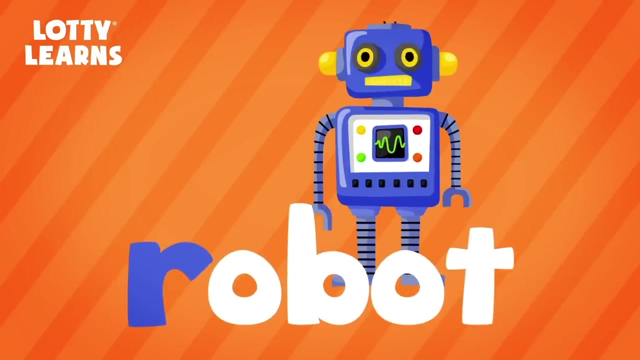 I wonder what's inside Q Q Queen- Q is for Queen. Let's play again. Once we get one, we can see what's inside Orange. I wonder what's inside. I wonder what's inside R R Robot- R is for Robot. This is fun, let's do it again. 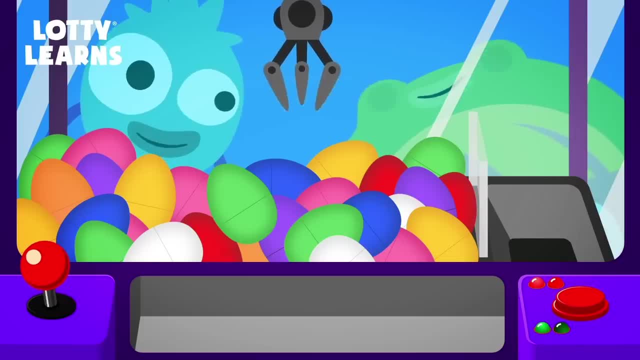 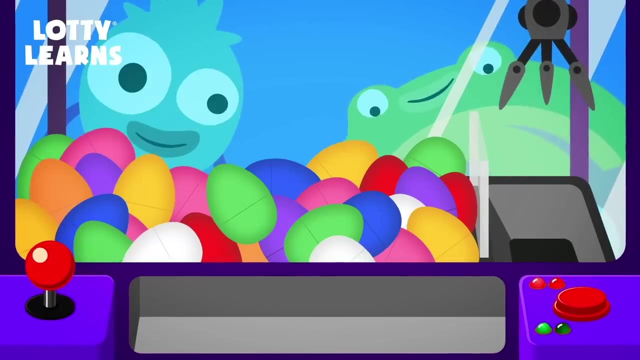 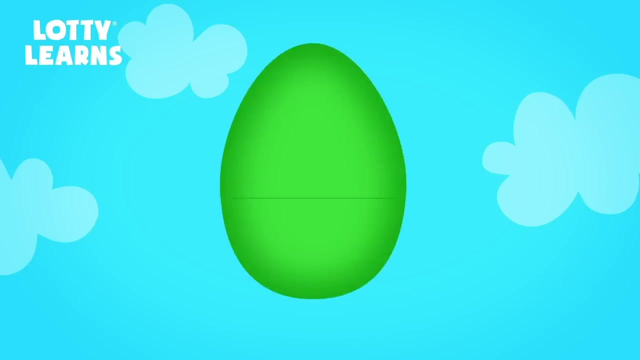 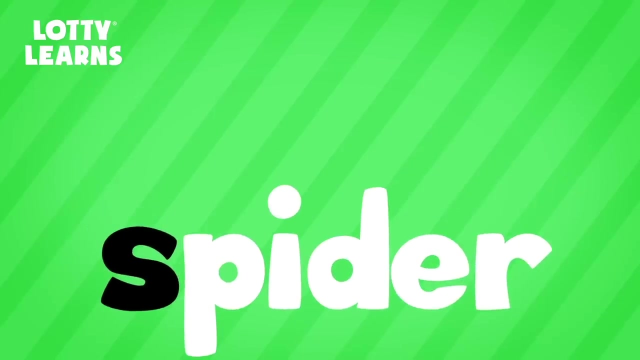 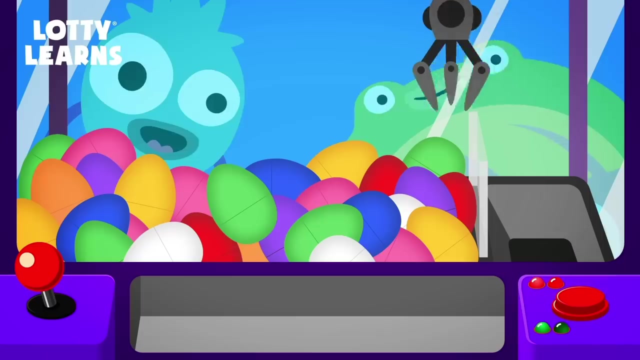 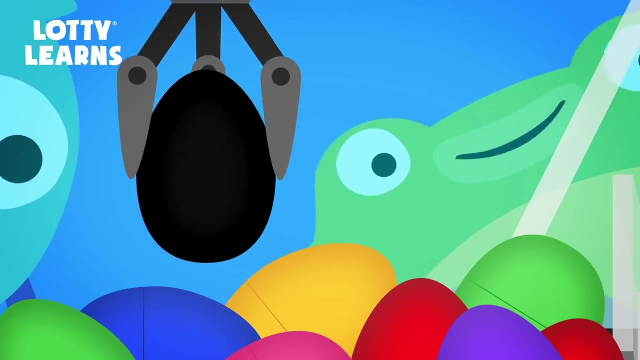 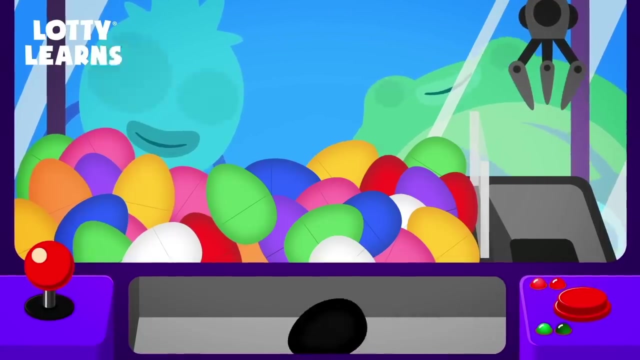 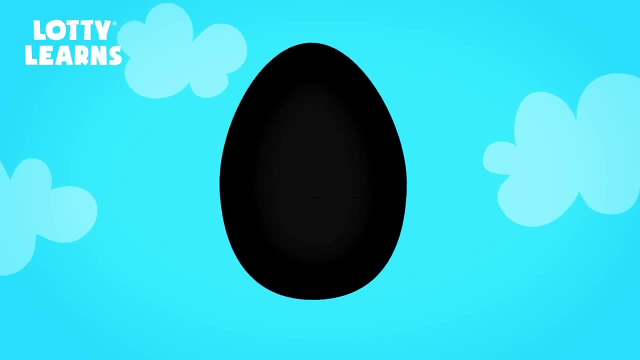 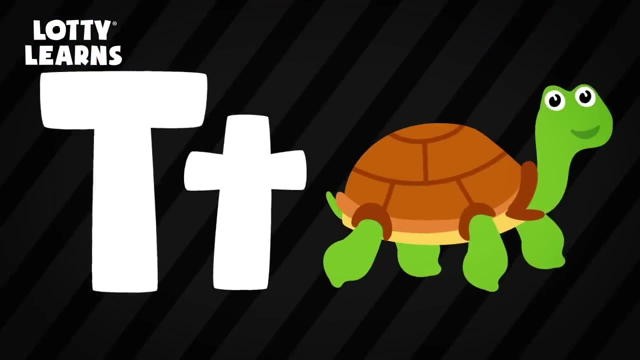 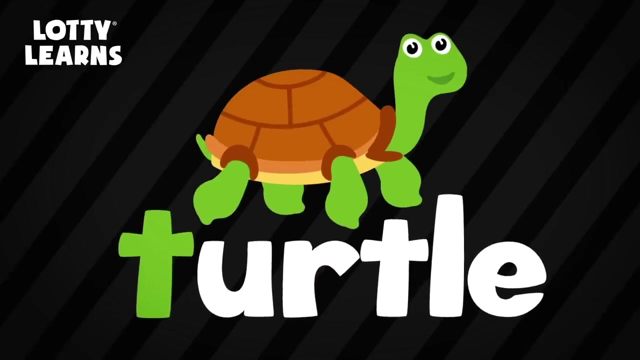 T, T, Turtle. T is for Turtle. Let's play again Black. I wonder what color we'll get this time. Black. I wonder what color we'll get this time. Turtle. I wonder what color we'll get this time. 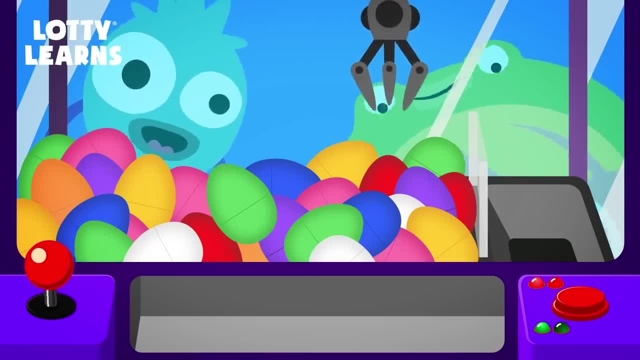 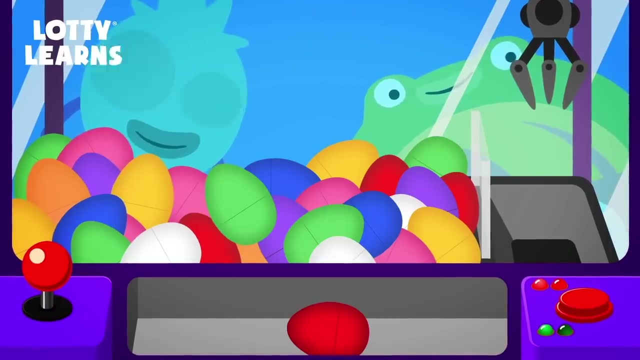 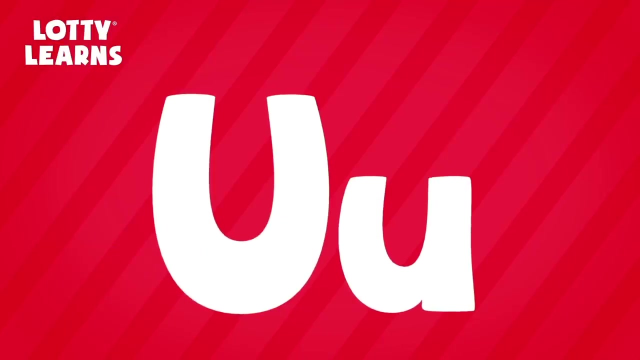 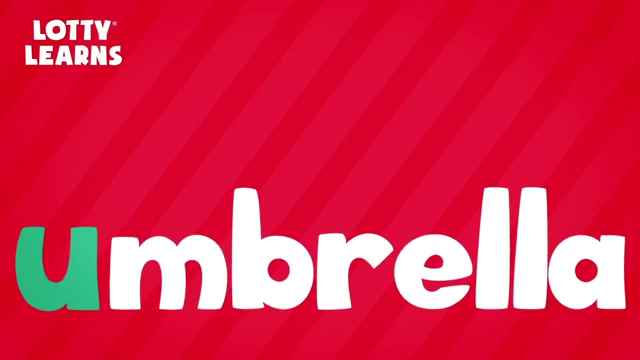 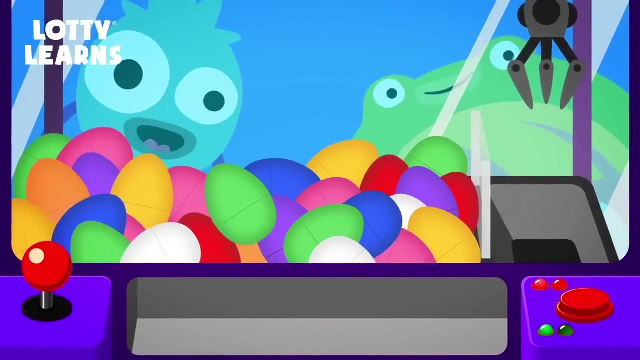 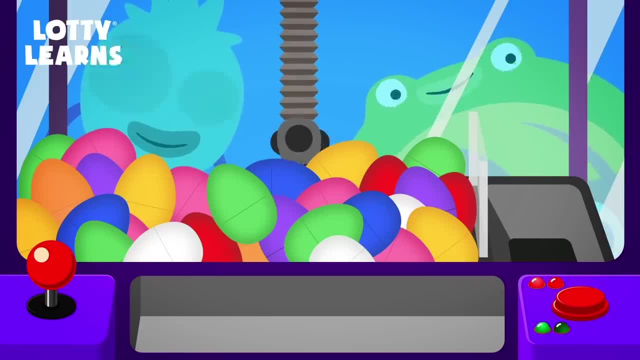 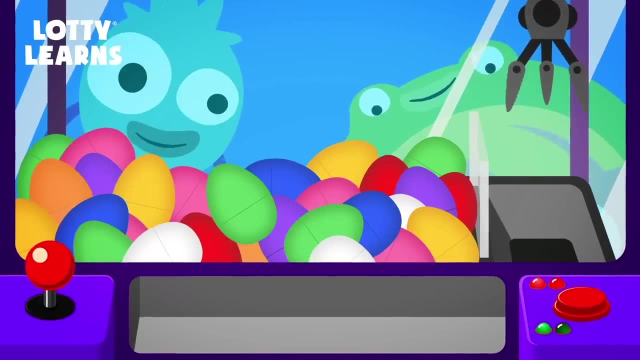 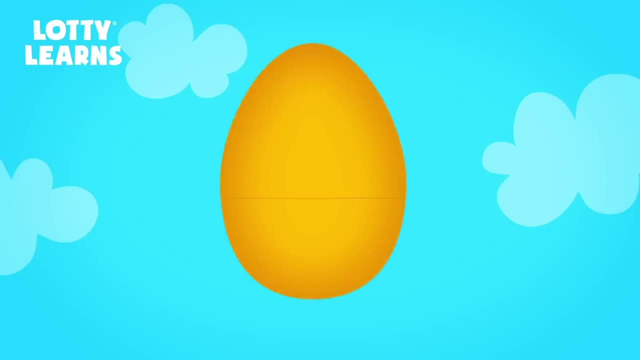 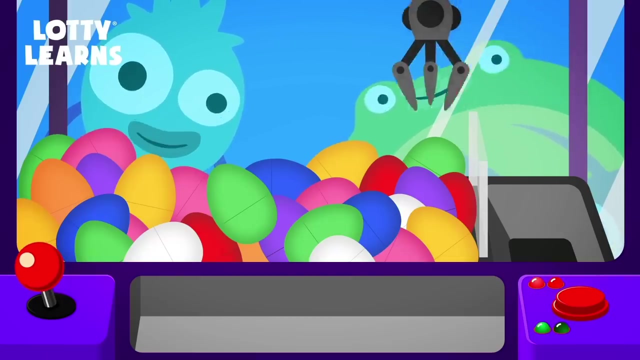 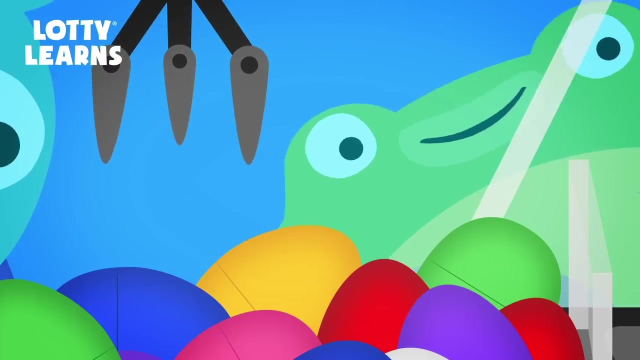 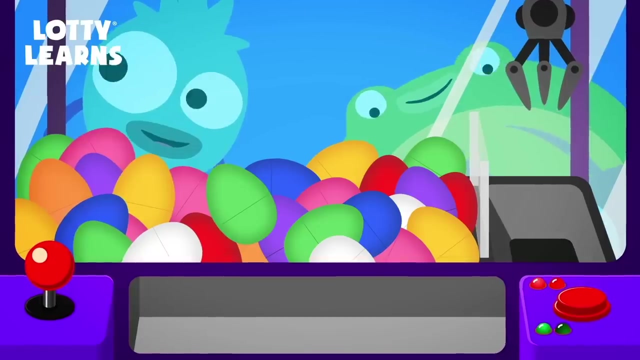 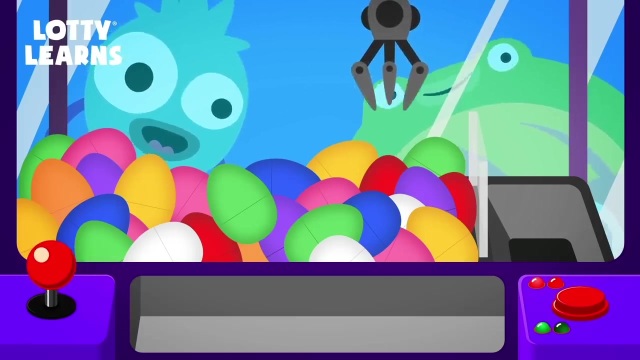 Yellow. I wonder what's inside. V V Vegetables. V is for vegetables. Let's play again. Once we get one, we can see what's inside. Try again. What color will we get this time? I wonder what color we'll get this time. 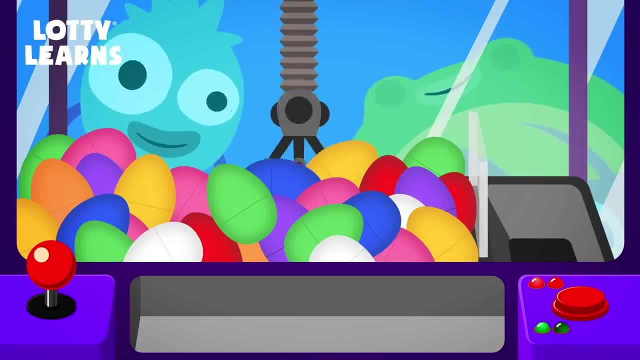 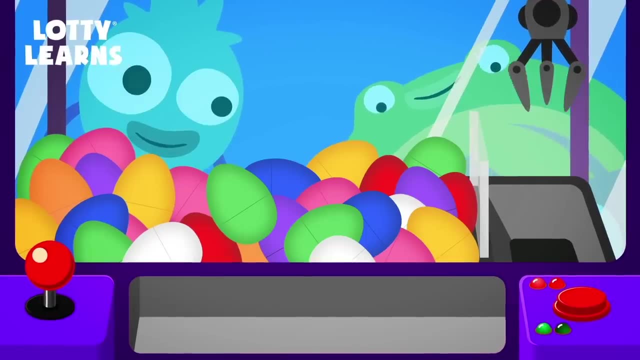 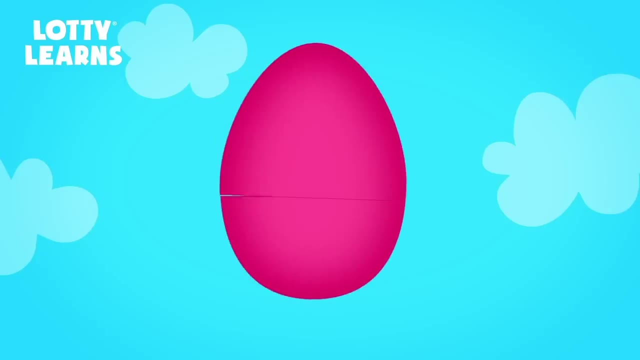 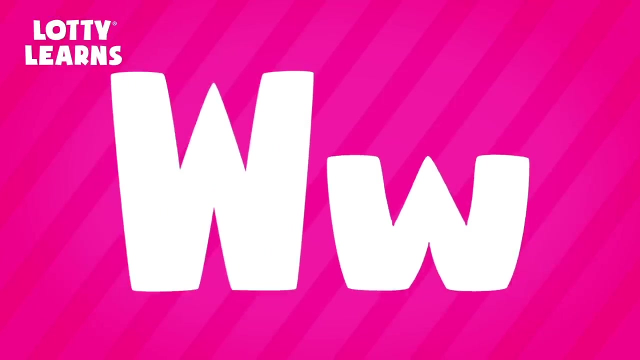 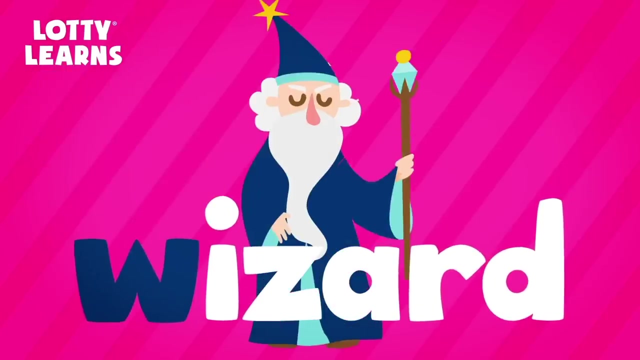 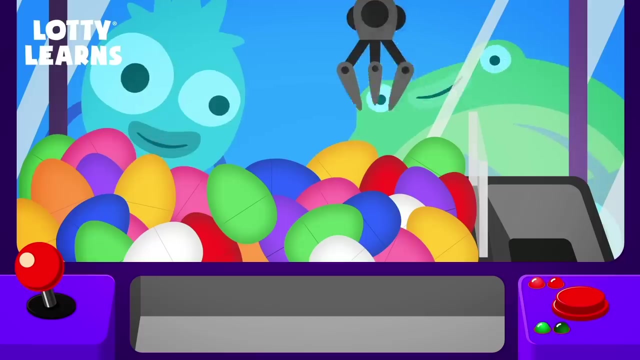 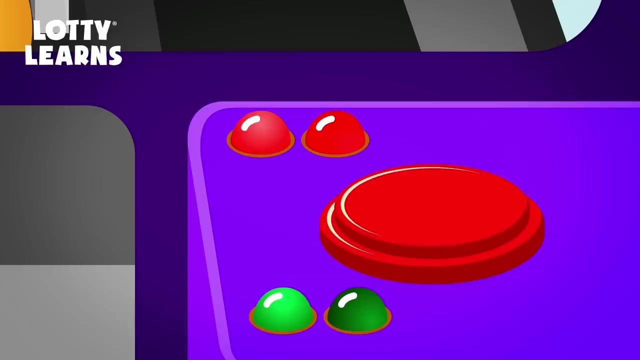 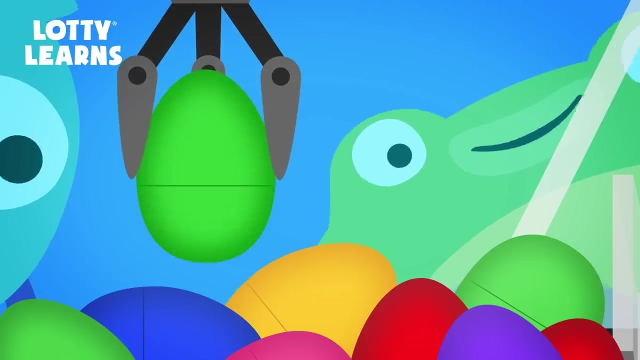 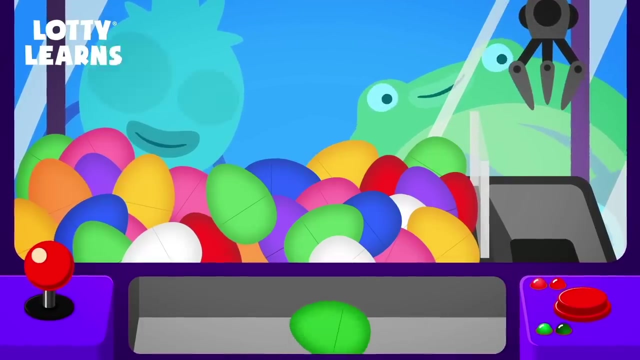 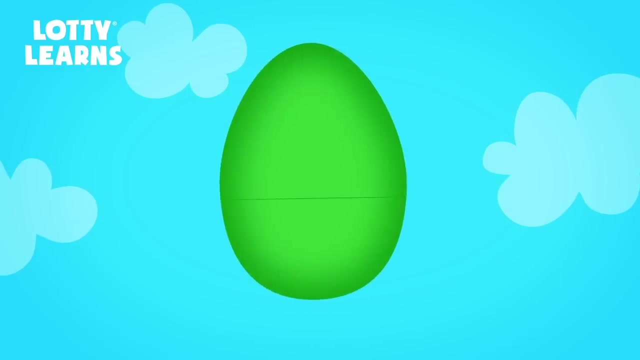 Y, Let's do it again. Is that roasted game milk? Oh, I wonder what's inside V, V, Vegetables. what's inside? Let's play again. Can you guess what color the egg will be Once we get one? we can see what's inside Green. I wonder what's inside. X, X. 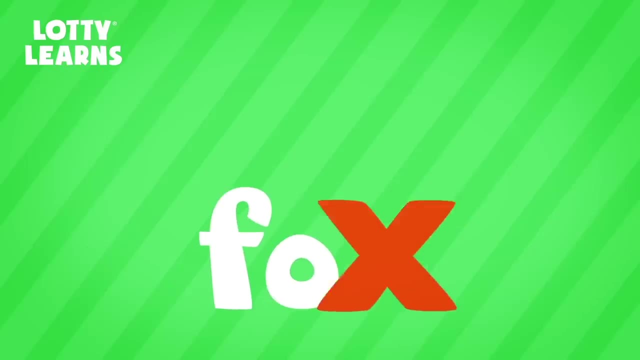 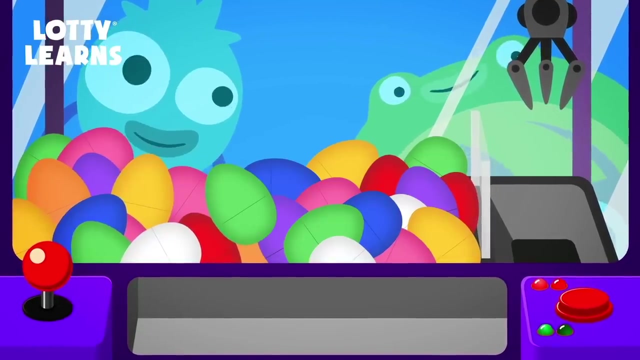 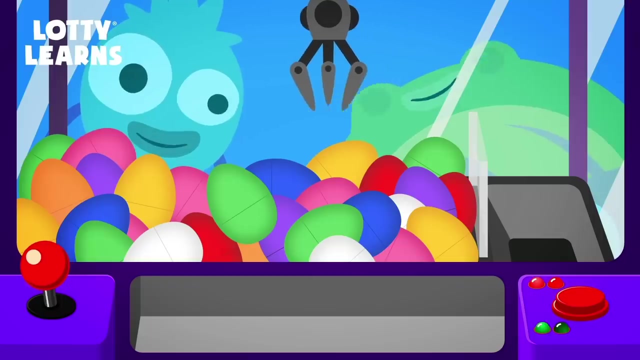 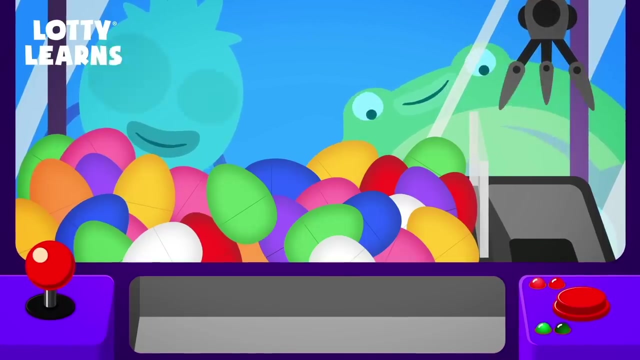 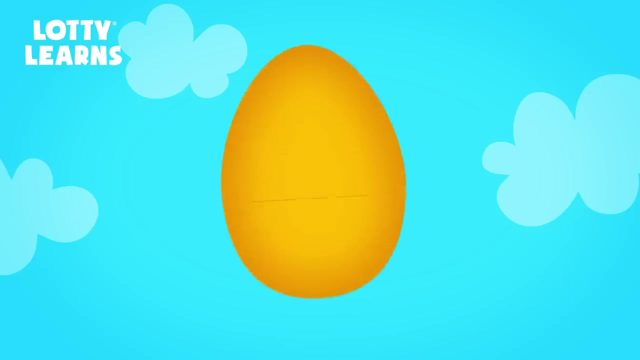 Fox X is for fox, Let's play again. I wonder what color we'll get this time. Ooh, a yellow egg. I wonder what's inside this egg. Y, Y, Yellow, Y is for yellow. Let's play again, Can you? 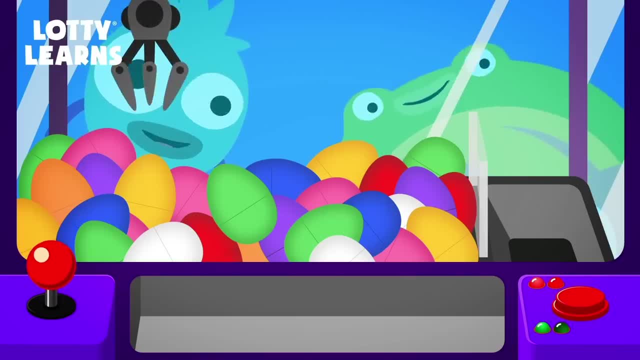 guess what color the mystery egg will be? X, X, Yellow, Y is for yellow. Let's play again. Can you guess what color the mystery egg will be? Once we get one, we can see what's inside. We grabbed a blue egg. I wonder what's inside. 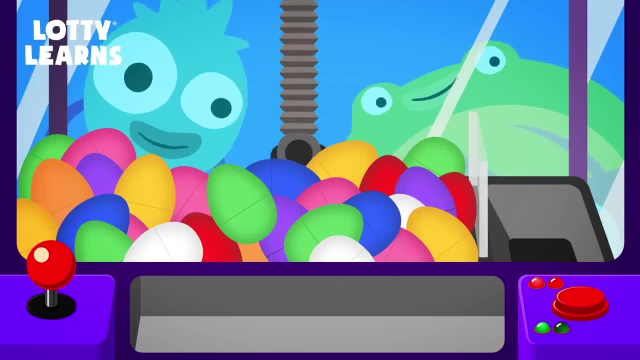 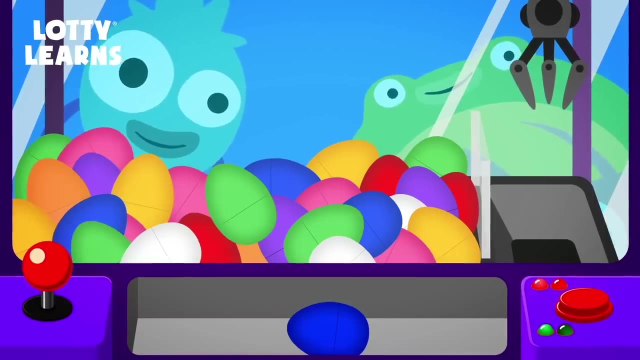 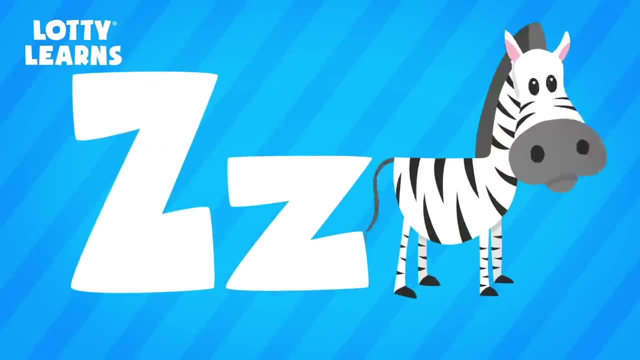 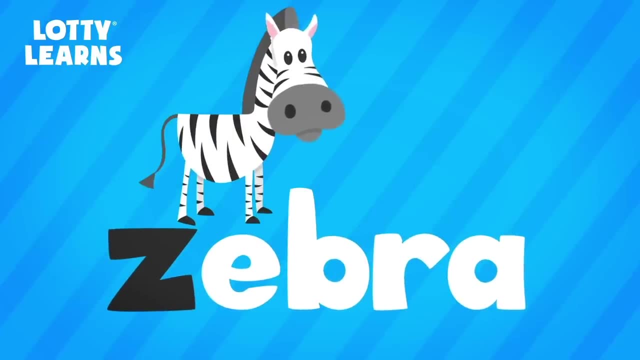 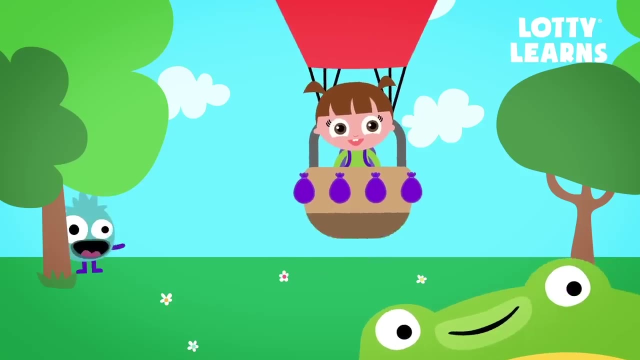 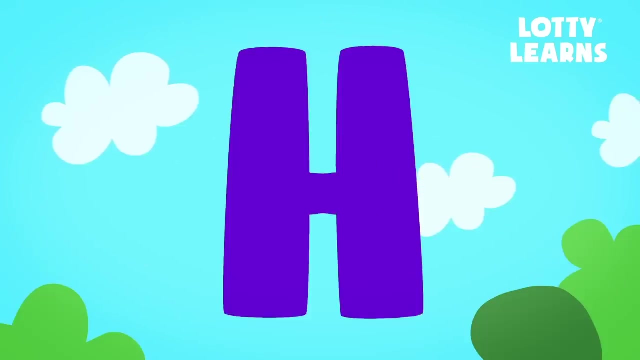 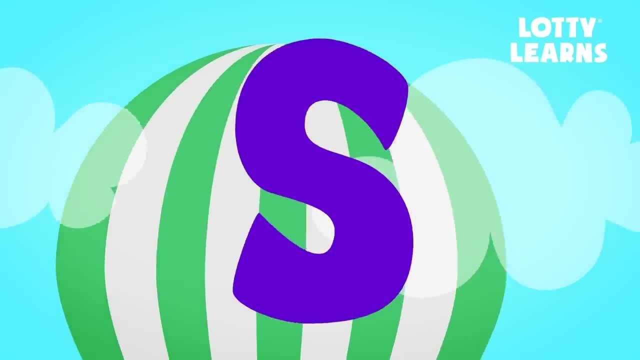 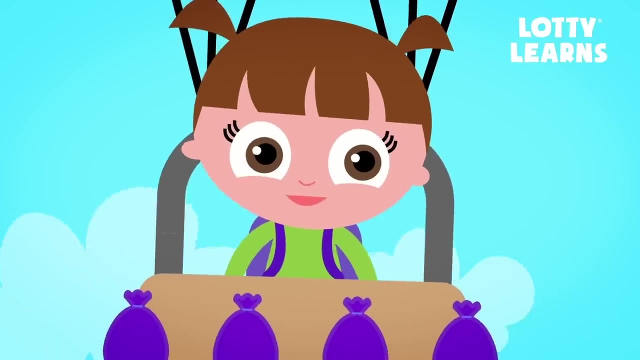 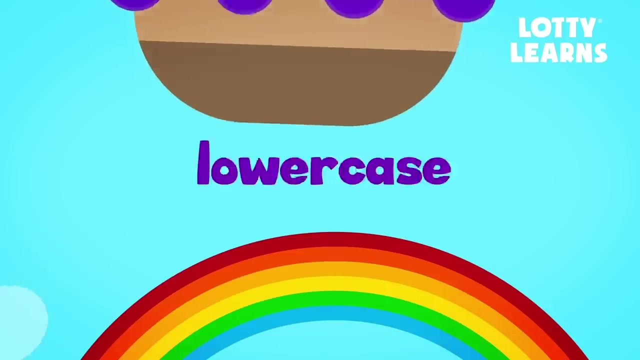 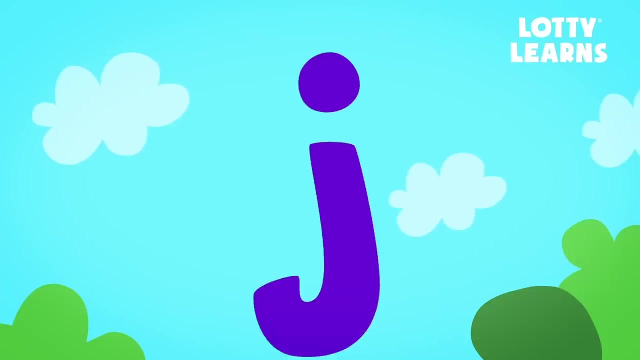 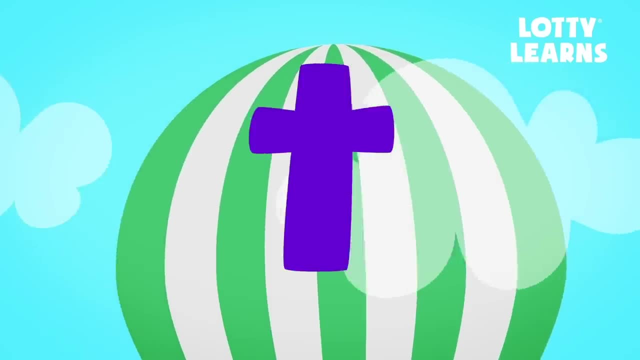 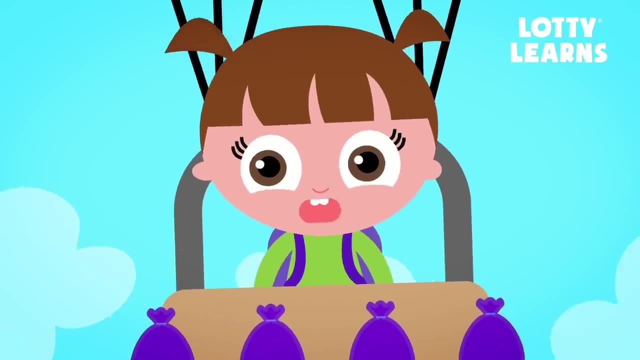 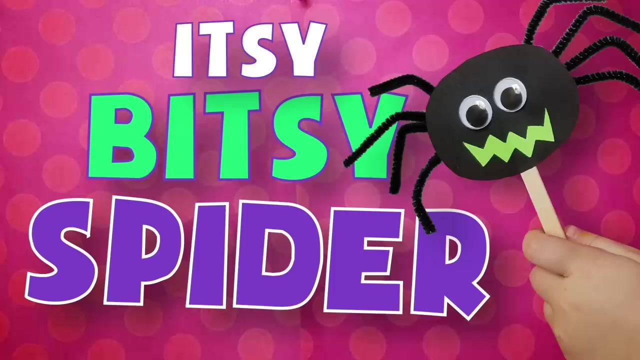 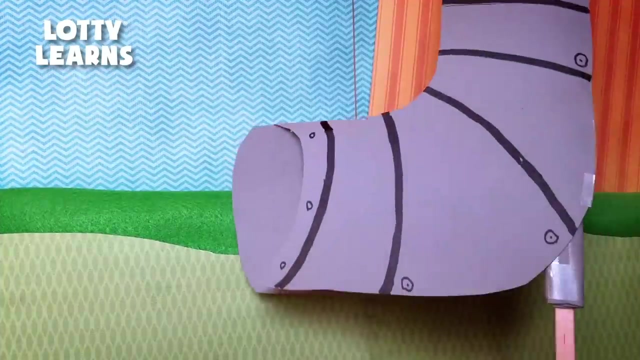 X, X, X, X, X, X, x, y and z. now i know my abc's. next time won't you sing with me the itsy bitsy spider? the itsy bitsy spider went up their water spout, down came the rain. 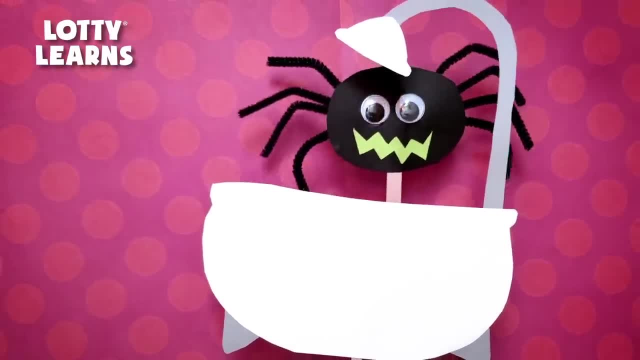 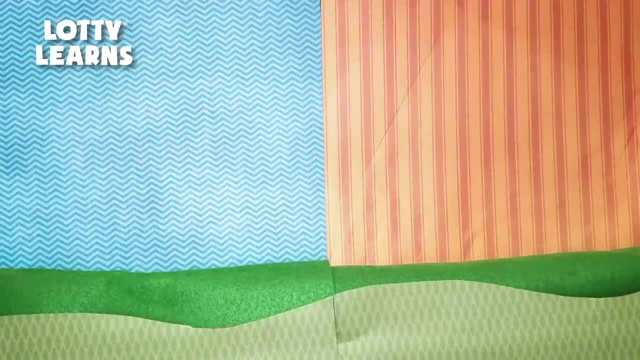 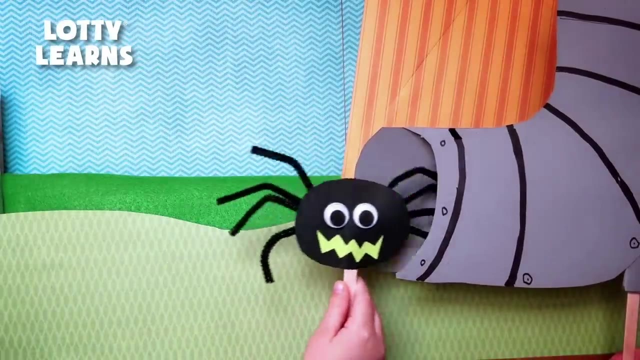 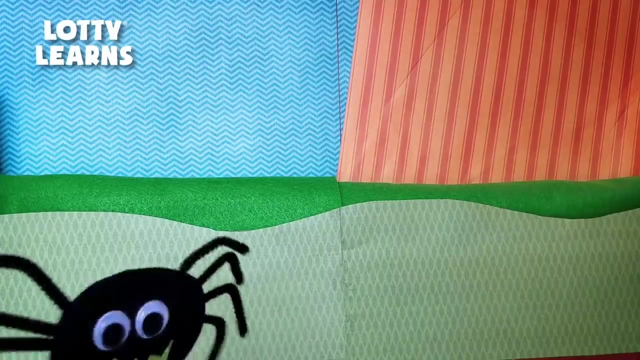 and gave the spider a bath. no, wash the spider out. oh, i, i always thought it was supposed to give him a bath. no, that's not what he does, okay. okay, let me start over again. the itsy bitsy spider went up the water spout. down came the rain and washed the spider out. up came the. what sun? the sun. 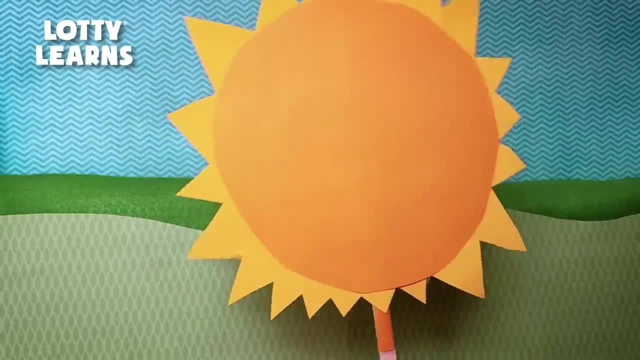 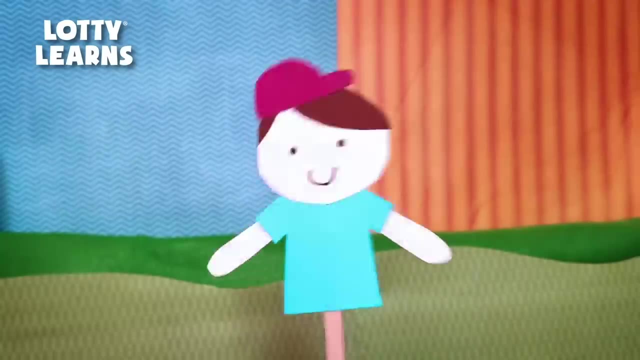 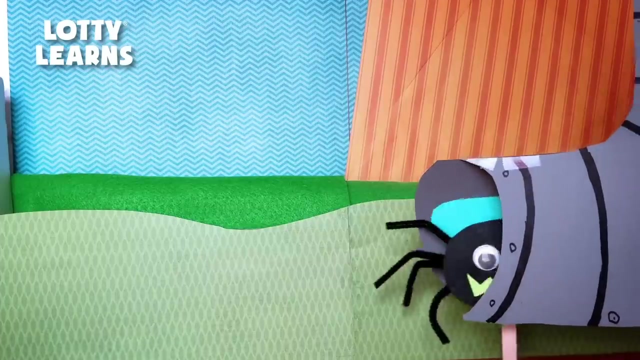 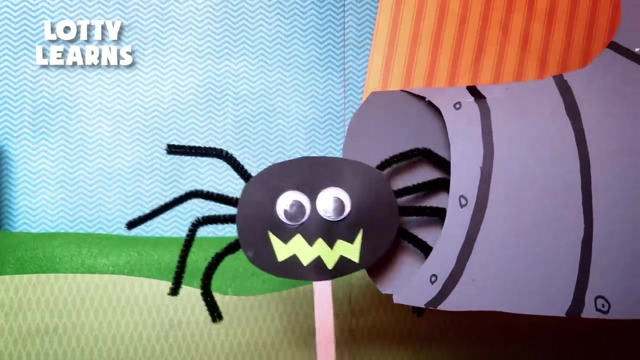 whose sun? no, the sun in the sky. oh, i thought somebody's kid came out. it was supposed to come out here. the itsy bitsy spider went up the water spout. down came the rain and washed the spider out. up came the sun and dried up all the rain and the itsy bitsy spider went up the spout some more. 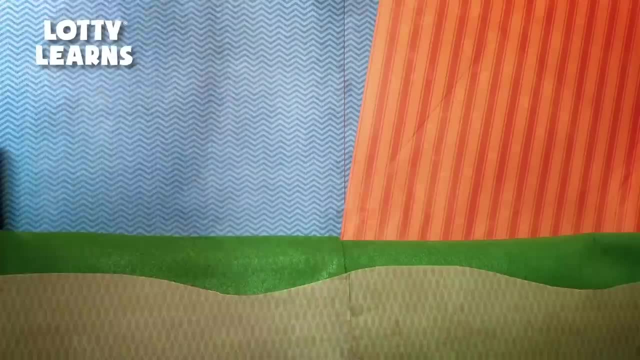 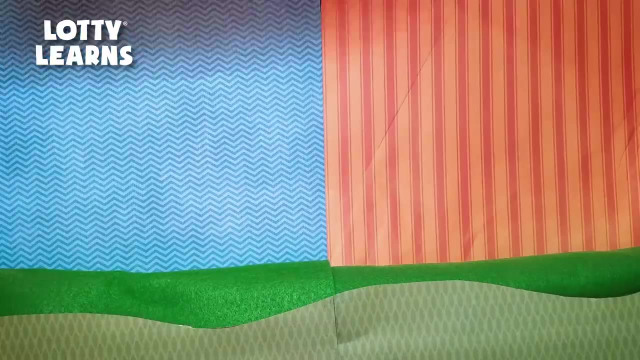 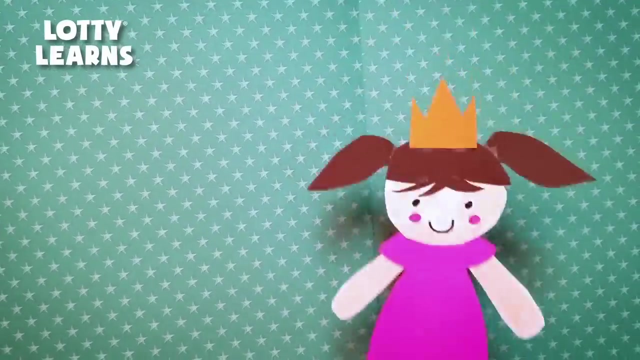 no again. oh my god, oh my goodness, i'm messing this song all up. okay, give me a second here. the itsy bitsy spider went up the water spout. you have to impress the princess, you have to impress. there's not a princess in this song. yeah, look, do we need to make a princess? 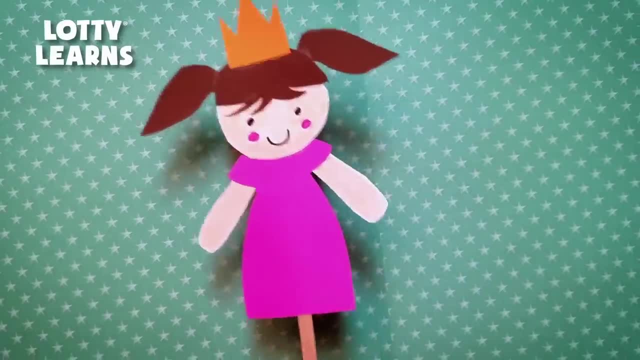 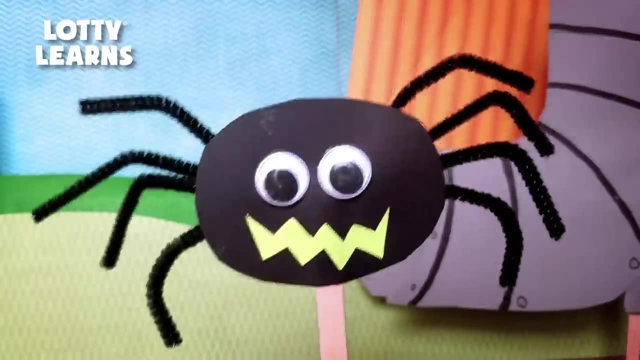 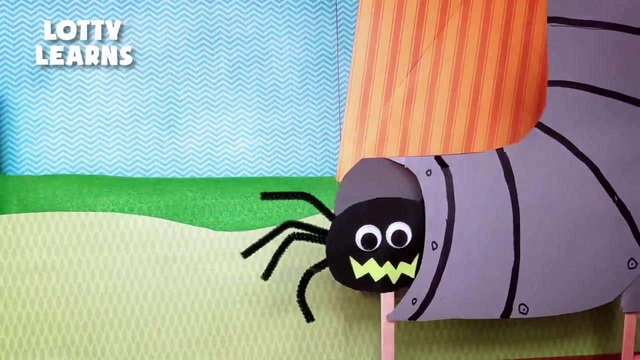 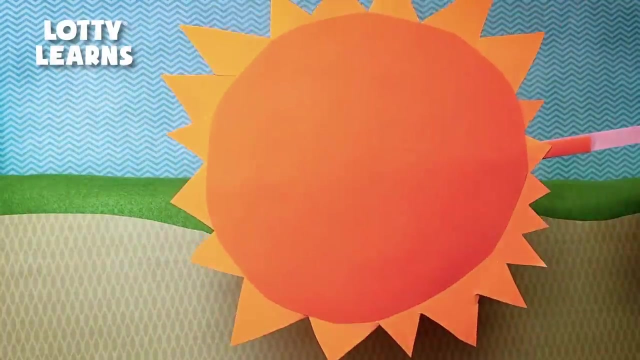 character for this. you want to sing it with me? don't clap. okay, ready, we can sing together. the itsy bitsy spider went up the water spout. down came the rain and washed the spider out. up came the sun and dried up all the rain and the itsy bitsy spider went up the spout again. 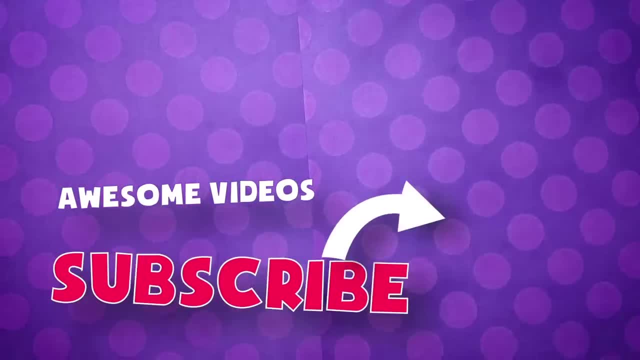 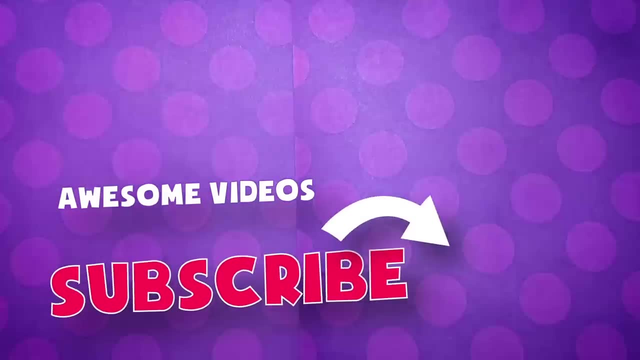 bravo, yay, click another one of our awesome videos and please subscribe and hit the notification bell so you don't miss out on any of our new videos, and we'll see you in the next one. bye.